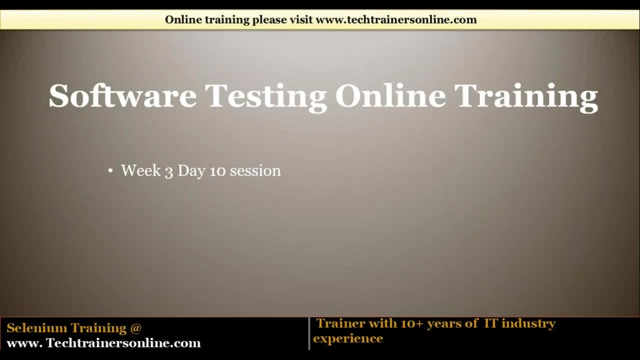 This conference will now be recorded. Hey everyone, welcome to Software Testing: Online Training- Week 3, Day 10 session from TechRenardsOnlinecom. In today's session, we will talk about test plan and as well as the defect management, and also try to understand what is the difference between defect management. 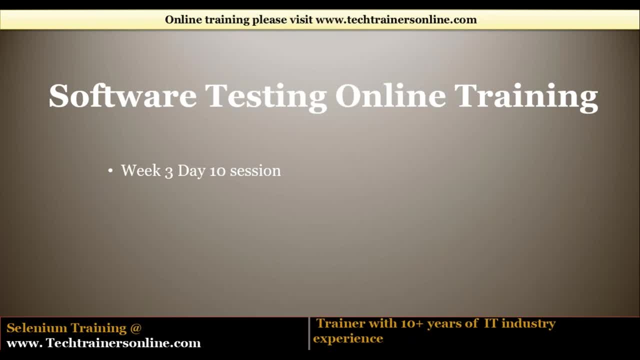 and the change request management. So let's start with the test plan. So test plan is a document which is prepared by a test lead or a test manager. So most of the time it is going to be prepared by the test manager and it all talks about. you know what are the activities? 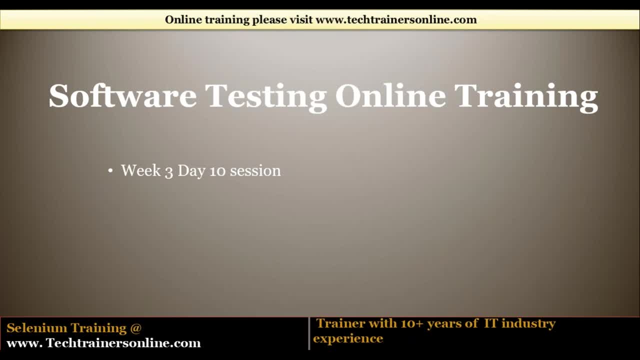 that we are trying to do as part of our testing. Like you know what types of testing we are trying to do, what are the different tools we are using for the test management or defect management, what are the automation tools we are using and all what are the resource management? 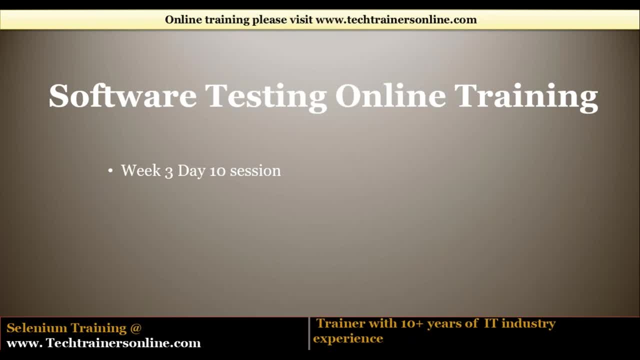 what is the time? You know deliverables of the testing activities. So what are the deliverables, what we are going to deliver? All this information is going to be detailedly written in the test plan. So once the test plan is prepared by the test lead and or the 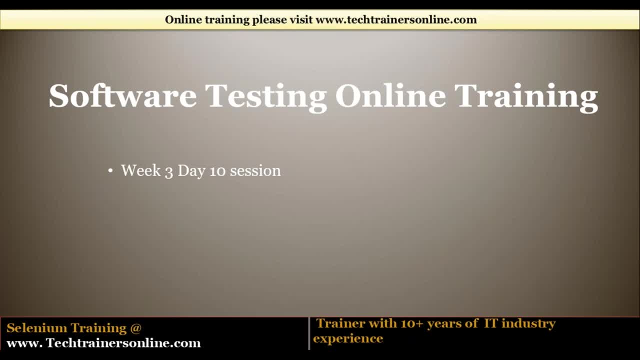 test manager. it's going to be sending to the client for the review and the client is going to review your test plan and then they can provide their comments Based on the comments. again, you guys have to- when I say you guys, the test manager has to work it out to know the comments. 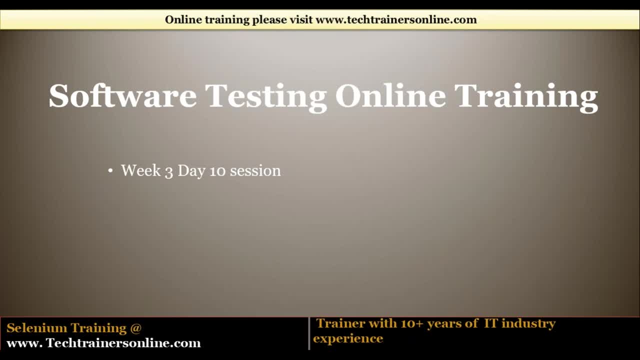 given by the client. So, in order to understand, this plan is a document which consists of all the information related to testing. all the information related to testing like: what are we, what are we going to test? What is in scope for us? What is out of scope for us? You know how? about the 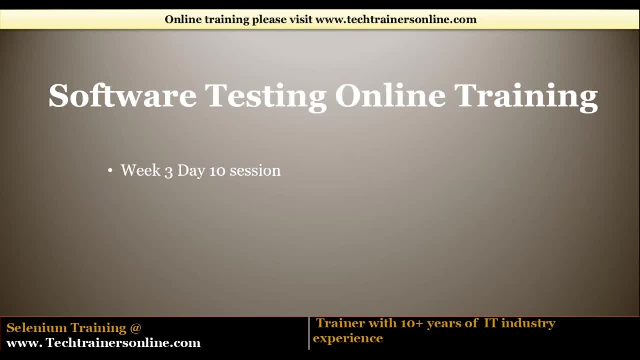 resource management. You know when to stop testing. entry criteria, exit criteria. all this information will be detailedly written in your test plan document. So when we talk about in scope, like, say that you guys are working for a bank called Citibank, is the client and the bank has. 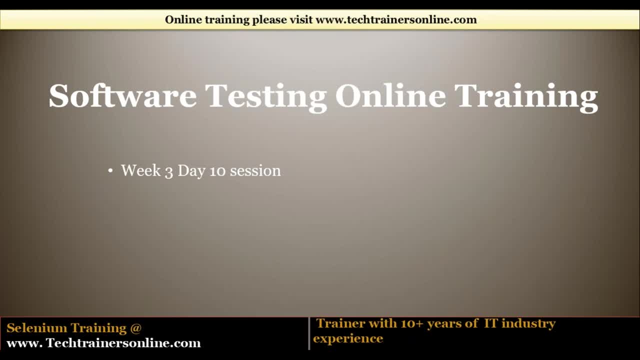 given to test this application and bank has the two different systems like debit card management and credit card management. Let's say that you are working for a company called Accenture and your client is the Citibank. I'm just giving an example. So Citibank has the two things. One is the Debit card management system and as well. 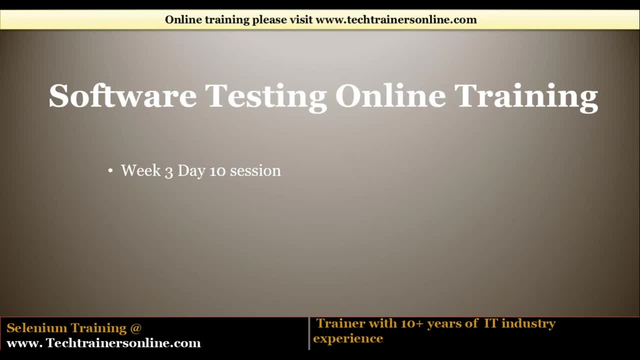 as the credit card management system. Let's assume that the Citibank has given the debit card management system for testing to the company called Accenture and debit card system. credit card system is given to the. you know the credit card system has unaccessibleWAN system. 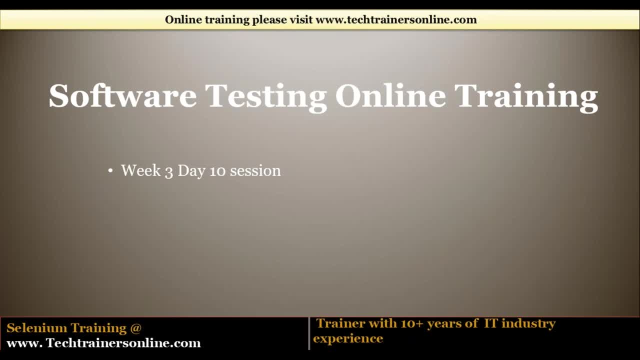 system is given to the another company called, let's say, ibm. so the company your client has given the system to the testing for different companies- one for accenture, one for ibm- right? so what are you guys going to do as part of the test plan? so what is in scope for me? 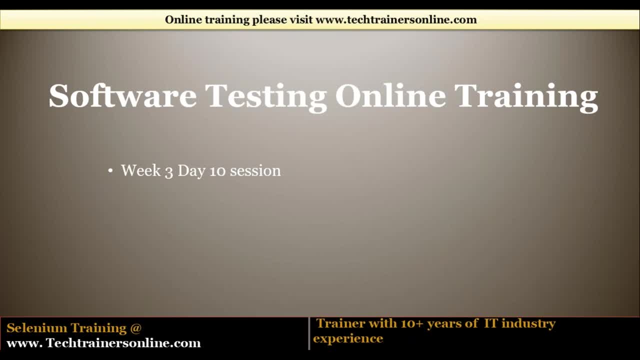 do you guys think that credit card management is in scope for me? it's not in scope for me, right? because it's not given to accenture, assuming that i'm working in accenture and, uh, i'm writing a test plan for whatever the client called citibank i'm working for. so when i say in scope, 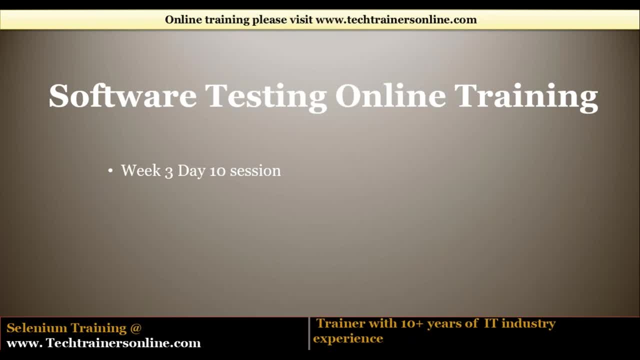 i'm clearly writing that debit card management testing will be in scope for testing. are you guys getting what i'm saying? what i'm saying is the debit card management testing will be in scope of testing. i'm not talking anything relevant to the credit card management system, because it's. 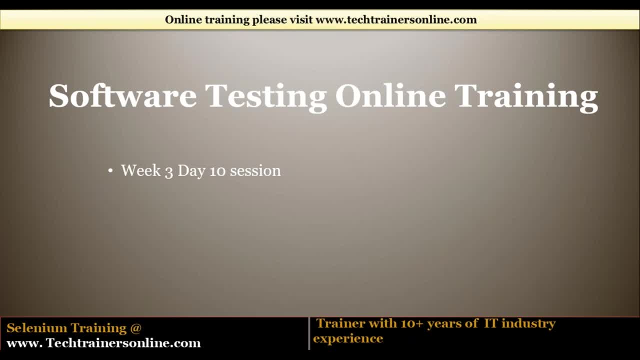 not in scope for me, it's completely given to me, given to another company, so where i'm not responsible for that particular module of the citibank. so, when it comes to the browsers and operating systems, we talked about the compatibility testing, right, so we learned. we learned what is compatibility testing and 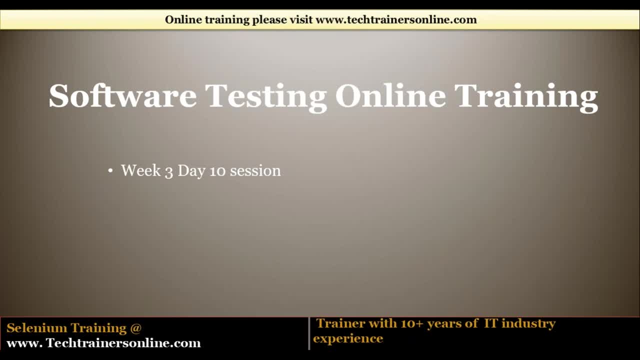 you know what we need to consider in the compatibility testing. so in the test plan we are all going, we are also going to document what are the browsers that we are going to use and what are the operating systems that we are going to use. so that's perfectly according to the protocol. so so you know what our testing kind of. 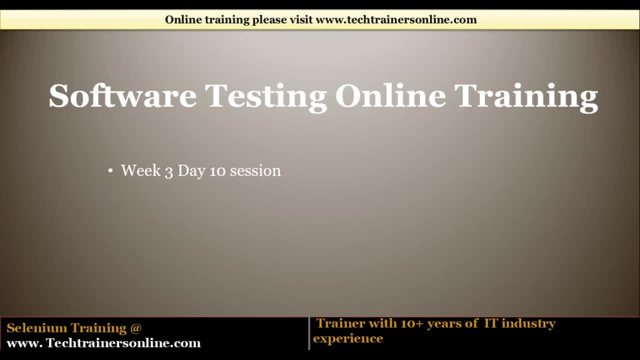 seems like the testing will be in scope of our testing, so the testing will be performed in below browsers: ie version with ie 6 and above and google chrome version with 42 and above. so i reach out to the client and asking that which version of the browser are? what are the different? 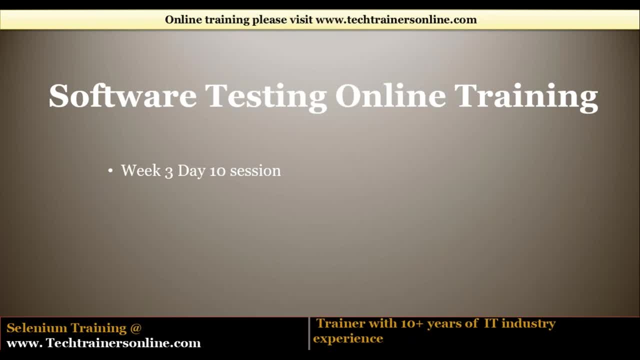 types of browsers that you are uh expecting us to do the testing, and we can go ahead and do that. that's what we are trying to trying to document it in our test plan. so what are the operating systems we are trying to consider? testing will be performed in below operating systems, like one is windows, with the version. 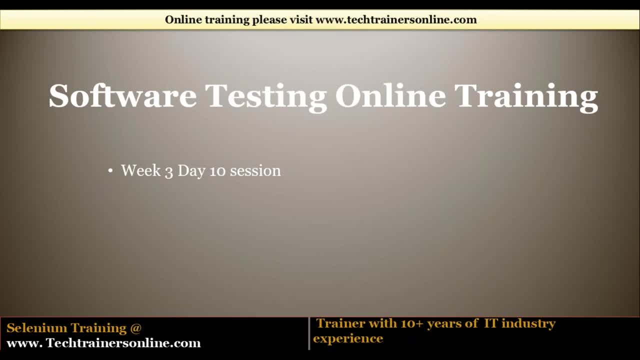 2008 and above. android version 2.0 and above ios 3.0 and double. i'm just given some version number for the sake of example. it can be any number. so these are in scope for us. debit card management system is in scope. iea 6 and above version is in scope for testing. chrome with version 42 and. 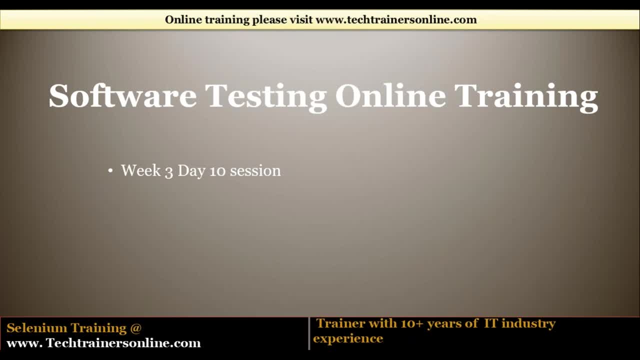 evo is in scope for us, and operating systems like windows, android and ios are in scope for us. so what is out of scope? so credit card management is out of scope for us because we are not working on it. the client has given it to another company, right, so browsers and operating systems other. 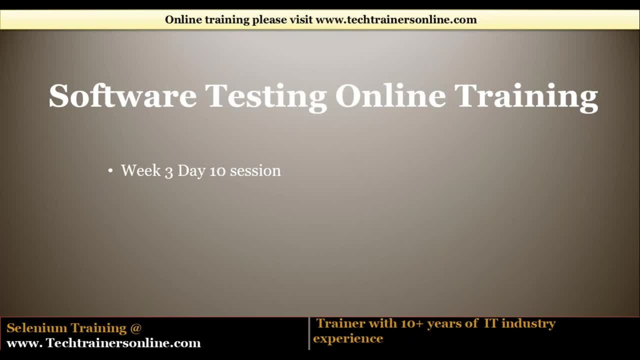 than evo is not in scope for testing. i listed out what is in scope for me. anything that comes outside of the outside of uh versions or browsers, whatever is mentioned, is not in scope for me, which is called as out of scope for me. so we clearly list out what is in scope for testing and what is not in scope for for testing. also, we need 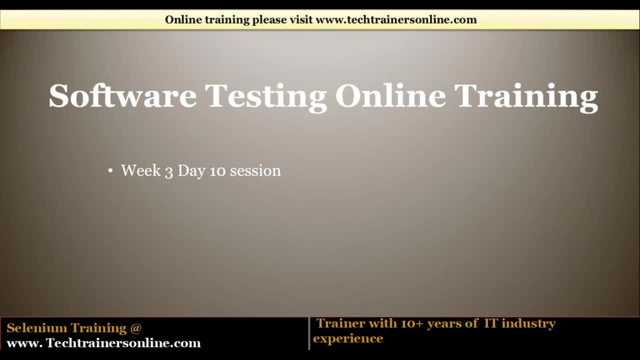 to document it in the test plan so that tomorrow if some customer is using very old version of the browser, let's say i or iu5, and if it is application is not launching or having some issues in the older version of the browser. if they call to the customer care, customer care executive will always tell that which version. 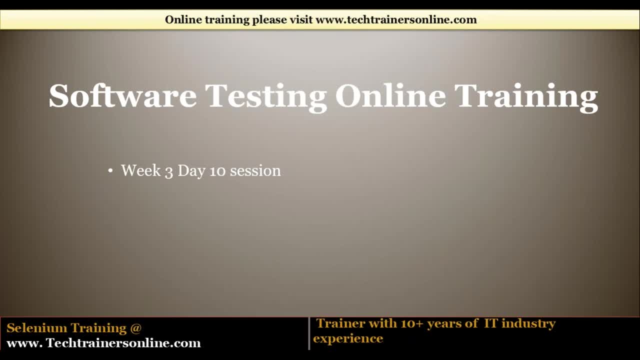 of the browser you're using. if the customer says i'm using iu4 or iu5, the customer care executor straight away can say that our application is not compatible in the old version of the browsers, so please upgrade your. please upgrade your browser so that our application is compatible. 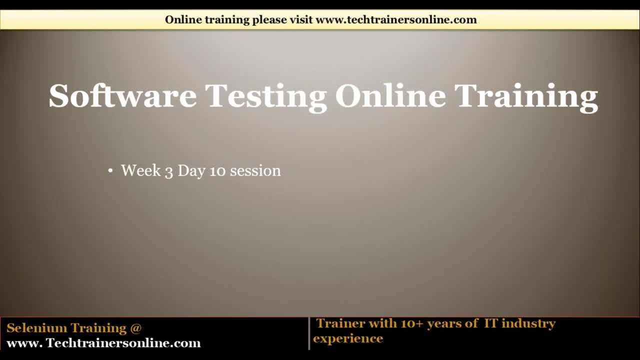 with your system. that's what exactly we are going to- uh, you know, discuss, because tomorrow i don't want client to come back and say that you know it's not working in ie4. so i can clearly show this document indicating this is what we have agreed and this is the version and the types. 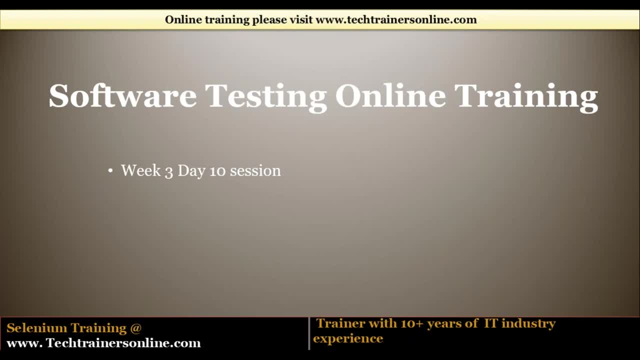 of browsers, what we have agreed, so it is not in scope for us straight away. you can reject any data effect that is coming relevant to compatibility issues. okay, let's move on for the test environment. we discussed about the test different environments yesterday. right, so like we have. like we have test environment, uat environment, reproduction. 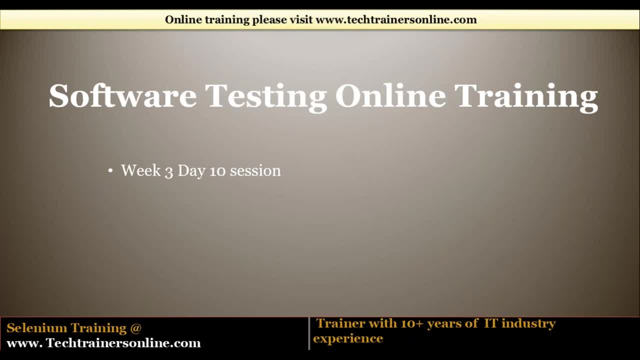 environment and production environment. so this test plan is always prepared by the test manager, right? so this is applicable for the system test, system testing. so we also call this document as system test planning. so when i say test environment, test environment should be set up and access should be given to the testing team as well to development team. so what i'm trying 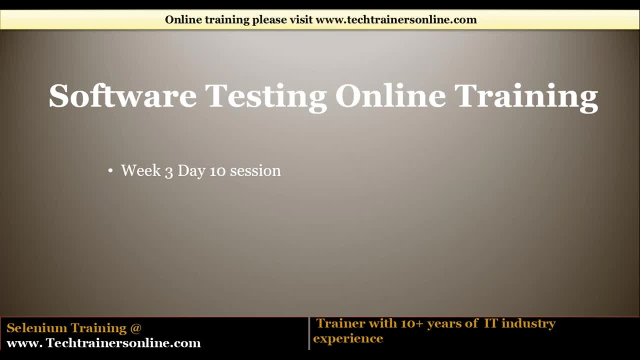 to say is if my testing team has to start the doing testing, i'm saying that the test environment setup is ready and all the testers has the access to the test environment to use it right. so generally, the testing team will be testing team will be given with the testing team will be given with the. 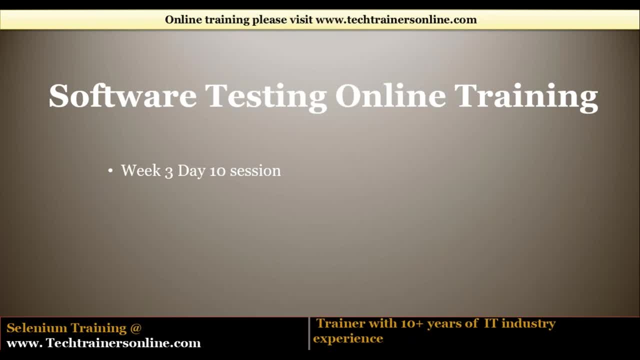 login credentials to the test environment and where tester can go ahead and log with the test user ids that are created. i think we already discussed what is test environment in previous session. okay, and then we are also mentioning what are the different types of testing that we are. 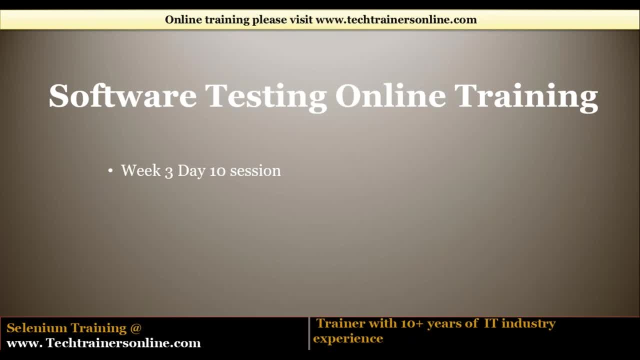 trying to do for this particular application. right, so we are what we are trying to do. we are trying to do the regression process testing. so i'm also trying to elaborate more. what do you mean by regression testing? so in this testing, we consider end-to-end flow as part of regression. we plan to do this testing through. 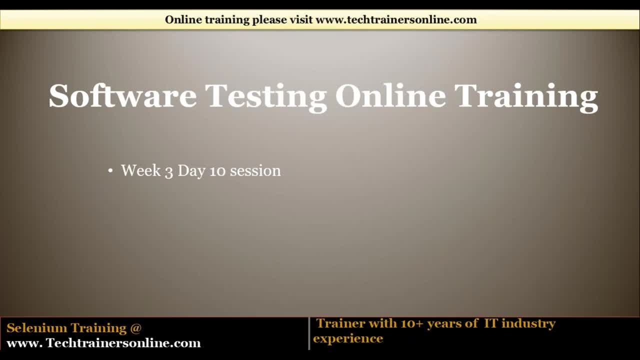 automation only. so, as mentioned, regression testing, we are trying to cover end-to-end flow and through with the automation right. so that's what we are trying to do. that's what we are trying to do as part of the regression. i don't want client to come back and say that 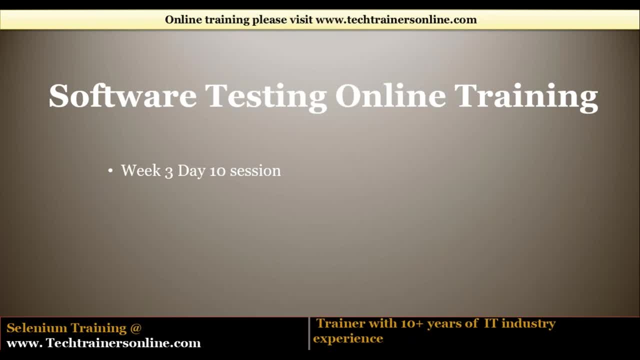 uh, you know what is not covered in regression. i'm clearly defining: i'm going to do the regression testing and it is going to be end-to-end flow. that too, with the automation. only are you guys getting what i'm saying? end-to-end flow means the core of the system. 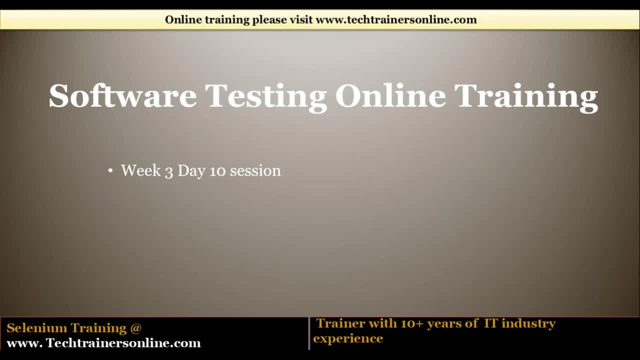 like if you take in a banking example, it it basically starts with login creation, register an account, login into the account right and then do all the transactions right. you create an account, log into the account, reset the password you know, use the forgot password and see it is working fine and, logging into it, add the beneficiary, transfer the. 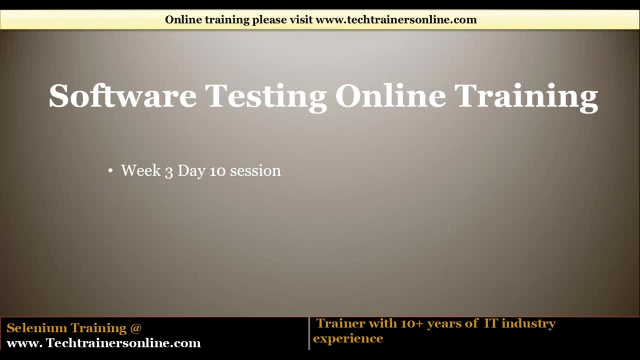 funds. we delete the beneficiary, change the pin number, generate instant atm pin number for your debit card, you know, and make the credit card payments or debit card payments. so this is what exactly called end-to-end flow. so you're trying to touch base with every functionality of the system. 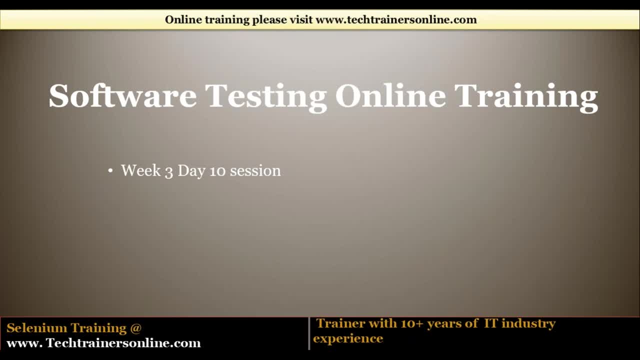 to make sure that core of the system is working fine. that's what i'm i mean to say. end-to-end flow is considered as part of the regression, and that too, we are going to do it with the automation testing only. any questions on this types of testing regression. 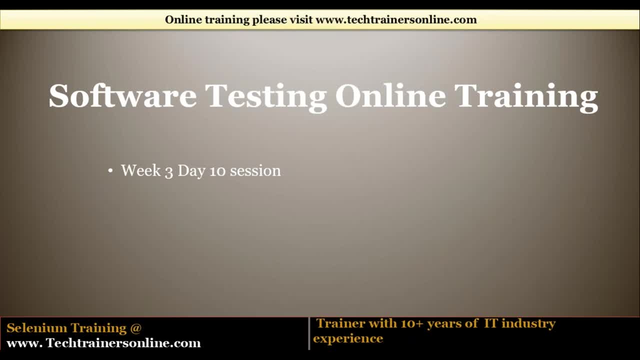 i'm also mentioning that i'm going to do the sanity testing. we also perform the sanity testing, functional testing, installation and uninstallation testing, if applicable. now let's say that you guys are working for a product-based company and let's say your client is microsoft and you guys are. let's say that you guys are working for. 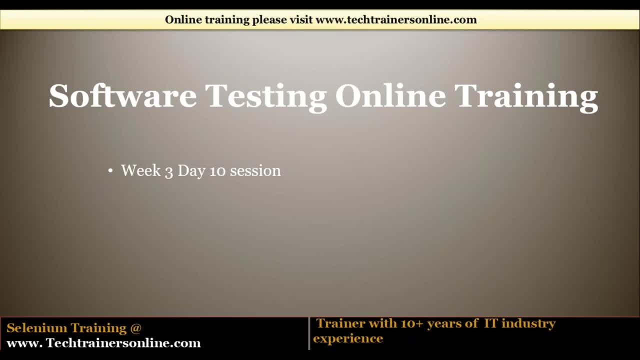 ms office is your product, so you have to buy it through online or you have to buy it through the cd and then you have to go through the installation process. so if you guys are working for this kind of project like this, so what i'm going to do is we are going to do a 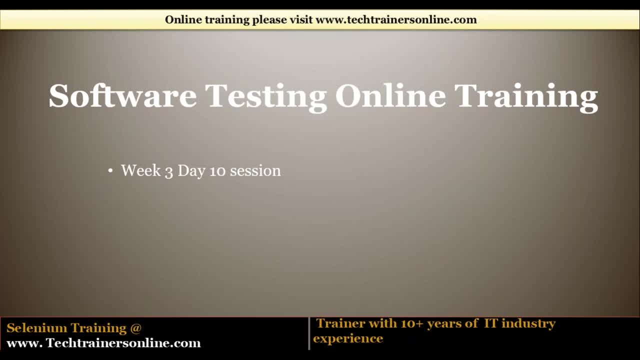 the installation and as well as uninstallation testing, also as part of types of testing. and when it comes to the automation, we clearly mentioned that regression testing we are going to do with the automation only. so, in automation, what are we going to do? in automation? we are saying that 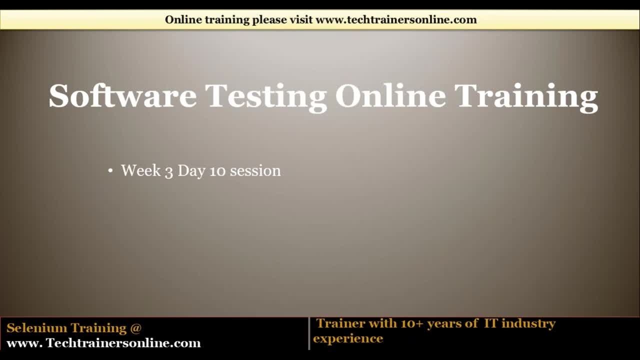 we do functional automation and non-functional- non-functional- as part of automation. i'm clearly saying that i'm also going through the performance testing which we already discussed. even performance testing also falls under automation. so when i'm talking about the automation, i'm trying to clearly define what is the scope for automation here, right? 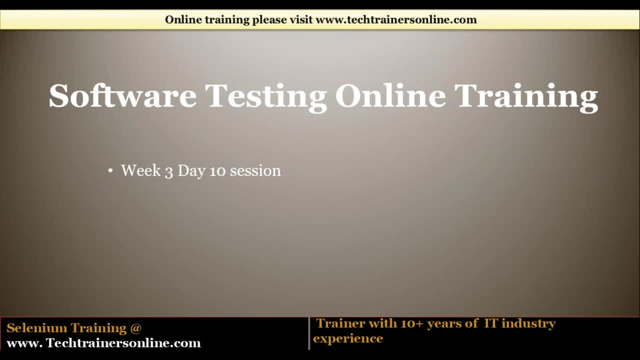 so what is my scope for automation? my scope for automation would be functional automation and, as well as the non-functional automation, testing which i'm going to do it. so then, i'm talking about what is the tool i'm going to use? selenium is the tool which will be used for functional automation. 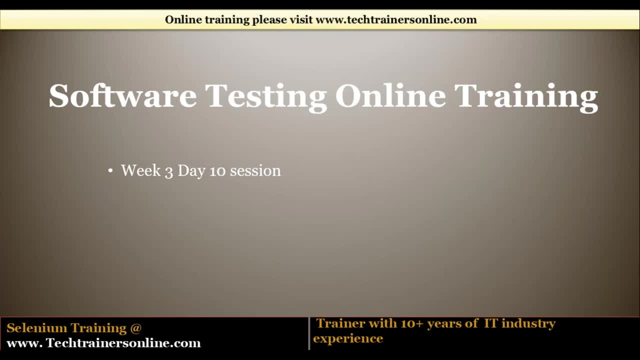 testing. i'm clearly mentioning that what is the tool that i'm going to use as part of my functional automation testing? and then load runner is the tool which is used for the performance testing. so i'm also clearly defining what is this scope for automation? scope for automation is functional. 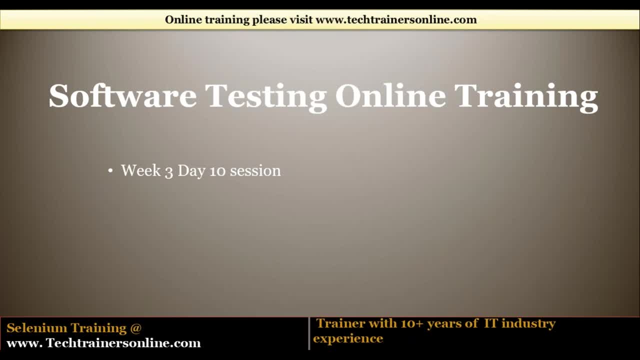 and non-functional automation testing. for functional, which tool i'm going to use. for non-functional, which tool i'm going to use. so this is what i'm trying to define it in the automation testing. right, and moving on to entry criteria. entry criteria: what do you mean by entry criteria here? any idea? 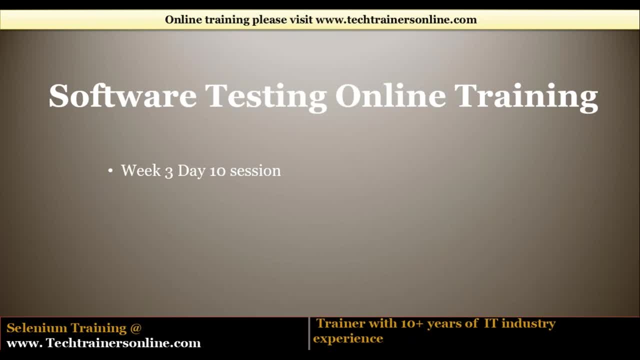 and to graduate, like in case of facebook, we have taken example in that, like, age is a criteria that 18 should be covered and that age is a criteria that 18 should be covered and that age is a criteria that 18 should be covered. okay, so entry criteria means: when can i start my testing? 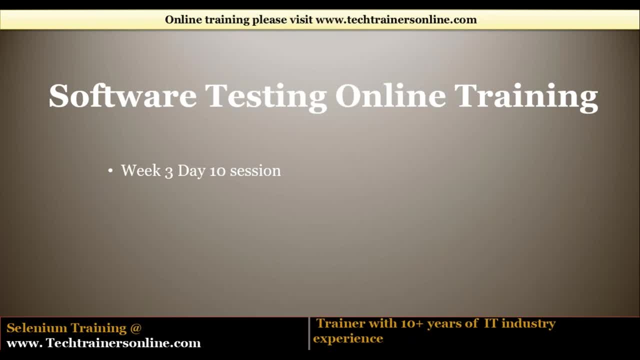 when can i enter into? when can my testing team can start doing the testing? so that would be my entry criteria, right? so test environment setup should be completed. the test environment setup should be completed. so i wanted my test environment should be completed, be developed and all users- i mean all the testers- got the access to it and their user credentials are created. until, unless the test environment is not set up, i would be not able to do any testing. that's entry criteria. and testing team provided access to this environment- right testing environment. and all the test scenarios and test cases are prepared and ready for execution. so i don't want testing team to do the testing without test cases. so what i'm trying to say is: all the test scenarios and test cases are prepared and ready for execution, so i don't want testing team to do the testing without test cases. so what i'm trying to say is: all the test scenarios and test cases are prepared and ready for execution, so i don't want testing team to do the testing without test cases. so what i'm trying to say is: all the test scenarios and test cases are prepared and ready for execution. so i don't want testing team to do the testing without test cases. so what i'm trying to say is all the test scenarios and test cases are prepared and ready for execution, so i don't want testing team to do the testing without. 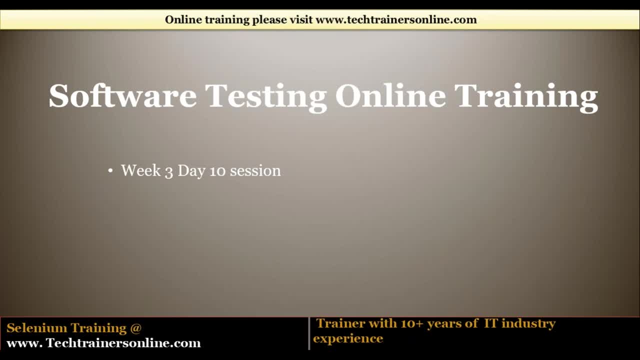 test cases should be prepared. all the test cases should be prepared and they are ready to. they are ready to execute it, and test cases are reviewed and approved by client if applicable. so what are we trying to say here? the test cases. whatever i said, peer review will be happening once you. 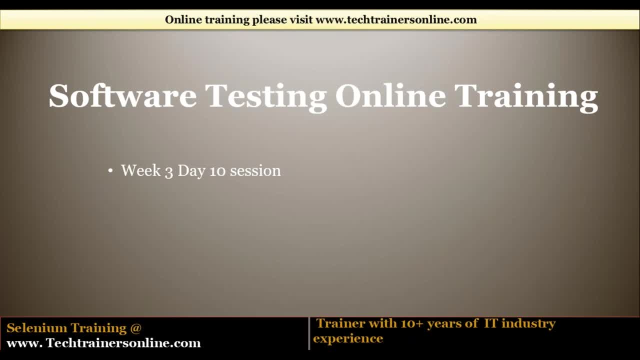 guys prepare the test cases. there will be a peer review once the test cases are prepared and, uh, you know other guys are to review, sometimes even client also going to review your test cases and refer to client to client. again, it's not 100 percent that every time client will review. 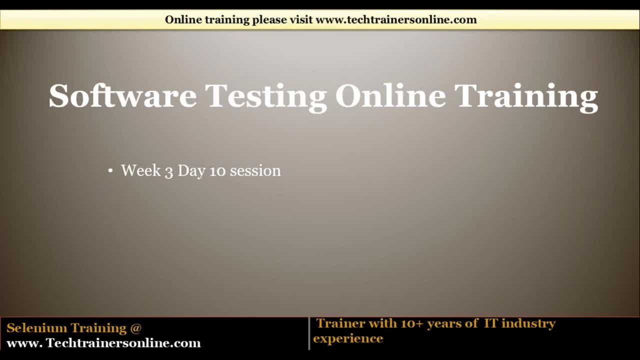 so if client is reviewing and make sure the test cases are reviewed and approved. also, all the tools related to automation is purchased and ready to use. i was talking about automation. i will be using the load runner. so load runner is not a open source, it's not a free of cost. 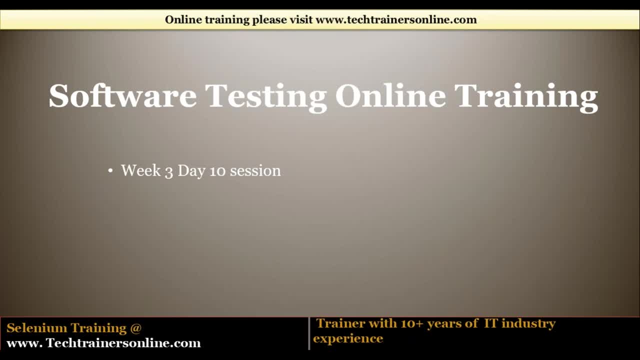 it's a licensed version where you guys have to go and where you guys have to go and purchase the tool. so what i'm trying to say is load runner tool is purchased and it is ready to use, and the next one, test management and defect management tools, are purchased and ready to. 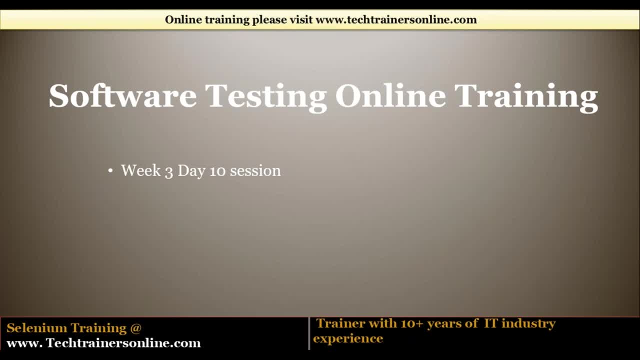 use. so what i'm trying to say is the test management and defect management tool as discussed. we write the test cases in the test management tool and we write the. we raise the defects in the defect management tool. so there are plenty of the tools available in the market, right, and most of them are the licensed version. where you guys 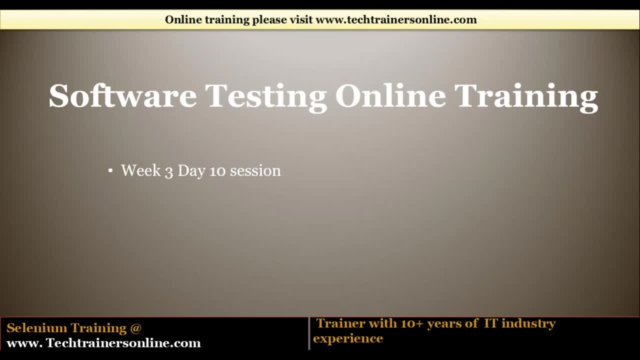 have to go and purchase it right. so typically, whenever you guys are going to use the test management and defect management tool as a test manager, i need to make sure that i purchased license for the using the test management and as well as the defect management management tool and it is ready to use for the team. and again, login credentials should be created. 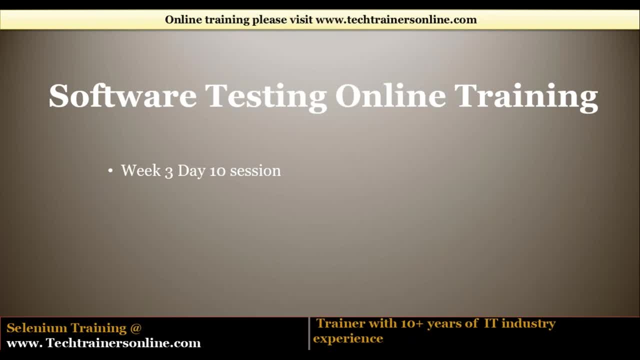 for all the testing team members and as well as to the defect management tool. also, team got all the relevant KT on domain. now let me give an example. if you guys are working for a banking application, there's a. banking is one domain, insurance is another domain, healthcare is another. 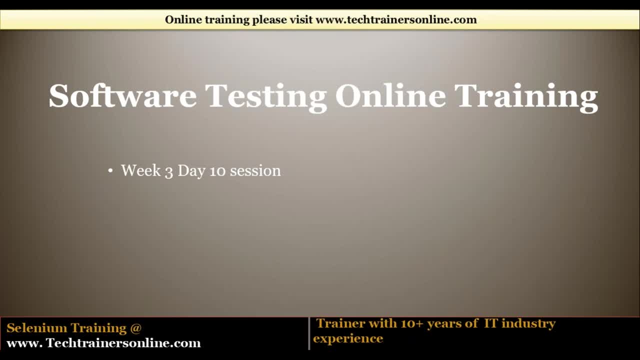 domain. you know, e-ticketing is another domain, so you guys will be working on in a project which belongs to the different domains. maybe today I'm working for banking application- it's known as a banking domain, right- and tomorrow I'm going and working on insurance domain. so what I am? 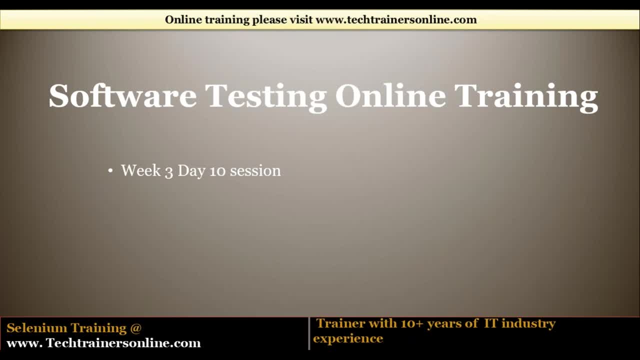 trying to say here is: as part of my entry criteria, team got all the KT related to domain. so if you guys go and talk about insurance, there is something different. terminology of the words will be used. they say that: what is the copay? do you guys know? 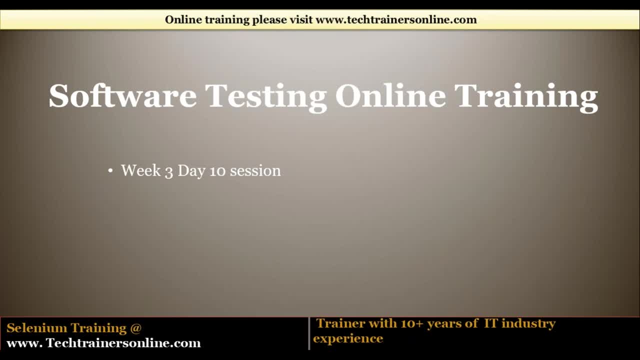 what do you mean by copay? it's nothing but how much you have to pay and how much insurance company will pay for it when you claim for insurance, right? so some people say that 2080 is a copay. so we need to understand the terminology of the words specific to the domain in which you guys. 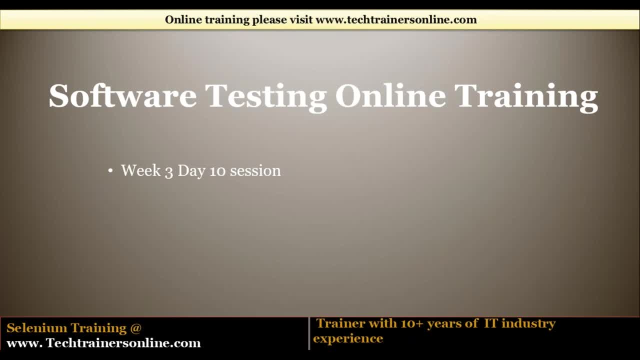 are working in. when I say copay, so 20 percent, I have to pay, so that is known as a copay. so banking also has their own. banking also has their own terminology of the words, like due to co-wire- sorry, due to this covet. and banks are, you know, ignoring the. it's not ignoring. banks are giving an opportunity for. 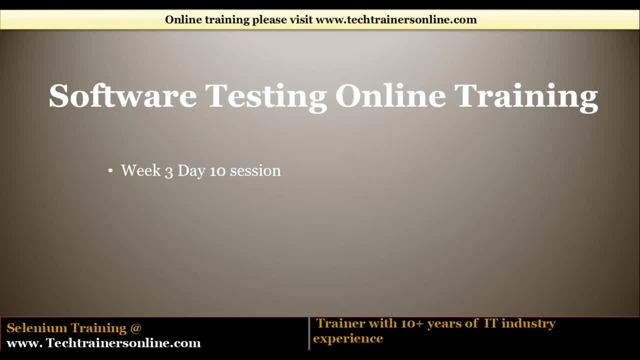 their loans. what is the terminology that used? I am not recollecting that you can postpone your emis right, moratorium something. what did the word they use? so you also need to know the terminology of the words that are used in banking domain or any domain which you guys are. 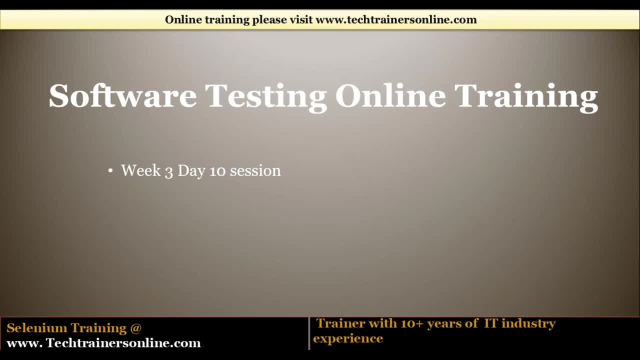 working in. so nowadays no client is providing the banking domain training. earlier you know when I was working for one of the biggest MNC company and it is purely for the banking applications, they were very famed for banking applications. most of the major banks are their clients. so whoever is joining, 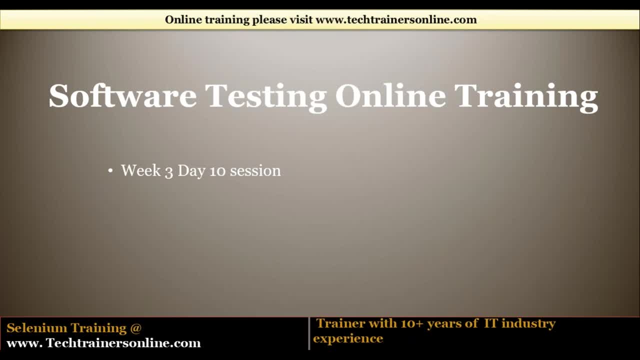 in that company. as part of the banking formalities, they used to provide a KT on banking domain, because you will be placed only on the banking application, so is the KD is given on the domain or not? that's what we are trying to talk about here, but it it has become on a complete non-requirement. nowadays no one is giving a. 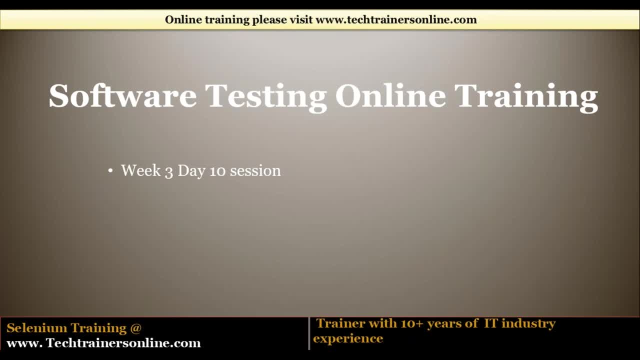 training on the domains. right team got training related to test management and defect management tools asset. we have to purchase the test management and defect management tools and maybe you are working test management called test link today in one of the project and you are moving into another project where, where they are, where they are using the, where they are using the. 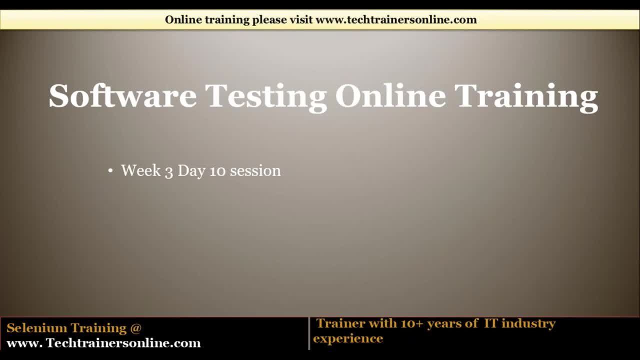 another test management tool right, so generally we would expect some KT. KT means knowledge transition, so they generally we explain, we generally explain to the team members, whoever is joining to the project on the test management right now. all these things should be ready. then only I can go ahead and start my testing. this is known as an 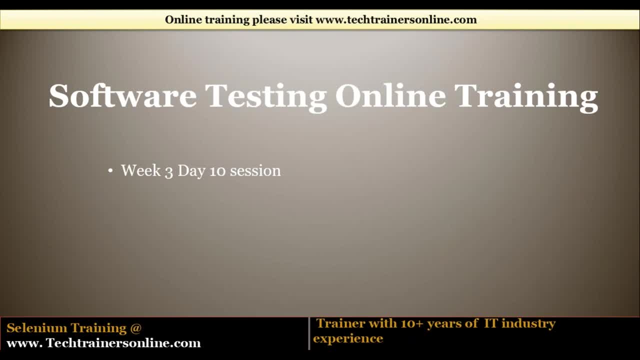 criteria. any questions on entry criteria? in short, sir, that we are making a complete platform for testing the, the product which we have to test, right? Hello, Hello, You, You, Hello, Yes, Yeah, I think there was this connection of the internet. It's restored now. Yeah, 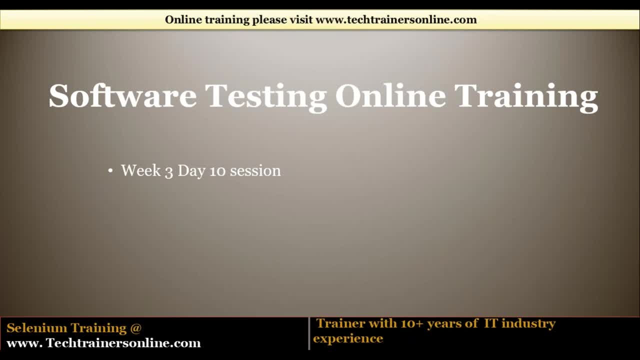 Yeah, I'm sure asking some question, But in short, in Test plan we are creating complete platform there, like a product will comment how to test and which are the different steps. Everything is should be ready means like it is a complete creation of environment, right, Yeah? 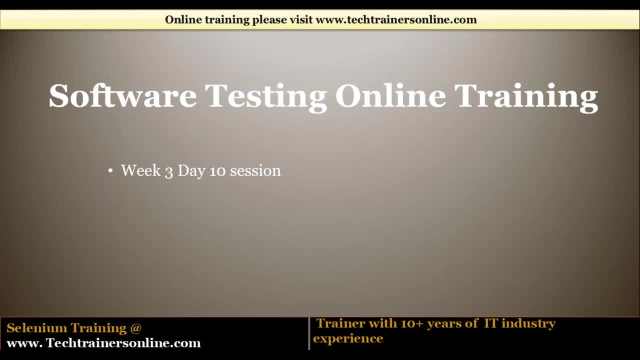 And so the second thing is regarding Your code hours about functional testing. I go in functional testing, We are using selenium for automation And performance testing for load on a right, but in case of test management tools, Which are the services, are different test management and different management tools. 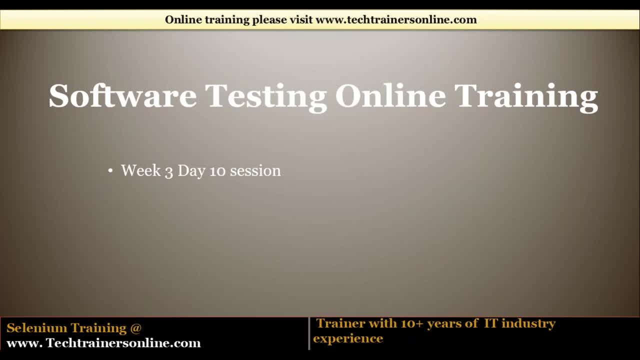 Like you have a test management, like a test link. you see quality control Management you have. you have Zira, Mantis, Mozilla, PFS. There are so many tools available in the market. Zira is designed management tool. Now you can use zero for raising the defects also. 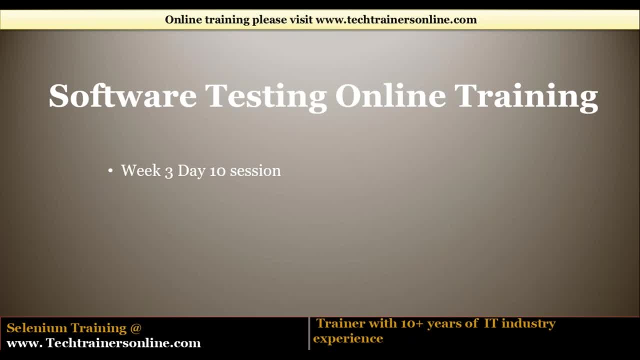 Zero, zero, zero. Yeah, zero is majorly use it for a giant, For other kind of project management stuff. but you can still go ahead and refer the different management also. So we will learn Jira tool in detail. So With this, with this, today session, 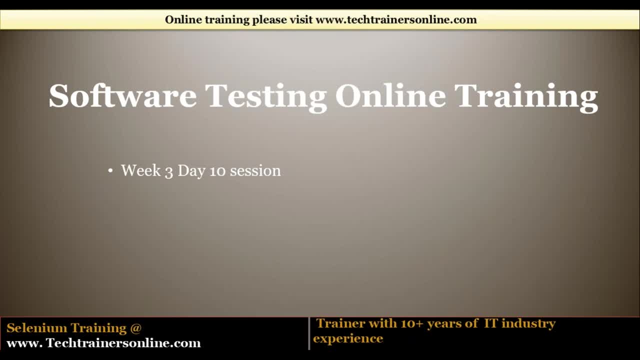 We are done with the manual testing and we'll be completely working on the tools management. Like what is the test management tool? we try to install test link and try to explore and, You know, create the test cases. I mean execute the test case, this in the test link, and then raise the defects in the defect management tools like Mantis or Zera. 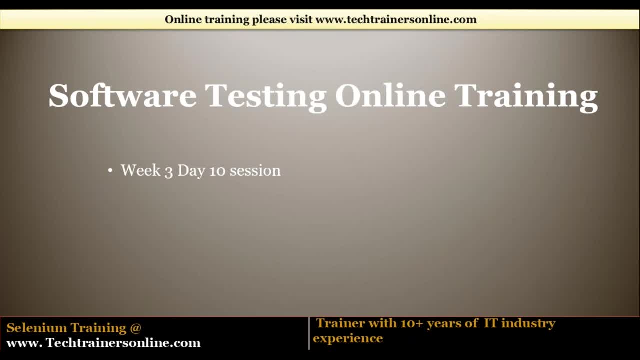 So from tomorrow- I mean tomorrow, from next week onwards- will be people working in the tools management. So, sir, I'd like you. you told us that these are licensed version, so whether Crack version is available, trial version will be there for one week or so. test link is: 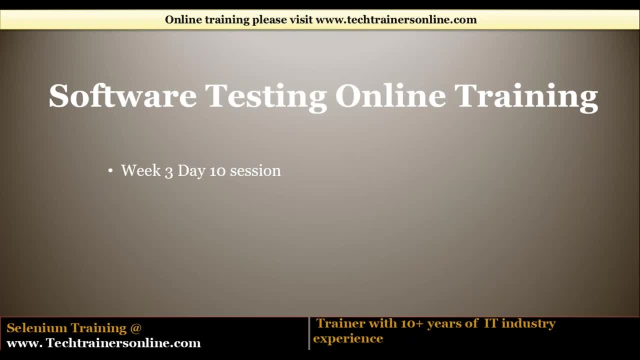 not a licensed version. it's an open source, free of cost. we can download and use. okay. but when it comes to zira or mantis for the defect management tools, they are not free of cost, but they give you trial version of one week or two weeks so we can use that for one. 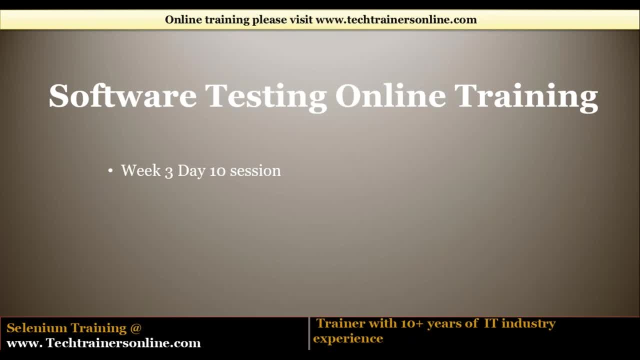 week or two weeks just to explore how it works practically okay. okay, so exit criteria. what do you mean by exit criteria? hope you are clear with entry criteria. opposite to entry criteria is nothing but exit criteria. when i have all these things in entry criteria, i would go ahead and start doing the- uh, what you call. i would go ahead and. 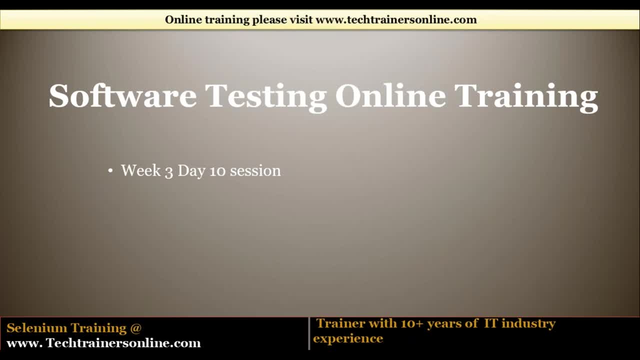 start doing the testing and it's a exit criteria: when can i stop my testing? when can i stop my testing? so it's difficult, as simple as it's mostly- to ask question: when do you think you guys can stop your testing? so when all test cases are. 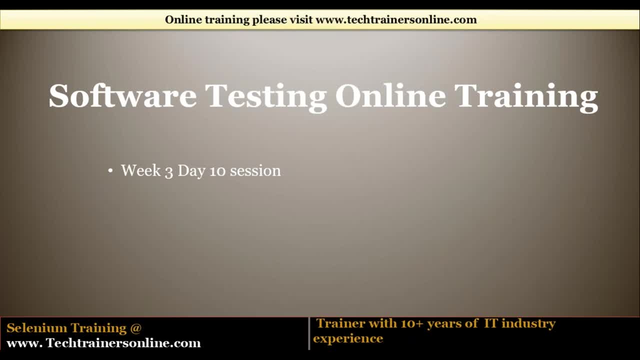 executed and 95 percent of test cases are passed. this number can slightly, this number can be slightly changed. this number can be slightly slightly changed here and there. someone will say 95 and someone will say 98 percentage, someone will say 90 percentage. the client to client. and we need to discuss with the client and understand what is the. 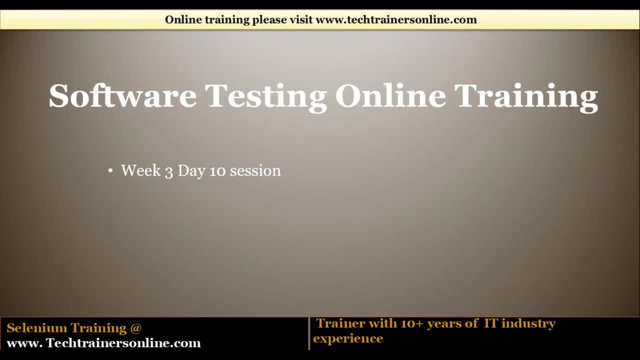 criteria that you are looking for. we have written the test cases. we are going to execute the test cases. what is the percentage of the test cases you think? what is the percentage of the test cases you think that we have to mark it as a pass, then we can stop the testing. so we are saying 95 percentage. 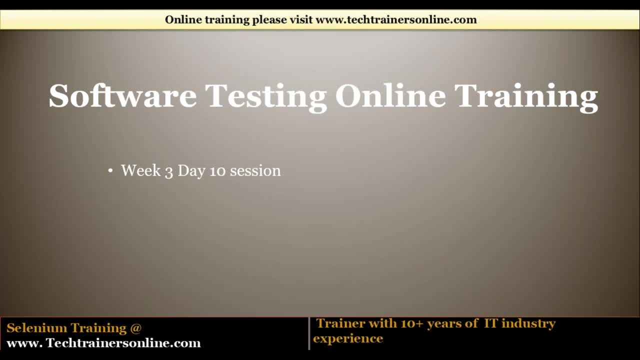 of the test cases should be passed. no test cases are in blocked status, so we also discuss: what do you mean by blocking your test case? right? when do you think you guys will block a test case we discussed it right? when do you think you would block a test case we discussed yesterday, i think previous session? 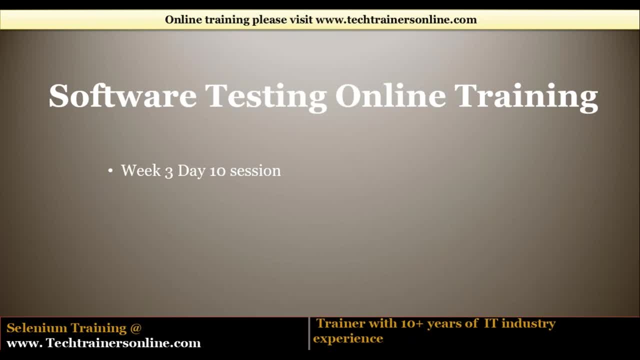 where we'll have three statuses of the test case: right, one is passed, one is failed, one is blocked. when do you block the test case? so whenever you see the dependency test case is not working, i am going to block my current test case. example: funds transfer. i cannot transfer the funds until unless i 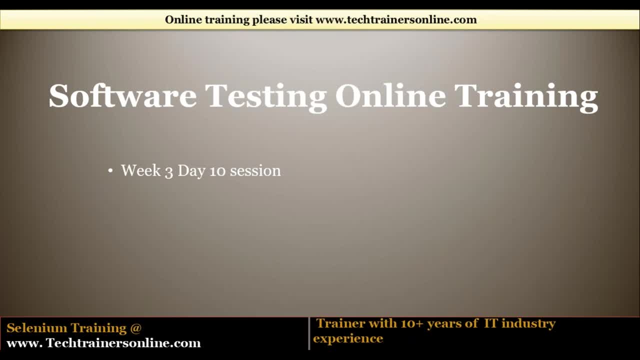 add a beneficiary. there is a defect in adding the beneficiary so i will block the benefit. would not be able to transfer the funds because because the adding adding beneficiary is not working at all right, so that's called as a block. i don't want any test case should be in. 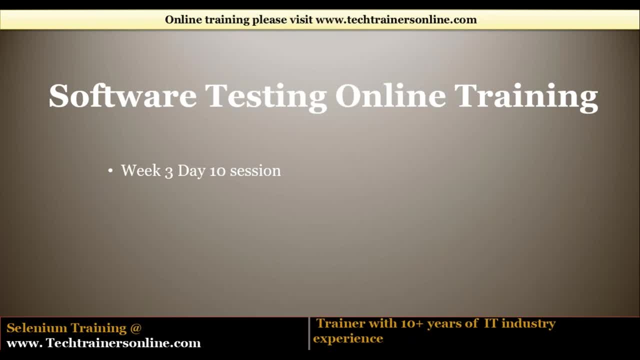 blocked status right and all the defects with the critical- high- medium severity defects are closed. i don't want any defects which is kept in open. with the severity of critical high and medium, there can be low severity defects. we will discuss what you mean by severity in today's session. 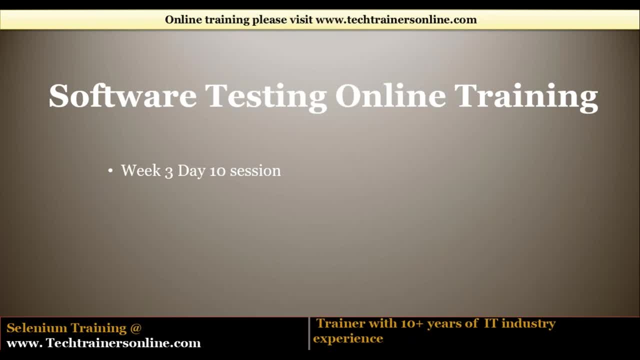 itself. so don't worry. so there should not be. there should not be any defect which is kept in open. with the severity as critical high and the medium, there should be zero defects with this severity is so that's what exactly called exit criteria. let me add one more point. there can be max of five defects. 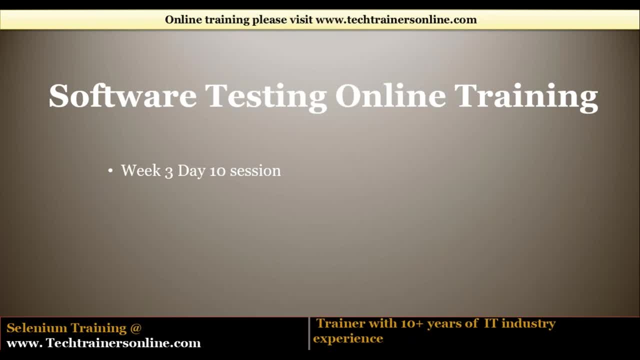 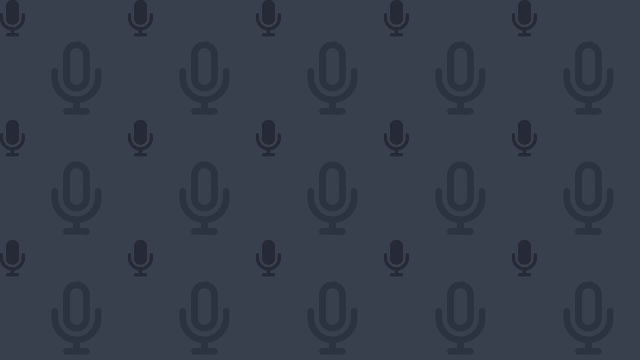 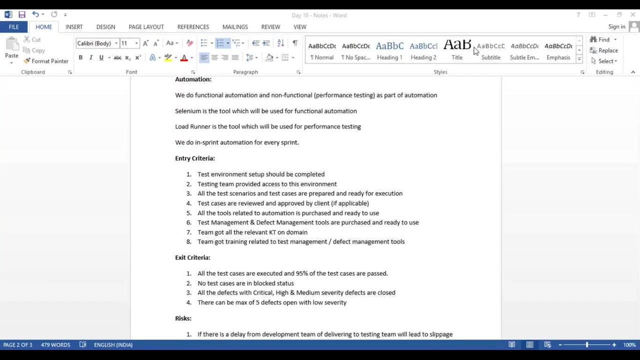 open with low, with low severity, you can. you can still have five defects open and there can be a system with a defect, but we are not able to see your screen, sir, parents, yes, sir, yes, let me stop and share it again, fine, okay. so what i'm saying is, as part of exit criteria, there can be max of five defects open. 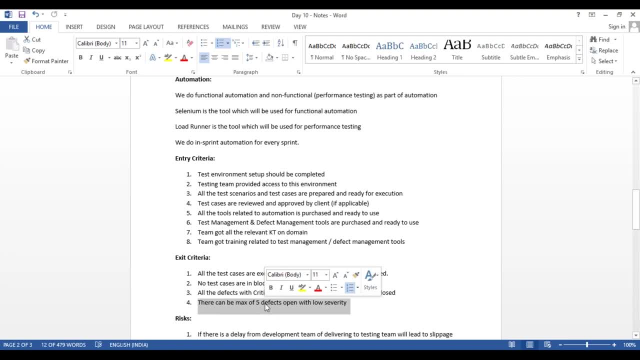 with low severity. that's what i mean to say. you can still have a defects in your system with low severity. you can still have a defect in your system. max of 5 and it is open. with low severity, that's what i mean to say. you can still have a defect in your system. 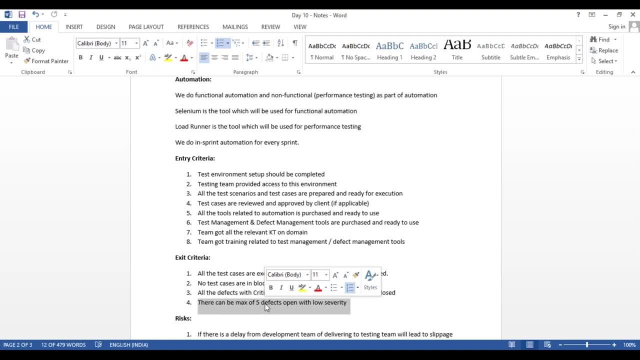 of 5 and some people will take 2 defects. some people will agree with 4 defects, some people will go with max of 5. so no client is going to take the system with the defects. okay, so, but that can be okay. you can still go ahead and release the. 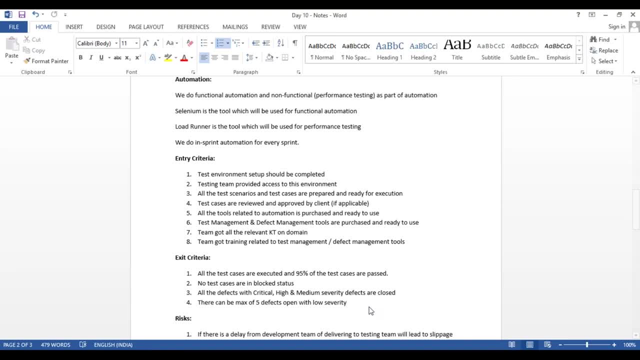 system with the defects, but there should be low severity defects. that should be my exit criteria. so exit criteria: if someone is asking a question, when do you think you can stop the testing? that would be your exit criteria. what is written in the test plan, mostly interview ask question. when do you think 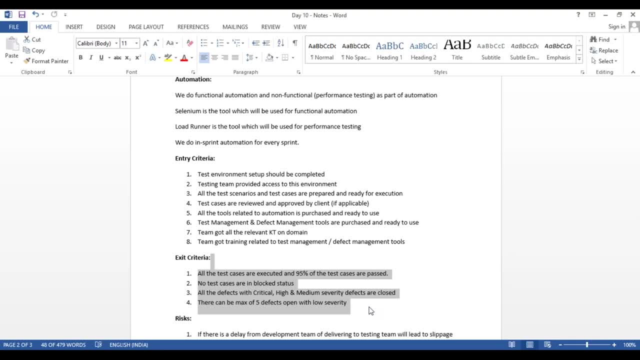 you can stop the testing. the answer is: as per the criteria that is defined under exit criteria in the test plan document. that would be your answer. if someone asks again: what is the exit criteria that is defined in your plan. so could be your answer. these are the four points you can highlight. 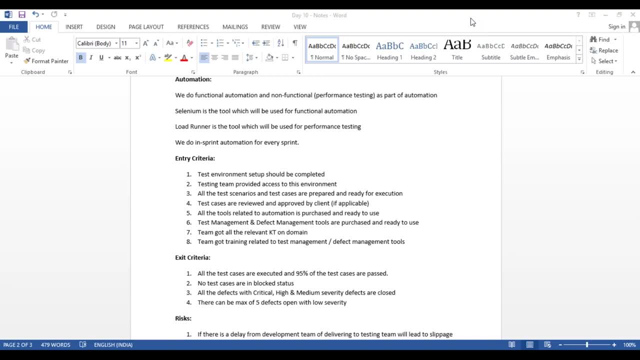 any questions on entry criteria or exit criteria. so client will generally say the execution of test cases should be hundred percent. i didn't get your question. like we are saying that 95 percent of test cases are passed right. so maybe that and or it depends on the client to client. 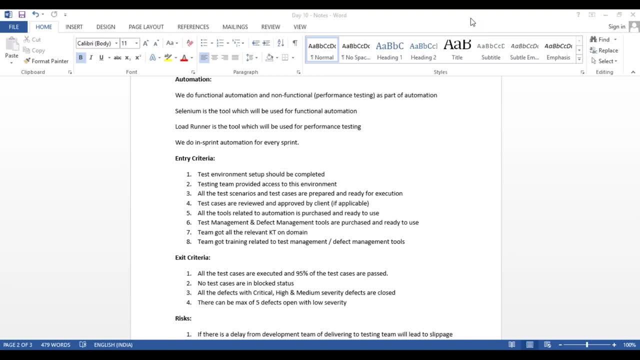 so the client can generally will say it should be 100 test cases should be passed. yeah, they can say: then we have to go for 100. correct, then that that is the case. this will work right. no test cases in block state means all the test cases are executed. okay, then there should not be even a single defect. 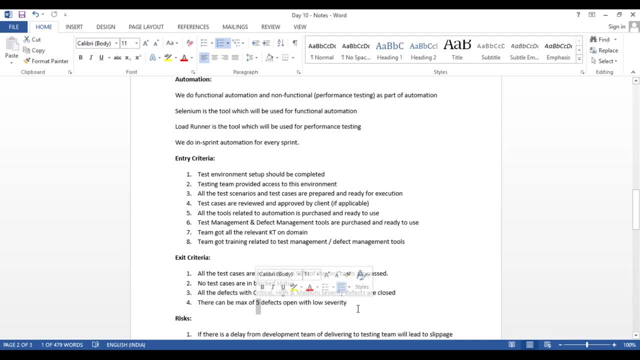 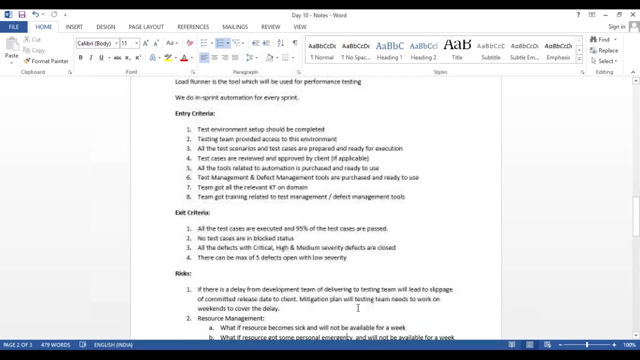 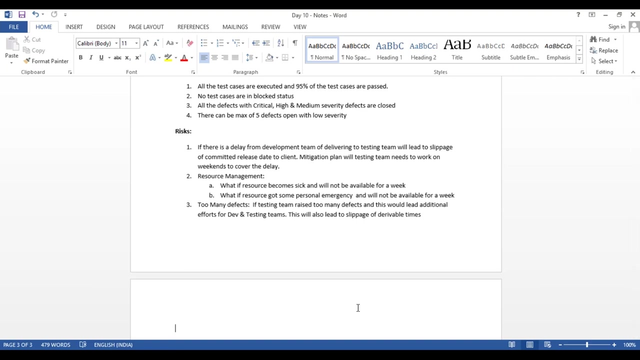 also because if you have a five defects, open five test cases are paid. yeah, okay, it differs to client, okay, okay, now let's move on for the risk. what are the risks we have? so every project will have some risk. risk is something that may happen and that may not happen. 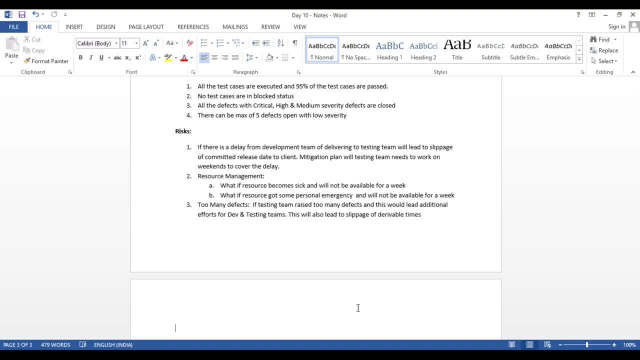 so what do you mean by a risk which may happen, may not happen, we don't know, but we are predicting there could be a risk here. so if this risk is a risk, then we are predicting there could be a risk here. so if this risk is going to happen, what is the mitigation plan for the risk? 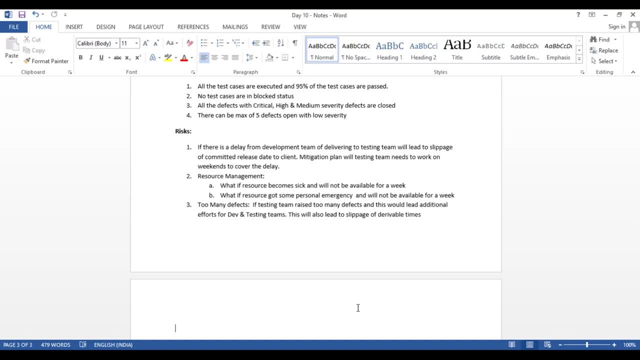 right, so that's what we always talk about the risk here. now, what is the risk from the testing aspect of you? if there is a delay from development team of delivering to testing team to testing team will lead to slippage of committed release date to client. so what? 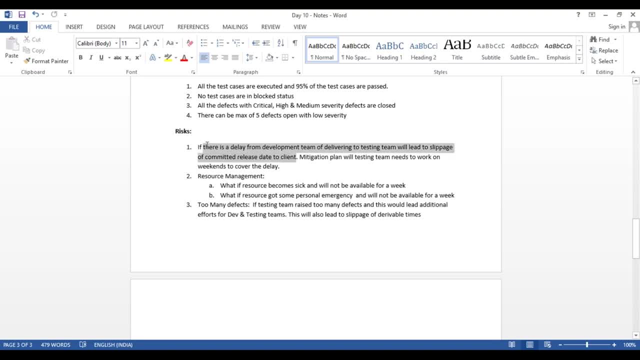 do you mean by with this statement? now, let's say that the december 31st is the date when we have to release it to the client for the testing, to user acceptance testing. now what did we consider? it's total one year project. out of one year, nine months are given to the 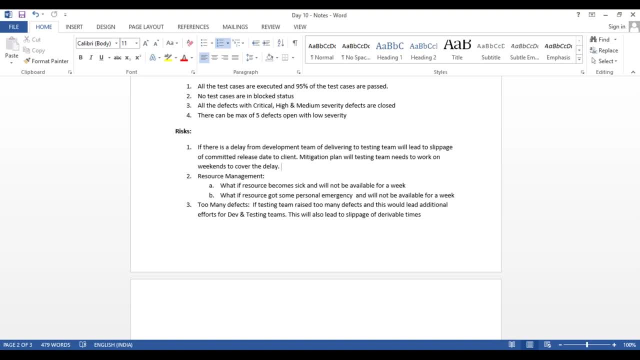 development team, architecture and all the stuff, but three months time, we estimated for the testing, where the testing team will take three months in the next three months we are planning to take, you know, october, november and december. these are the three months we are planning to take it. 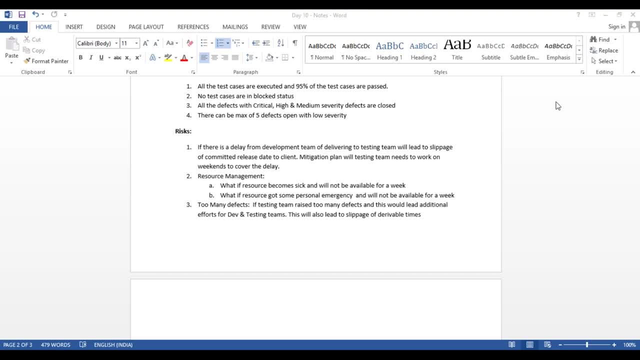 so when i'm saying three months i need to take, i generally expect october. first is the time when i should get my system for the testing team, so it should be given to the testing team on october 1st so that i can spend three months time: october, november and december. 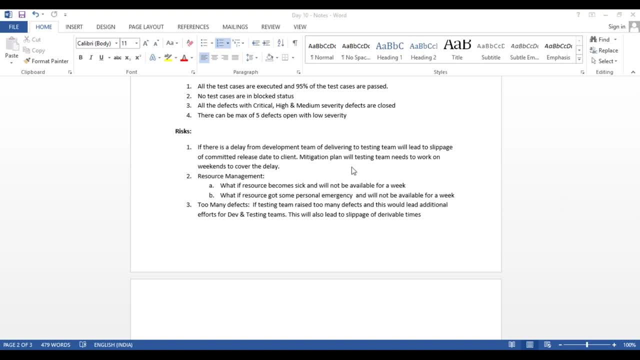 what we are delivering your system for UAT. Now there is a delay from the development team. So what is the time they should give you for the testing team In October 1st? But what is happening? let's say that they have delayed for two weeks of time Instead of October 1st. let's say they have. 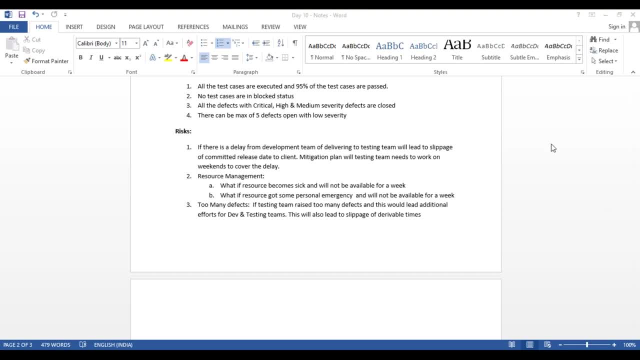 given you on October 15th. What would what do? what will happen? So testing team will not have sufficient time of testing estimation: Three months. we agreed and we agreed 31st December what we are delivering it to the client, But if you do not see 15 days, if it is not delivered on. 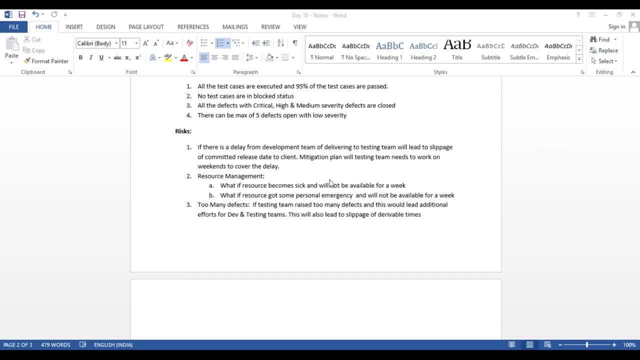 October 1st. so your development- sorry testing- team is losing the 15 days. So why should I? you know I cannot go and tell to the client. you know it's all internal team: development and testing. both are from the same company. I cannot complain. 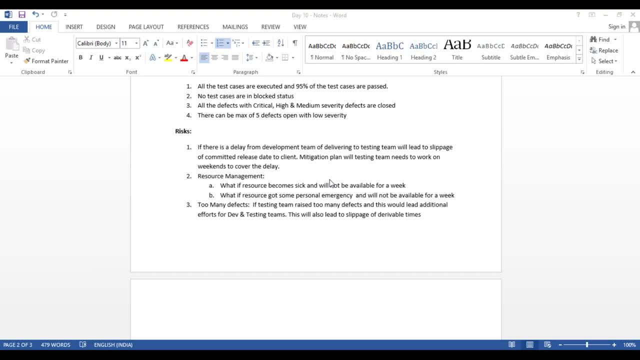 About my team to the client right. I cannot tell that your team did not give me on time So I can't deliver it to you on time. So we cannot, we cannot say that. So there is a risk. I said it may happen. 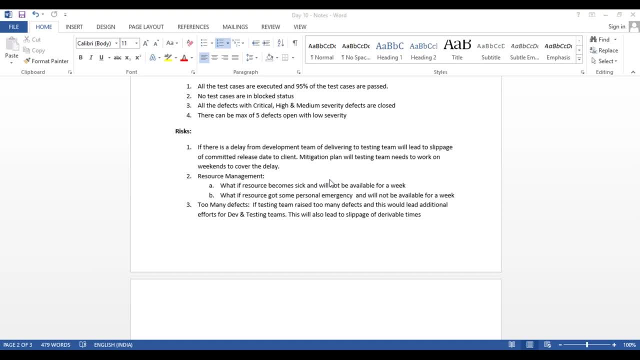 it may not happen If there is a delay from the development team to delivering it to the testing team. If there is a delay, then what are we trying to say is that it would lead into slippage to the UAT date, What we agreed with the client. So for every risk there should be a mitigation plan. What do you mean by a? 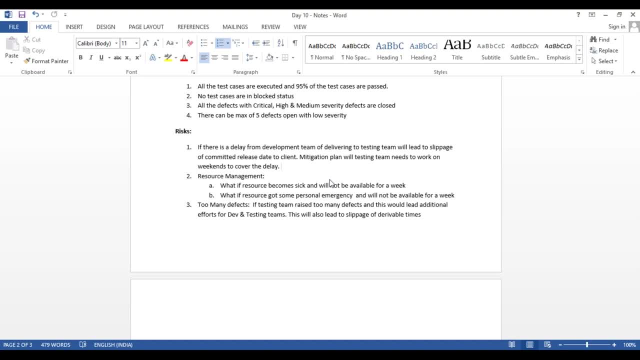 mitigation plan If the risk is going to happen, how I am resolving that particular risk risk right. So mitigation plan will be: testing team needs to work on weekends to cover the delay. Are you guys getting what I'm saying? I wanted my team testing team should go on work on the weekends to support that 15 days. 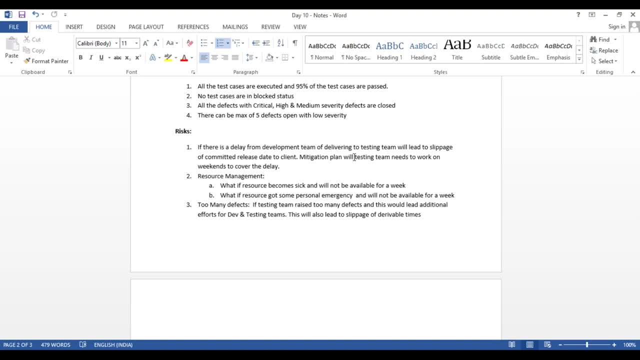 Delay so that I am on timeline and the committed for the dates that I have agreed with the client. So I'm also going to highlight that particular risk in the test plan. Any questions on this particular risk. The first one is not only on the weekends. team can even stretch more daily, two hours extra, whether than eight hours work for 10 hours. 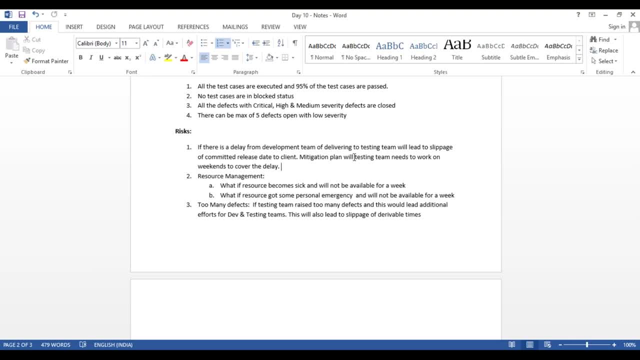 And cover those number of hours that are delayed so that you meet it on the time. client will not agree. It's all together, your team, You guys go ahead and fight internally or do whatever you wanted to do it. You agreed to deliver it after people. 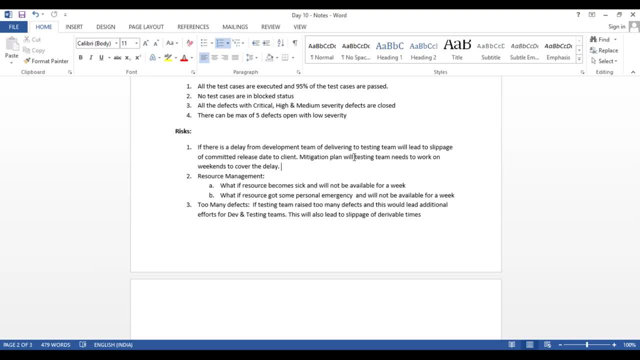 You'd give it. you know that the first, that's what clients stick to it. Okay, So the second one is the resource management. So what if resource becomes sick and will not be available for a week? Now we said the first risk can be from the development team. 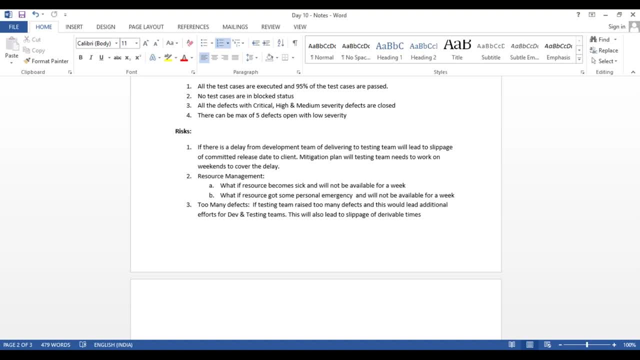 If they are delaying. it's a testing team. it risk to the testing team and we cover it by stretching extra hours or the weekend. now what if? what if resource becomes sick and will not be able to work for a week of time? so i estimated eight hours for every resource. based on that, only i come to. 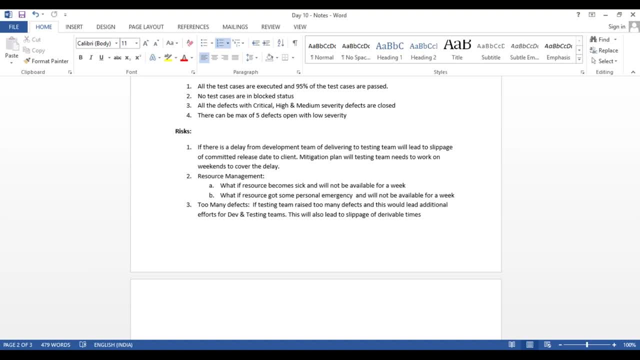 conclusion that because is the data? i need three months of time now. what eight? one week? if the resource is not developing? how many number of hours per day you work? eight hours per resource, then 40 hours gap in there, right? so if the resource is not coming for a week due to seek, 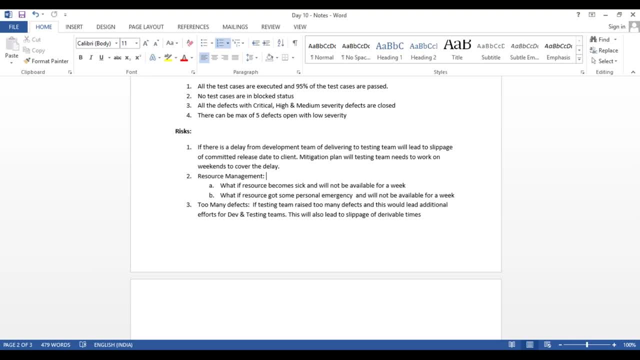 or some personal reason, there could be anything right. if that particular resource is not available, there can be a risk. so what i have to do is i have to mitigate this risk now if i have given it to tester who is a unplanned sudden sick or goes personal emergency on leave. 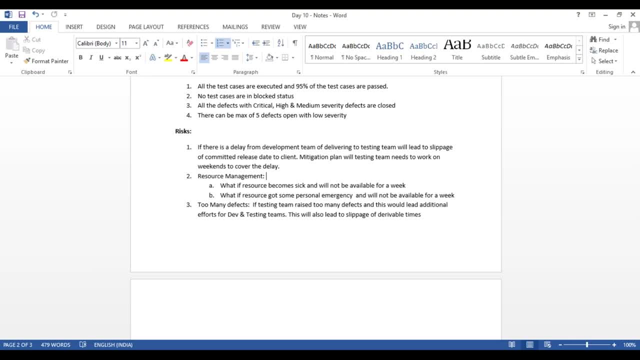 i have to assign the tester one work to tester two, tester three and tester four, so i have to distribute this 40 hours of work and make sure that it is being delivered. that would be the mitigation. so what if resource got some personal emergencies will not be available for a week. that's what we just discussed now, and another risk is too many defects. 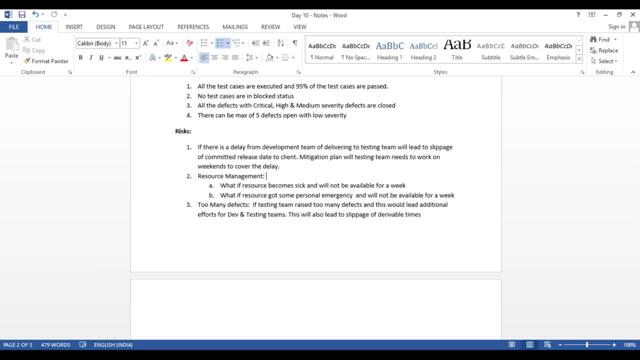 so what will happen if there are too many defects that are raised from the testing team that we discussed? right, what would happen if too many defects- like in the previous session we said on the test matrix 40 percent defects- are being raised? it would be high, time consuming. 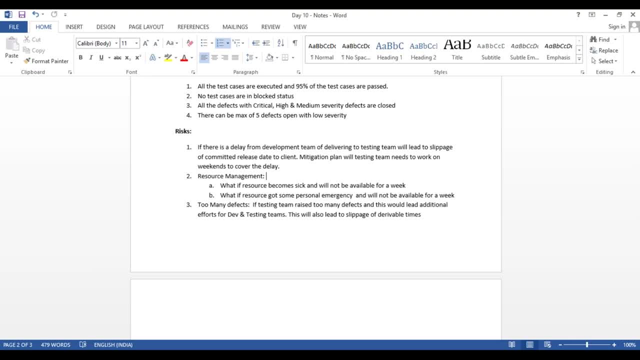 then they expected further development team and also to the testing team. so where the team has to keep fixing the defects. so that's what we discussed right. so that's what we discussed right. what would happen if too many defects and testing team also has to keep retesting the defects? so that would lead again into the risk. 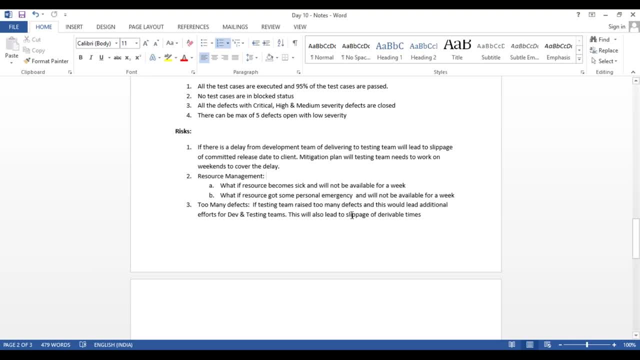 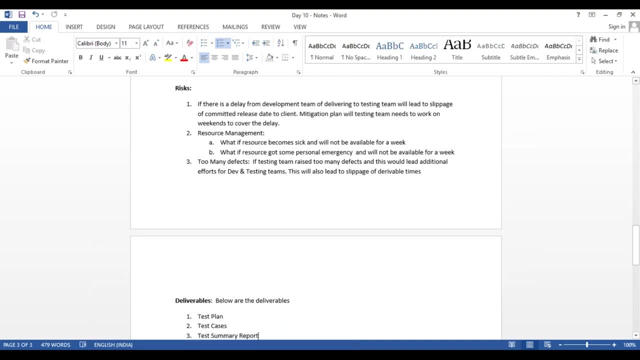 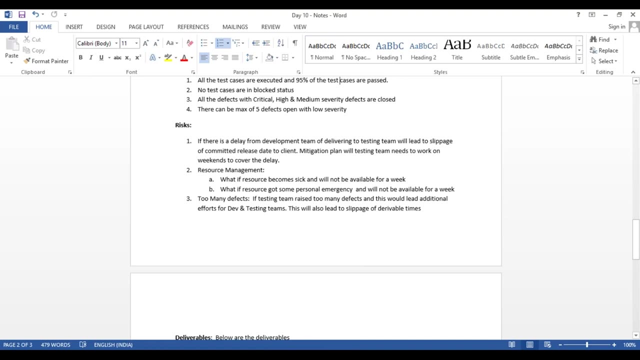 of my deliverable timelines. so this will lead into slippage of deliverable timelines. we need to make sure thorough testing is done by the development team before it's coming to the testing team. any questions on risk before moving on to next one? no, sir. okay, let's move on for the deliverable. so deliverables are nothing, but what are we? 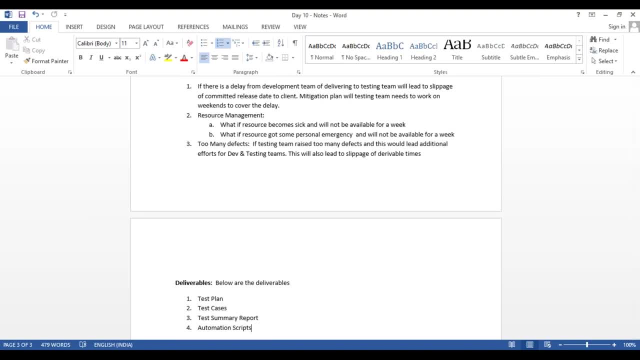 delivering it to the client. we are delivering the test plan document. we are delivering the test cases. we are delivering the test summary report. we are delivering the automation script. so, whatever the test cases have, i have automated. i generally write the scripts for that right, so i delivered. 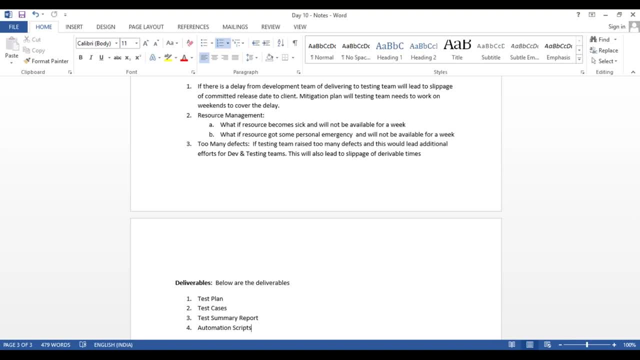 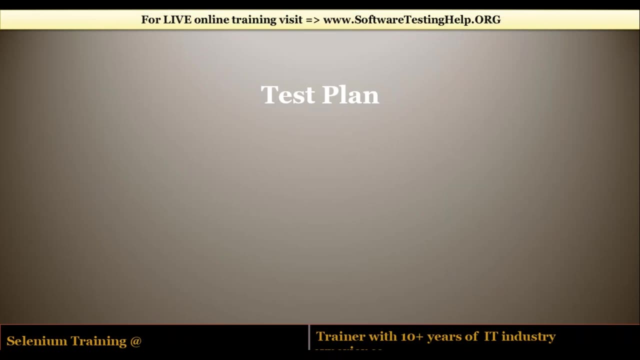 a particular script. so that's what exactly the deliver deliverables which we are giving it to. the are giving it to the client as part of my regular deliverables. okay, so that's all about the test files. any questions? yes, sir, that automation script. so automation script is, like, generally, a corner. 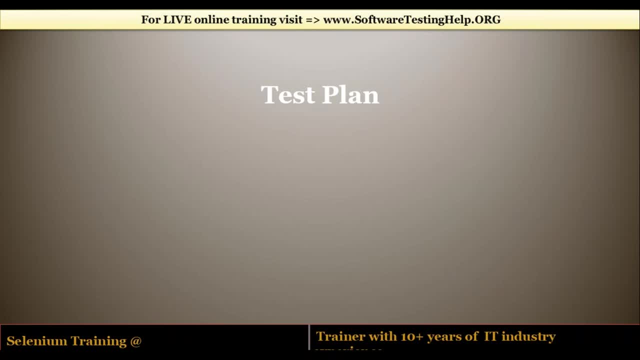 yeah, it's a code, so then, why we are going to deliver it to the client. is it necessary? because we are going to do the testing, so it is in our scope now. no, no, no, let you. let me give an example, like, say, you're working for a client, okay, and you targeted 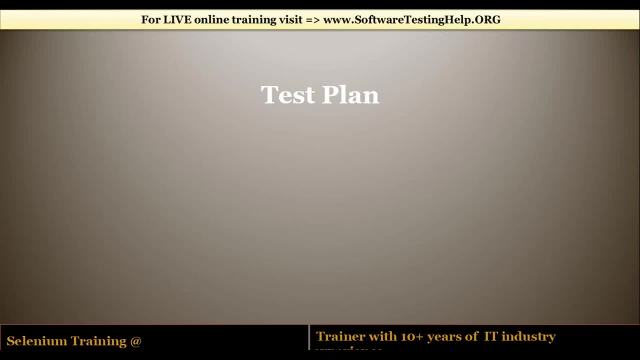 for six months, testing, right, yeah, and they have end-to-end flow. okay, now automated the end-to-end flow. let's say the banking application, creation of account, logging into it, transferring, blah blah. whatever the end-to-end flow, you have it. you already automated it. now your project is over. 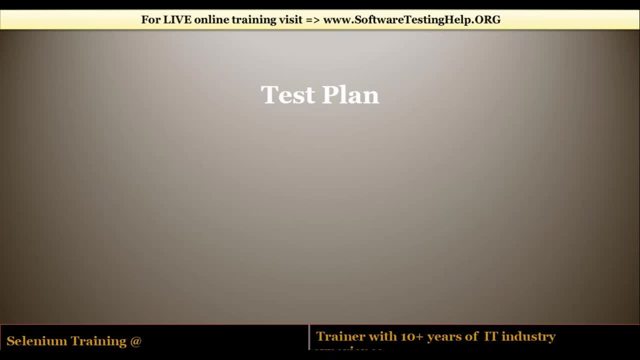 okay. so even though project is over, smart client will have small, minor changes and they are managing themselves. okay. they have very small team and there are no much scope for giving it to other company for outsourcing. then they are managing with two developers and one tester- minor changes. 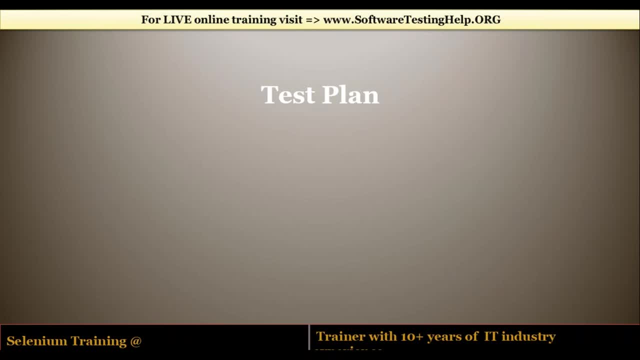 they keep getting it. production defects they are getting in right, so they have to still keep fixing it. so whenever they're modifying the code, they wanted to make sure that automation scripts are executed. i'm no more than that with the client. i'm done. so when i'm done i'm saying i'm done, i'm done. i have to deliver my 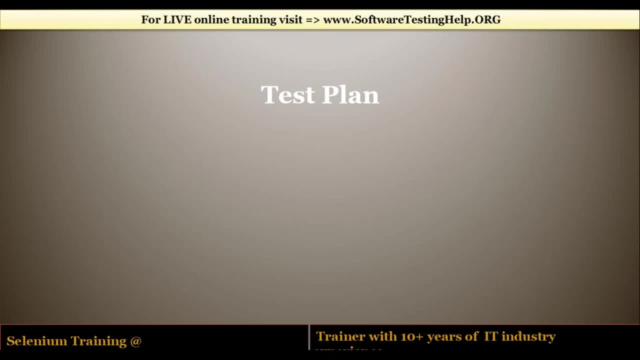 script to the client so that they keep making integration, integration suite for their product. what you will do with keeping the automation with nothing. is that clear your doubt? yeah, so we always our automation to the client and show that they are can go and run it whenever they want it. to make sure no impact on the particular system. let me 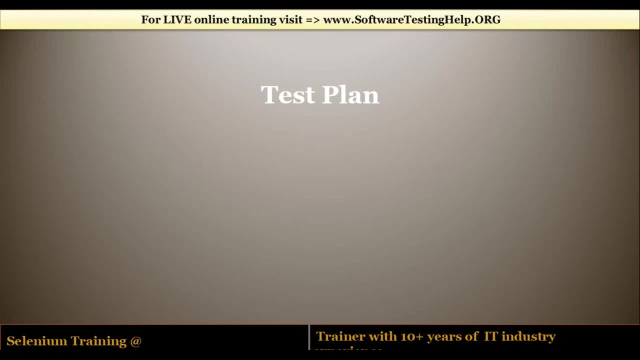 give you an example. did you guys hear something called a product, called salesforce, crm? salesforce is one of the crm product. right now, salesforce is a product or the technology, what i would say, rather, and my application is completely developed on the salesforce. 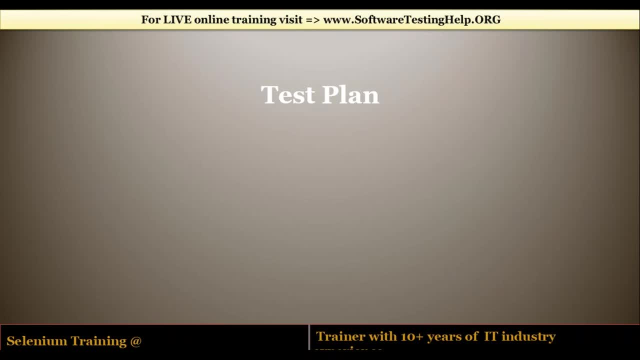 let me give you an example. i'm done with the project and everything is done, so salesforce is going to enhance their product. when i say enhance their product, it's ongoing product. okay, they have some releases called like winter release, summer release. you know, for every quarter they have a release. so when i say every quarter they have a release, they are keep on. 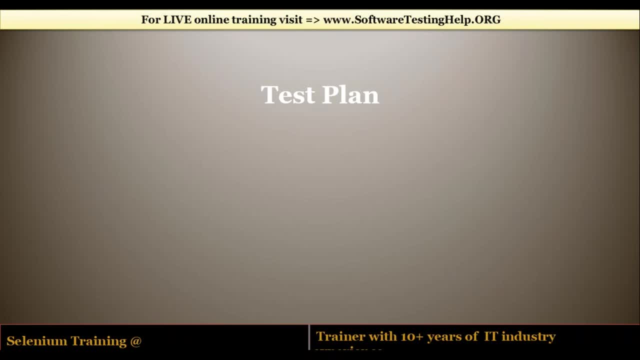 adding the new features to their product and, due to their product enhancement, it might impact to the my project because i use the technology right. so what i wanted to do? for every quarter, it is scheduled every quarter salesforce releases this particular release. it's a planned every year. so since my application is developed using the 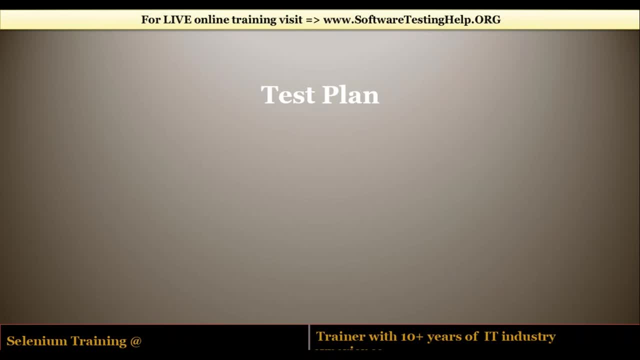 salesforce, because their product, which is called salesforce, is getting upgraded every quarter. i have to make sure it is not creating defects in my application. so what i would do, i would run these regression scripts just to make sure nothing is broken. okay, so anytime we have to give our automation script to the client, only we can't keep it with us. 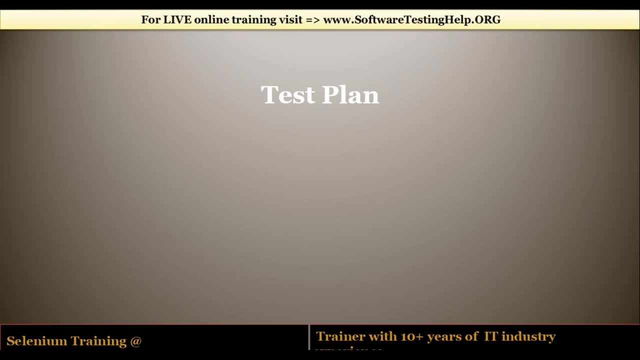 if you think we need to keep it, client will definitely ask: give it to us. so we have to. we have to deliver it to the client, okay, okay, any other questions? let me know before going to defect management. okay, so what do you mean by a defect? defect is something which is not working as expected. so as 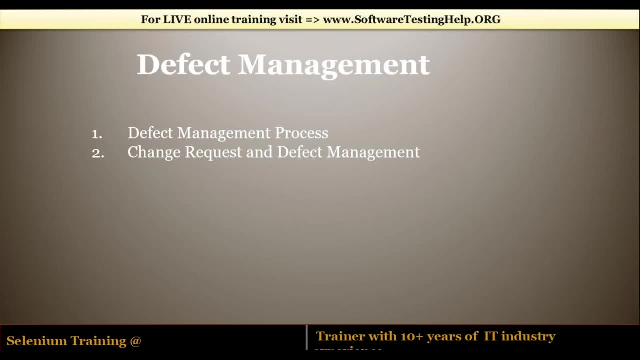 long as you see something is not working as expected, what are you going to do? you guys are going to raise a defect, so defect management process is all talks about what happens when you guys create a defect and how it flows after that, so that's what we are going to talk about. the 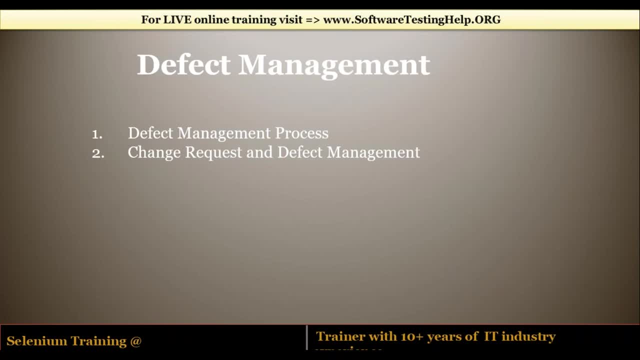 defect management. so we are going to talk about the defect management process on my page and you can see that we are also going to talk about the maintenance of the defect management process. so definitely there are many students of takes thisD warum wir arbeiten dabei. 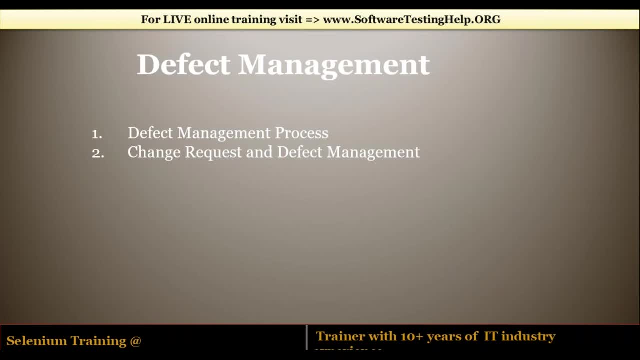 nämlich um. so most of the time, tester is going to raise the defects when they are doing the testing execution, whatever the test cases are prepared by them. so once they start execution of the test cases, they go for raising the defect. so what happens when the defect is raised? to whom? 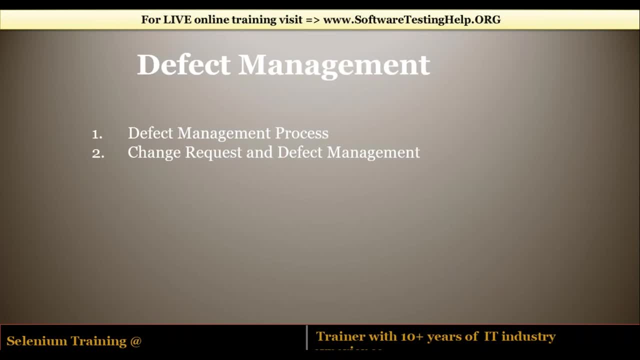 should i assign the defect? can developer reject the defect? if so, why they have to reject it can. So for raising a defect, we have defect management tools in the market. Like I said, Zira Mantis, Bugzilla, you know there are so many tools available. 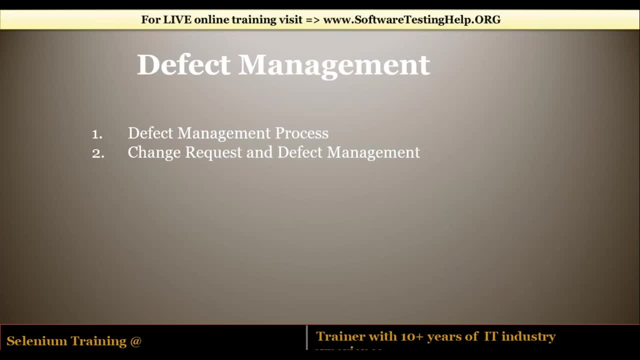 TFS. there are so many tools available in the market. Every client will be using some different tools, right? So as you are moving on to the different projects, you will be moving on exploring the different defect management tools also. So it doesn't mean that if I have thousand defect management tools in the market, it doesn't mean that I have to learn all thousand defect management tools. 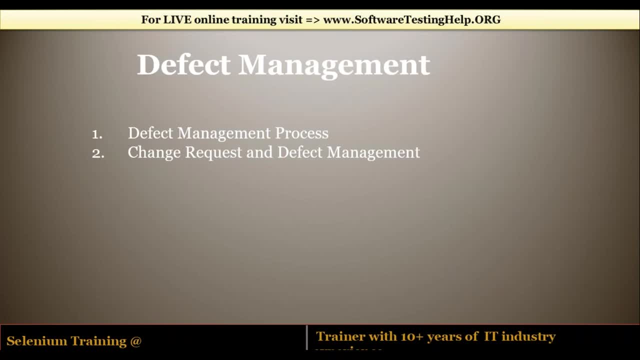 Answer is no. You don't need to learn that. The most of the defect management tools are similar. If you guys learn one defect management tool and remaining are going to be exactly similar. Here and there, slightly, there could be difference, Like label names would be different. 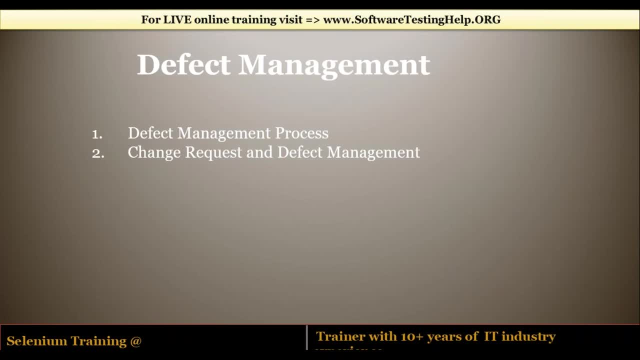 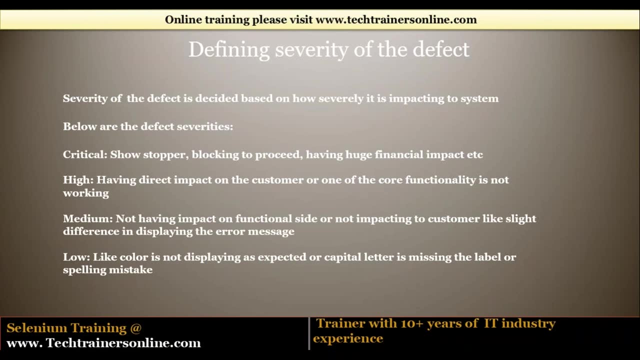 Some one or two fields will be extra added, Something like that, But not much More than that. Now, before raising a defect, what tester needs to consider is like: before raising any defect, the tester has to consider the severity and priority of the defect. 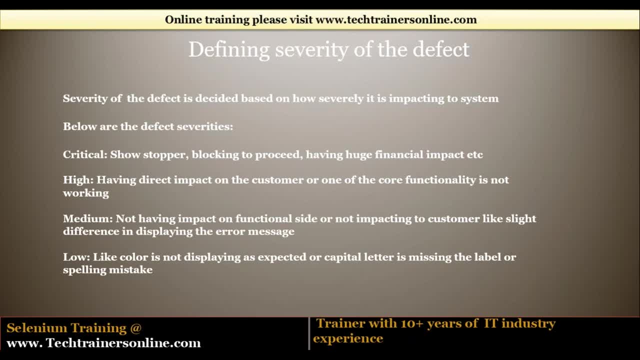 We will talk about what is severity and priority, And before to that, the tester for sure needs to check: is there any duplication defect? exist in it? Okay, Now let's say that you are working for a Facebook application. Now you wanted to test all the features of the Facebook. 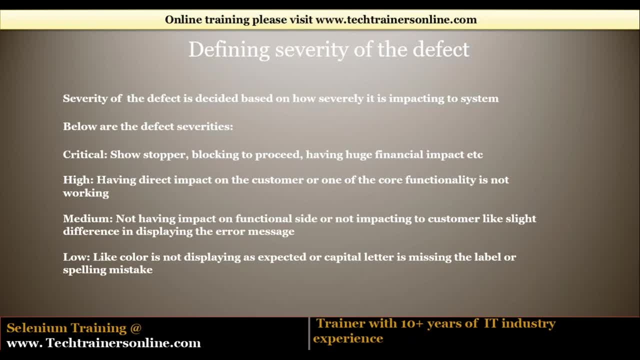 So what is the minimum thing is required Login. Can you do any testing without logging in? No, No, So most of the features in the Facebook like sharing the video, commenting, uncommenting, blocking, confirming the friend request. raising the friend request. 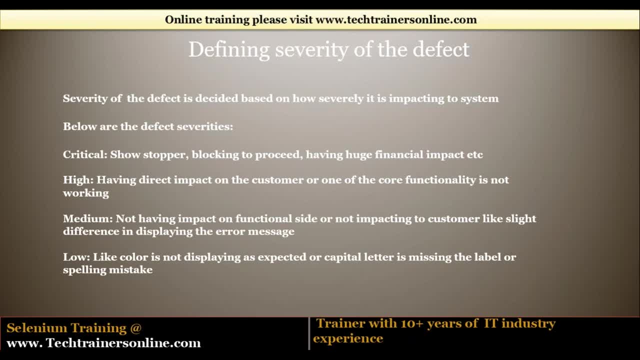 All these things comes only after you guys logging in. Now I have 20 testing team members who are working and all these 20 team members have been assigned with the different test cases. But for all of these testers, one common test case is: logging into the Facebook. 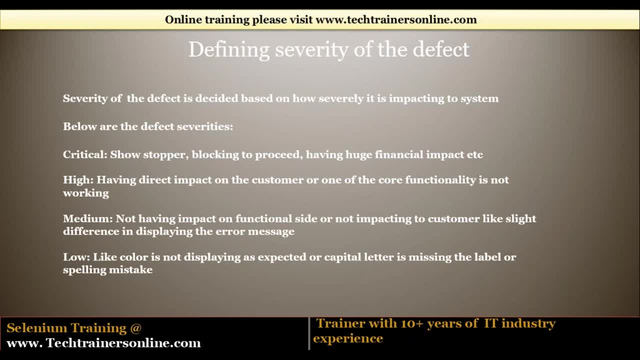 When I say logging into the Facebook, whatever the test cases that are being assigned, I have to log in first, irrespective of the test case. Someone might be publishing the video, someone has to test it with the commenting it. someone might need to block a friend, someone might need to add a friend request. 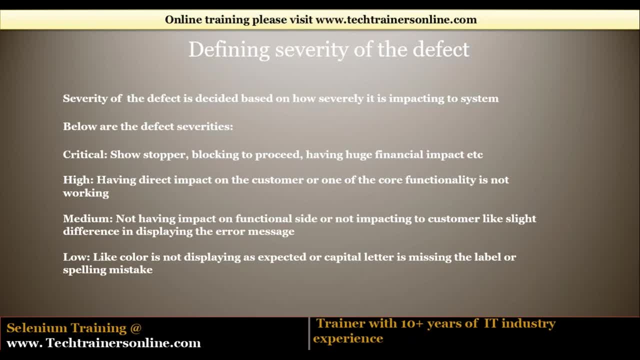 These are the different test cases, what they have. So, when they have all these test cases, the first thing is what they need to log in. Let's say that after entering the valid user ID and password, the system is not allowing the user to log in. 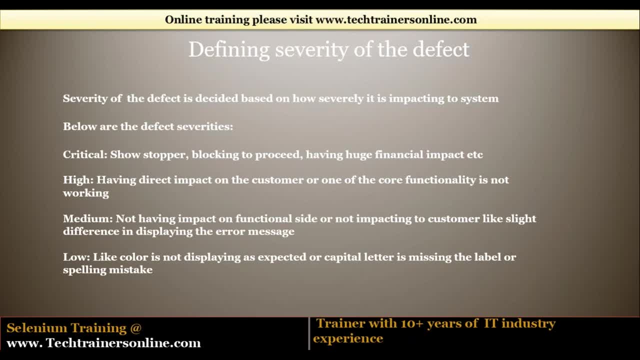 There is a defect, So do you think the Okay, All the 20 testers to raise 20 defects? It's one defect, So why do you think you need to raise 20 duplication of the defects? Are you guys getting what I'm saying? 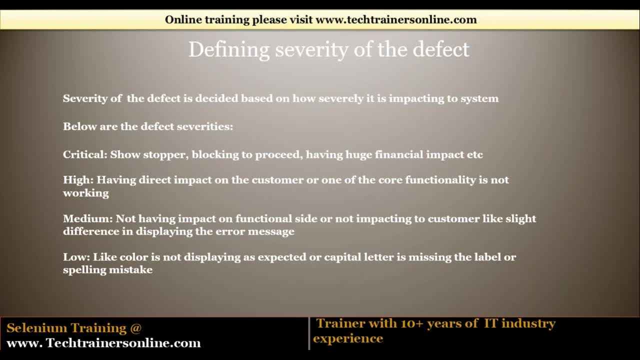 So we don't need to raise the 20 duplication of the defect. So any tester going to raise a defect, First we need to check that there is No duplication of the defect exists. We need to make sure there is no duplication of the defect. 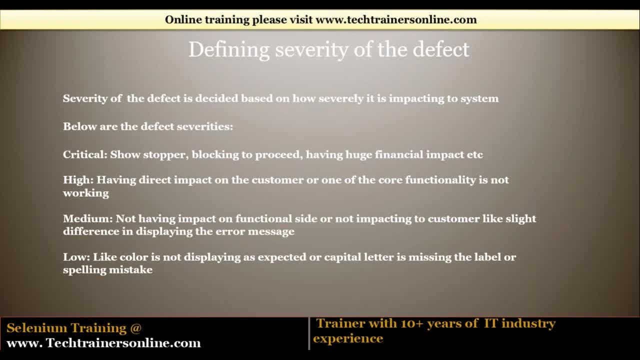 As an example, I don't want all 20 testers to raise the 20 defect. So then, how do I know whether duplicate defect exists or not? Every defect management tool will have an option for searching the defect. Right, You just go and search for the defect. 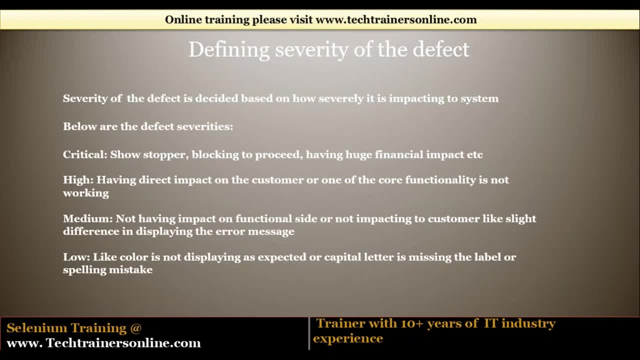 Now login is not working for me, Right? I just go and type in the search keyword as login paid or not allowing. I just go and type in the search keyword as login paid or not allowing to login, something like that. So, based on your search keyword that you have entered, it is going to take all the 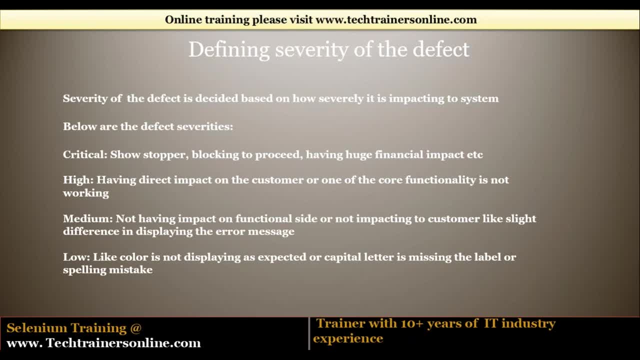 It's going to display all the relevant defects to it. You need to check which is relevant to it. If there is no defect exists, then go ahead and raise the defect. The first thing what tester has to look at is: is there any duplication of the defect? 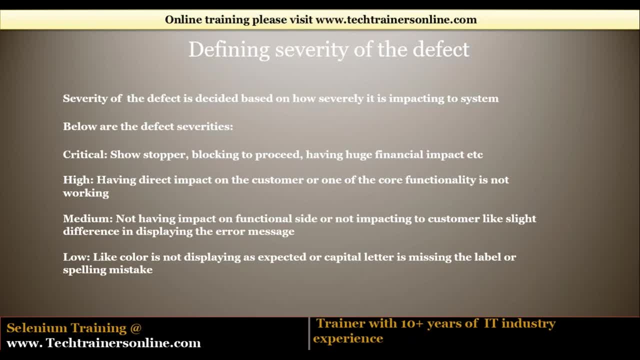 The first thing And the second thing, the make sure you attach the screenshots as much as possible. Now there is a spelling mistake in the error message, So it's a bug for me, It's a defect for me. So when you guys are raising that particular defect, you need to attach the screenshot. 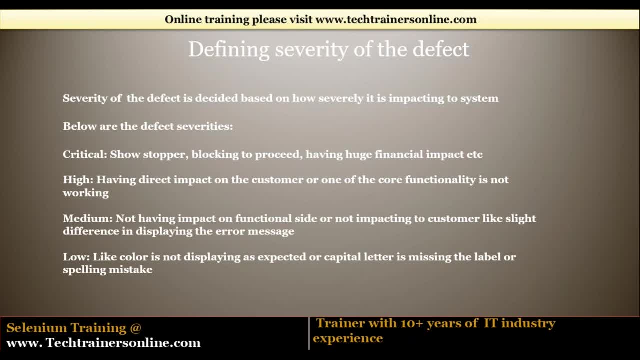 The developer need not to come to you and asking that. show me the error message on your system. So attach the screenshots as much as possible so that it is easier for the developer to understand. That's the one thing, And the second thing is: try to attach the videos also, if applicable. 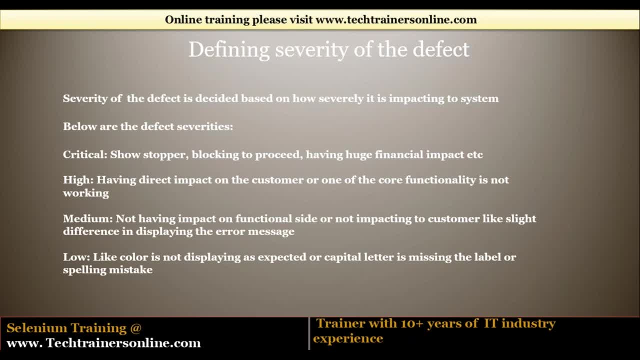 You guys can record the video when you are doing the testing. Upload that recorded video so that the developer who is looking at the particular defect it makes easier for understanding. I was working for one of the client who is a major bank in US and I was involved in doing 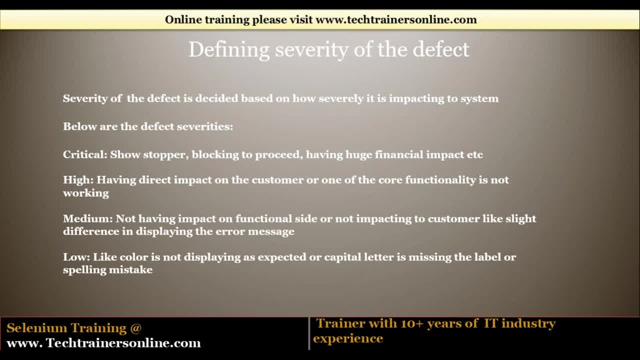 the ATM testing. You guys know ATM right, So insert a card, enter the wrong thing, blah, blah blah. There are so many test cases which are there. I was testing those test cases. I cannot capture the screenshot on ATM machine right. 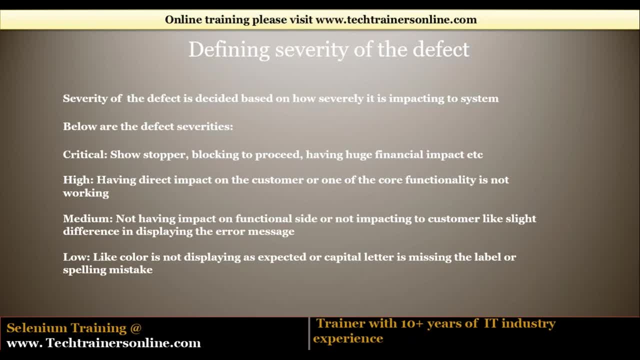 If I'm doing it in my system, I can click the print screen and take the screenshot and do it from there. But when it comes to something, example, like an ATM machine, where I cannot capture the screenshot, So go ahead and record the video. 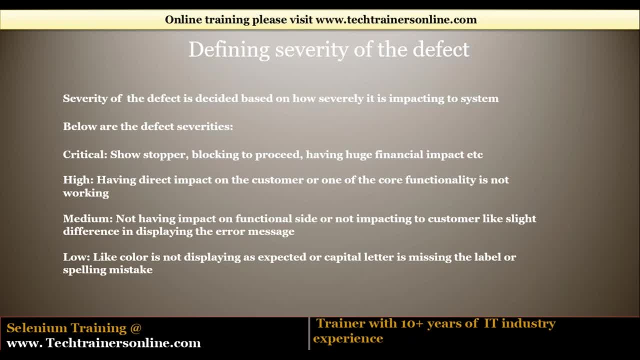 I was doing the recording video and place that recorded video in the defect. That's even allowed to do the video recording also, Okay. And when you guys are raising the defect, provide detailed steps as much as possible. So what I'm trying to say: provide detailed steps as much as possible and also provide. 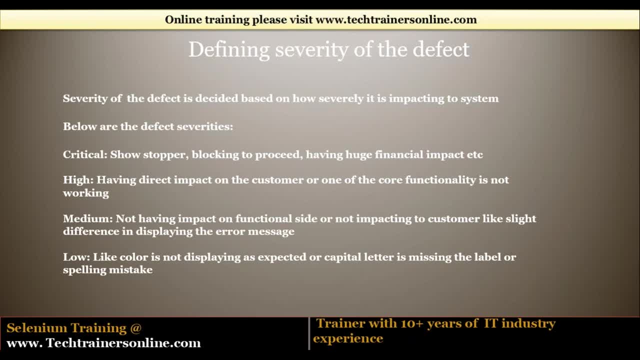 the test data that is used for raising the defect right Now. let's say that Darshi found a defect and she is going to raise a defect saying that even after entering the defect. Okay, Entering the valid user ID and password system is not allowing to log in. 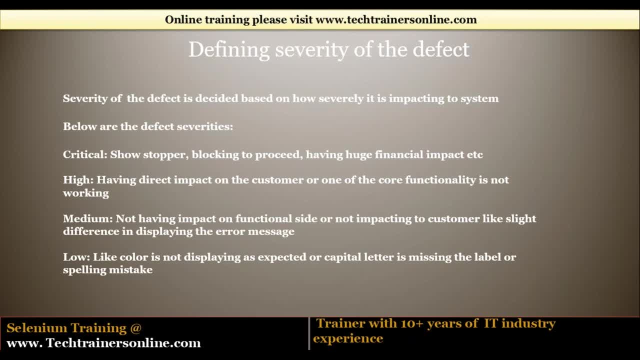 Let's say that you are working for a bag and you are entering the user ID and password. Both are correct. You are clicking on sign in. System is saying that please check your user ID and password. Enter correct user ID and our password. 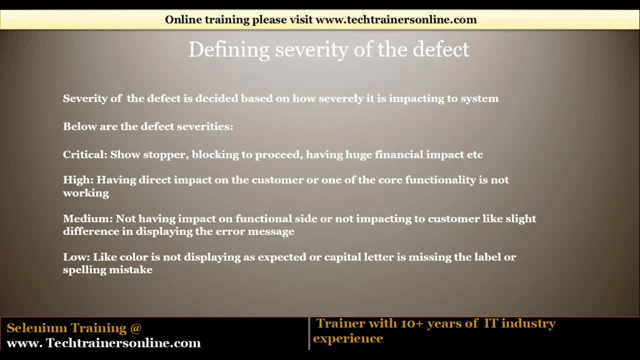 That's a message, what she is getting in, So she can go ahead and raise a defect. But what I'm saying is she need to capture the error message, what is getting in, attach it to the defect And then, Okay, Give the user ID and password that is used to logging into the system for which she is. 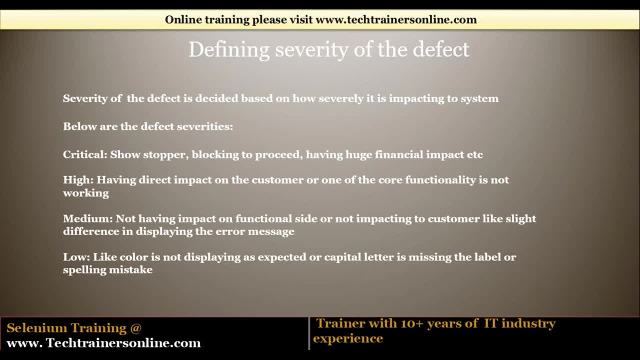 getting that error message. Why? I'm saying the test data. this is called as a test data. you should give the test data for which you got that particular defect. So when I say I got the defect for logging in, I need to give my user ID and password. 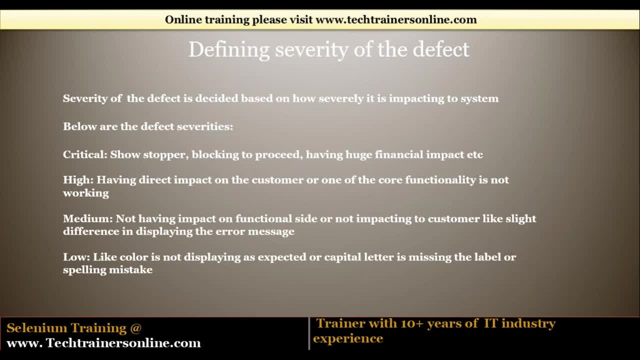 Now, if the Darshi is giving the user ID and password in the defect- what she used, for which she is getting a defect, Then you assign the defect to the developer When the developer investigate. developer tries to replicate the defect. Developer tries to log in with his credential system is allowing to log in. 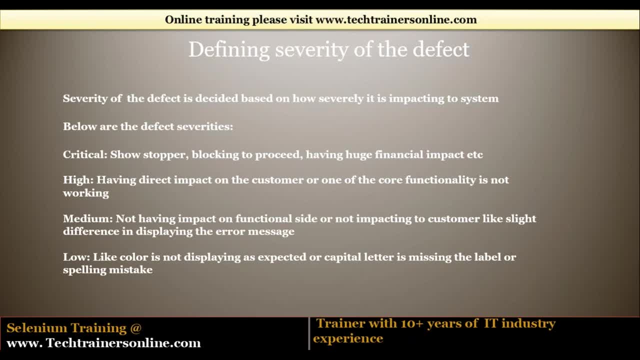 Then what is the problem? Is the problem with the system or is the problem with the test data here? What is the problem, guys? Developer is able to logging into net banking, but Darshi is not able to logging in. Is the problem with the test data or the problem with the system? 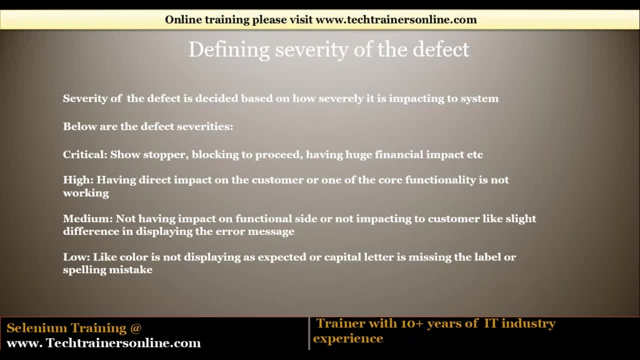 Problem with the system. Problem with the system, but I am able to log in with my user credentials. but you are not able to log in. Which means Now let me give you another example. I'm going to ATM machine, I'm inserting my ATM card and I'm getting money, whatever I'm entering for withdrawal. 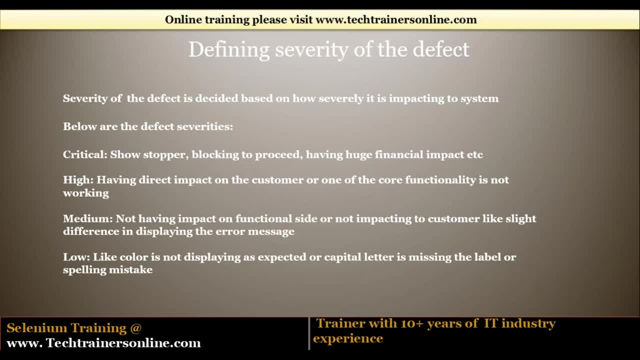 Now, Darshi, you go to the ATM machine next to me and you insert your card. It says your card is invalid. Is the problem with the machine or the problem with the card? For me it worked. For you, it is saying no. 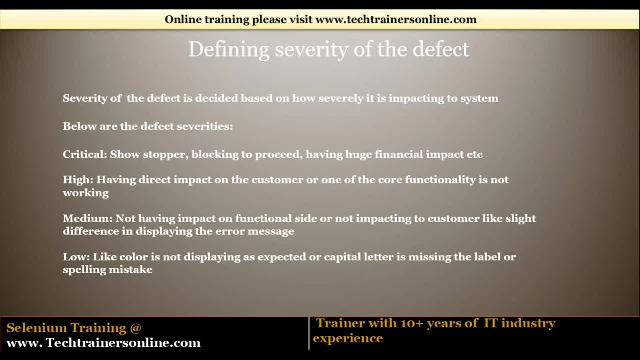 System is saying your card is not valid, Then there is a problem with your ATM card, which is not with the system because it is allowing to log in right. It's not a problem with the system. So that's why I'm mentioning you need to provide the test data. 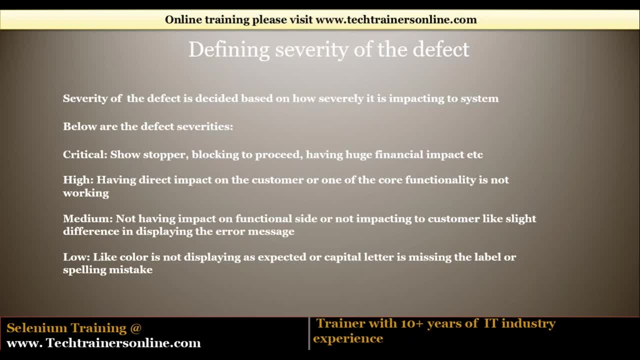 So why I'm saying you have to give the user ID and The most important is that your account was logged in and you did not enter in your password. you did not enter in your cell phone number and password. The developer logs in into the system, is able to log it into everything. 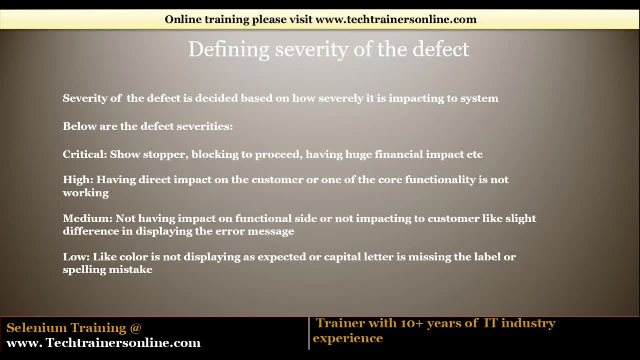 but with the user ID that you have given in that effect, they are not able to log in. when they went and checked it in the database, Your account is logged. Assume that you are someone who tried your user ID and type wrong password more than three times, which you are not aware about it. 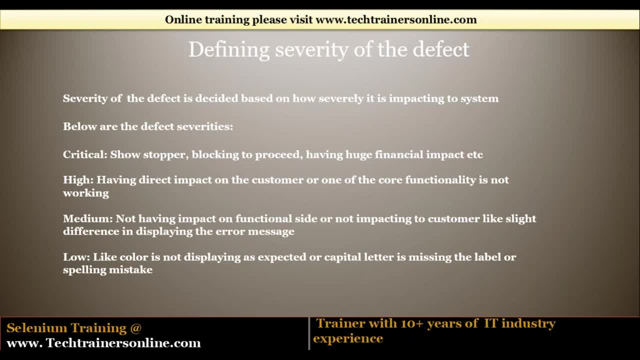 Then You keep entering is locked. what developer can say? developer can reject your defect, stating that the system is working as expected. I am able to log in. the user ID that you use to login is being logged in the backend because of invalid, wrong passwords that are entered more than three times. so do you think it's a? 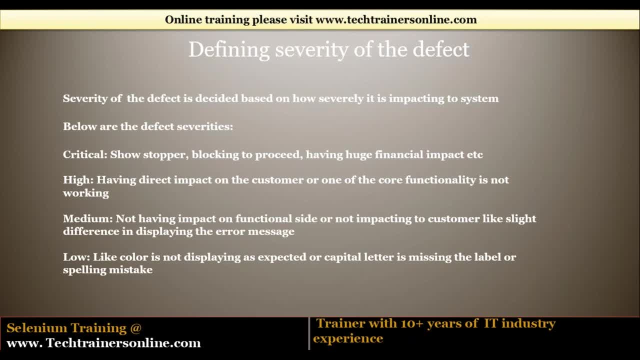 defect or it's a problem with the test data that tester is used. it's a test data problem which is used by the tester. so that's why I am trying to mention you always include your test data for which you got a defect. maybe something wrong with my test data, I don't know. so put the test data so that it makes easier. 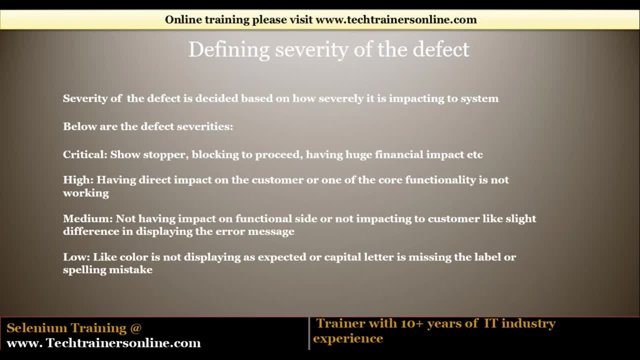 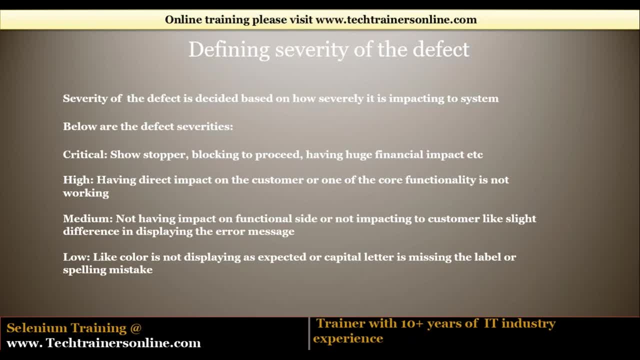 what needs to be considered before raising the defect is: first thing is check if there is a duplication defect. if the defect already exists, do not raise it. if no defect exists, raise it. check for the duplication of the defect. second thing is attach the screenshots as much as possible. you know for better. 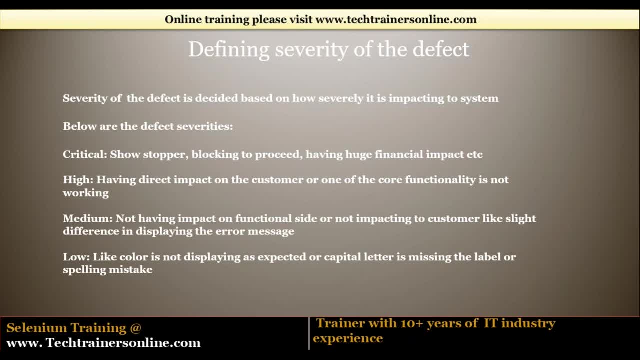 understanding. if applicable, attach the videos also, if it is permitted, before uploading, before recording and doing this stuff, check with your supervisor. don't do it directly. it could be into policy violation. you are not supposed to record client system or something we don't know, so don't take that talk to. 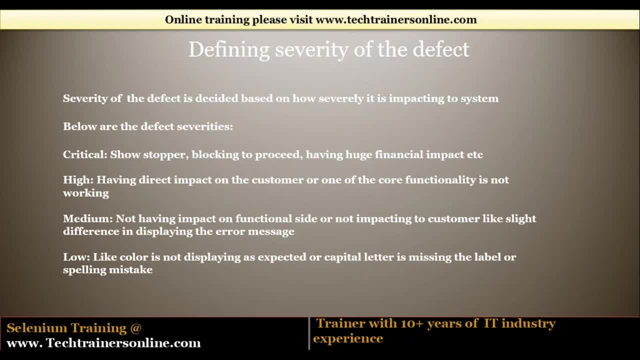 your this supervisor is recording. videos can be uploaded and then provide detailed steps to reproduce. I need to provide what are the steps I have to follow in order to reproduce the defect, so that the developer can reproduce the defect, and another thing is provide the test data that is used while raising the. 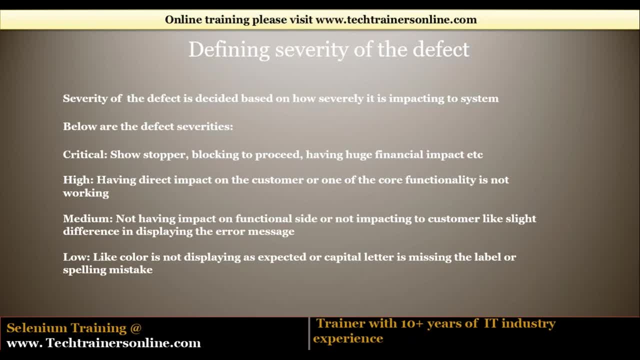 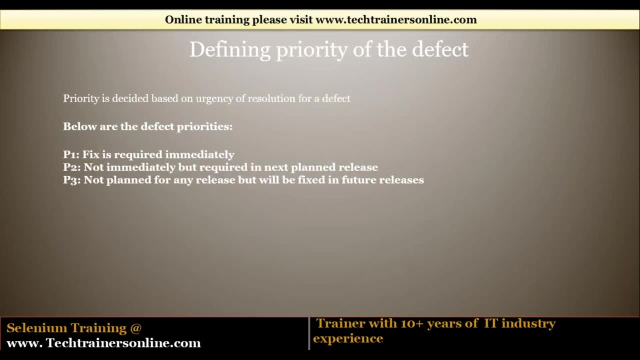 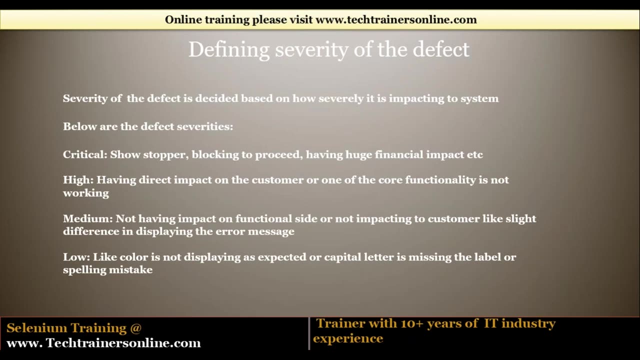 while getting the particular defect. so these are the things that you guys have to consider before raising the defect. you also need to consider the severity and priority of the defect, not any. we are going to talk about it, okay. so let's understand the severity of the defect. so we said in the test plan: what did we say? 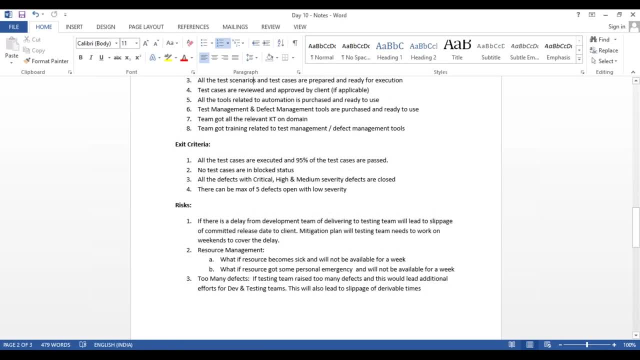 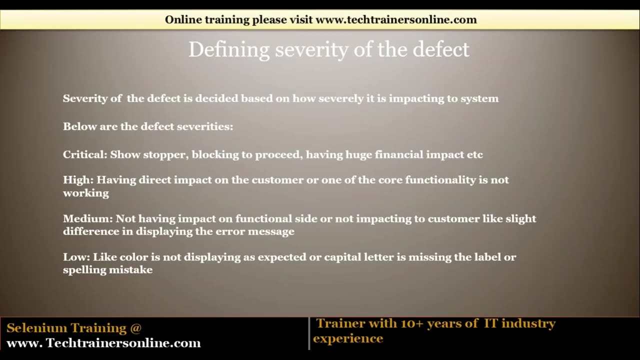 in the test plan, in the exit criteria we said defects with critical high medium severity. now we are trying to understand what do you mean by the severity here, right? so severity means severity of the defect is decided based on how severely it is impacting to the system. so we need to understand: if I found a defect, how? 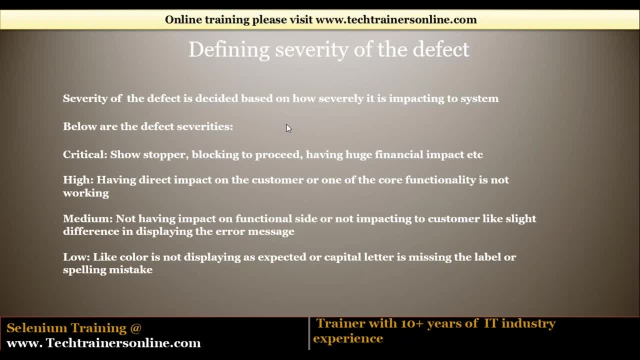 severely it is impacting to my business. so, based on how it is impacting to the business, you need to decide the severity most of the defect management tools have. common severity is called critical- high, medium and low. so I'm also defining what do you mean by a critical? 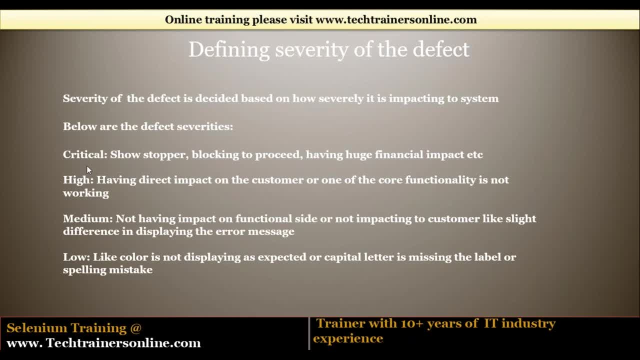 I am also defining what do you mean by a critical critical means. if the defect is so stopper, it's completely blocking to proceed, having huge financial impact. so if I see any of these things now, I'm trying to understand the severity of the defect and then the backlog again, including the severity of the defect. 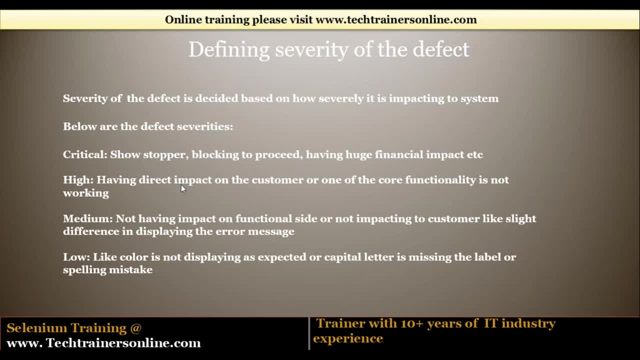 so you are saying your area, you are deciding whether you want to stopper it or stopper it. yes, so the severity of the defect is out to the left and in the right gut. it's a little bit depending on how many people are there and how many. 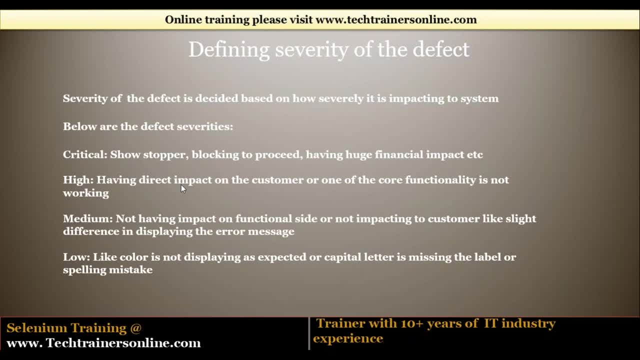 or how many people are in the right cell. it depends on how many people are there and how many people are in the left cell and what are the stages of that. we need to responding to your facebookcom. so do you think it's a critical defect or low defect or medium? 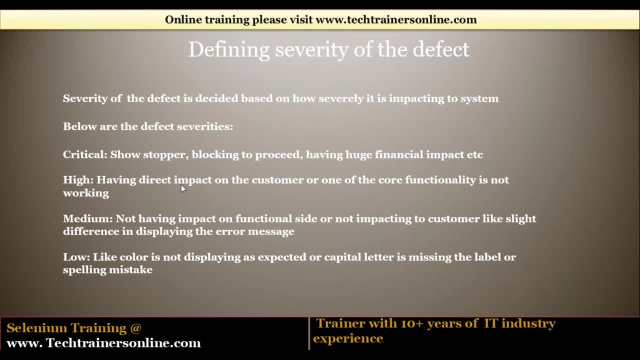 it's a critical for me is it: is it, is it blocking or not? it's. it's blocking entire testing team to proceed, right? do you think you can proceed to do testing without launching the application? no, it's a critical severity because it's a source stopper. it's completely a stopper. 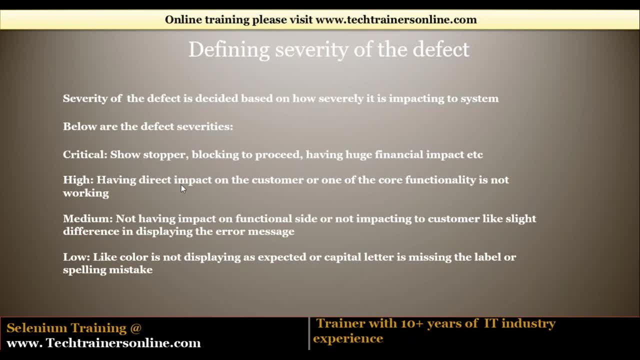 for entire team. it's a completely stopper for the end user also. they cannot use it right. and also, if you see there is a huge financial impact, now you're transferring funds of one thousand, it is transferring thousand rupees, but it is crediting you know it is debiting one. 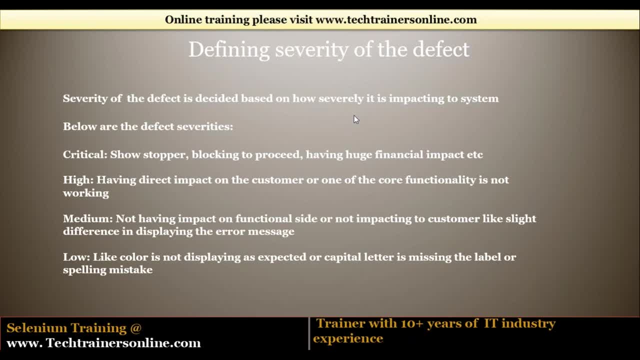 lakh rupees from you. let's say that. uh then, so you are transferring thousand rupees to me and i got thousand rupees only, but when it comes to your account, it is deducted one lakh rupees from your account. it is what it is doing. additionally, it is adding two more zeros. 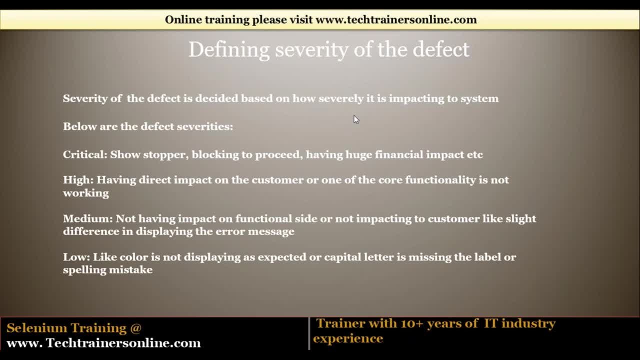 in the end. is that correct? so it's going to be. it's going to be a critical defect again because it is hugely impact on the financial system. do you think you will be happy if it is deducted one lakh rupees from your account instead of thousand? no, 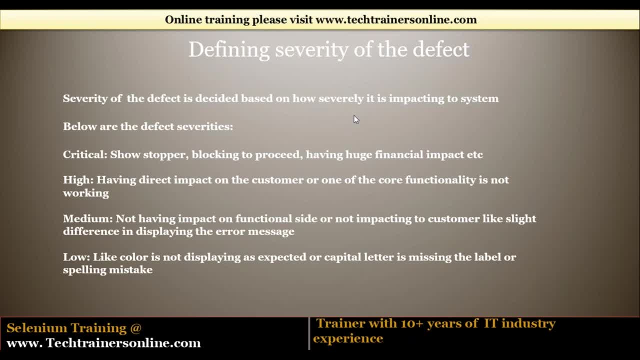 it's a huge finance loss to the customer. right customer will definitely go upset. then they have to call to the customer care and customer care guy has to investigate and then refund 99 000 rupees back to your your account. so as long as you see defect is severely. 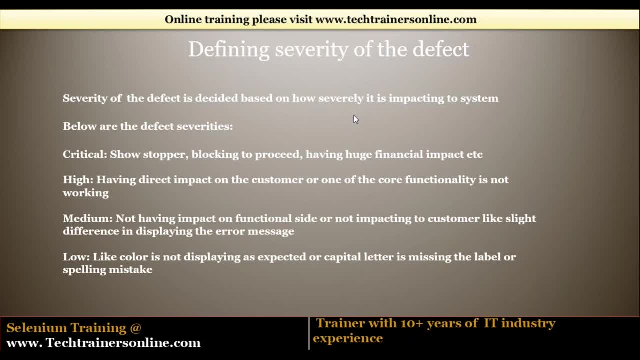 impacting like show stopper or a blocker or having huge financial impact. you go and select the create defect as a critical. so every defect management tool will have a drop down or a pick list. it's loaded with the values for called criticals- high, medium and low. so what is? 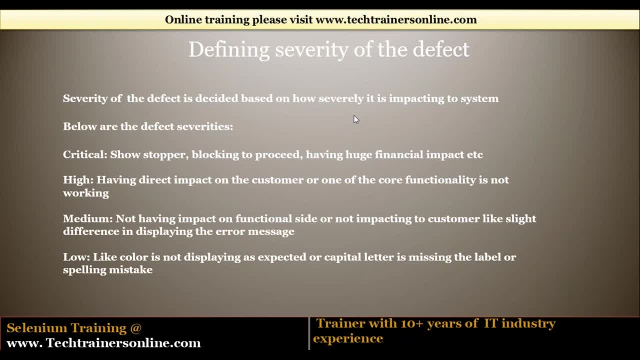 happening here. when you create, click on create new defect. anyhow, in tomorrow's session we will try to discuss defect management tool. i can show you what i'm talking. when you click on create new debate, it ask you to select the severity. so it's a drop down in which you guys see all these values are loaded. 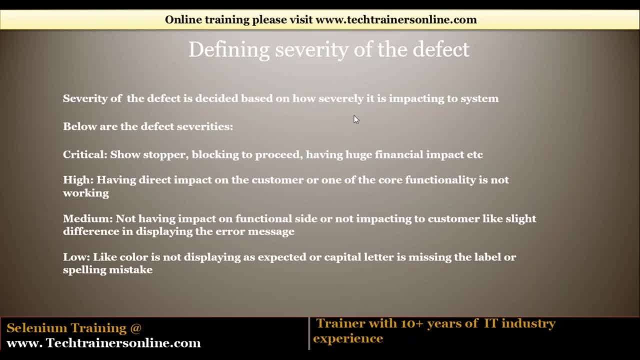 so you need to select the severity based on the defect, what it is severely impacting. okay, so if you see whatever is defined here, right, if you see whatever is defined under critical, you guys can go ahead and mark them as a critical defect. now, what is high severity having direct? 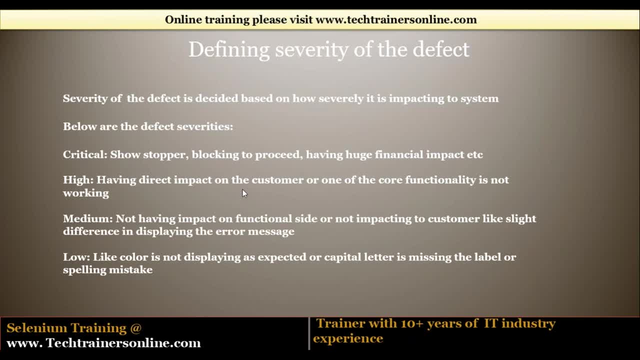 impact on the customer or one of the core functionality is not working. so we discuss the types of test cases right: gui, functional and field level validation. any test case that is marked as a functional test case is not working means i can straight away raise the defect as a high defect. 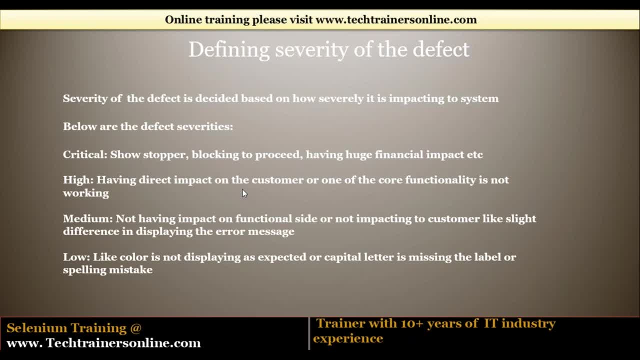 severity as a high, which means like, say, adding the beneficiary is one of the functionality you are not able to add because some defect. so in that case you go ahead and select the defect as a high severity. now i clicked on transfer funds. nothing is happening, so means it's a functionality itself is not working. 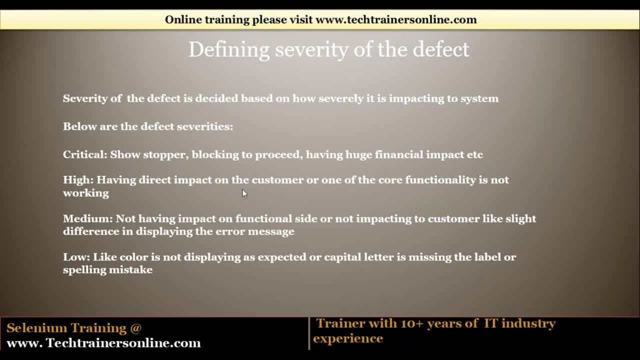 one of the core feature of the system itself is not working, then you can create that particular defect as a high severity defect, okay. and the next one is the medium not having impact on the functional side or not impacting to the customer. error like slight difference in displaying the error message. so the 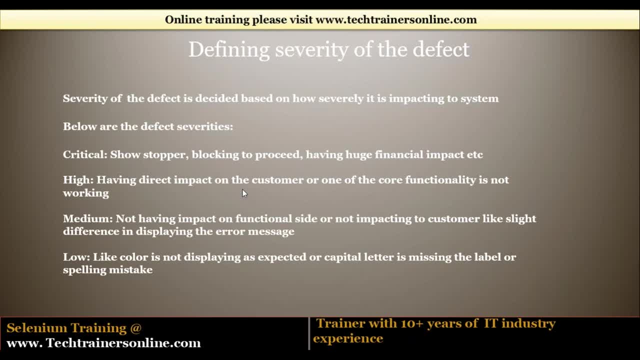 defect that doesn't fall under critical and high generally comes as a. so there is a spelling mistake, then i would go ahead and raise the defect. it spelling mistake will not come as a medium, it will come as a low it so media means the client requested to display an error message if user enters a wrong password. 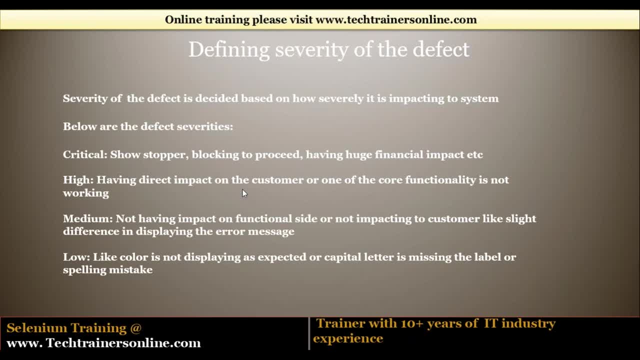 more than three times. they wanted to display if you enter wrong password more than three times. so if i confirm, enter to untransprit. if i encrypt the wrong password more than three times, they wanted to display if you enter advancedผ las farals in the cloud and ein car sc ice as an alternative error message. 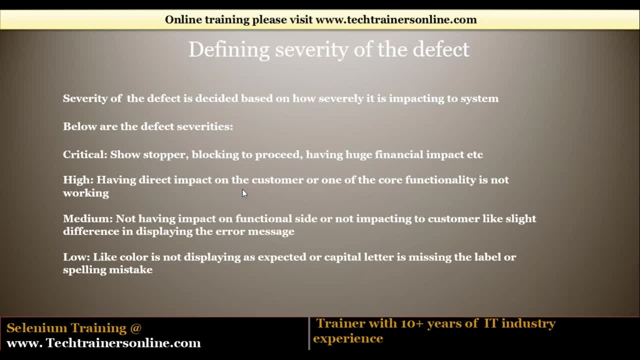 error height: very small error high: error: Install the error error message. if user enters the wrong passworde forty or five times, more than three times. they wanted to display too much error. jailKeeper should assess if the problem ends. the software is accurate. your account will be locked. that's a client asked, but what developer has? 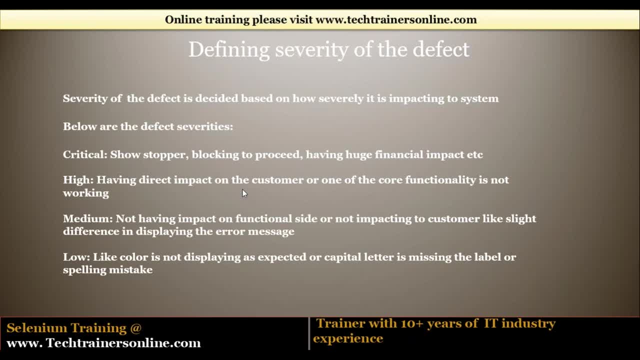 implemented. your account will be locked if you enter wrong password more than five times. so what is being asked three times? what is being displayed five times? it's misleading and, you know, misguiding to the client. right account is still getting logged after three wrong passwords. only functionality is working. 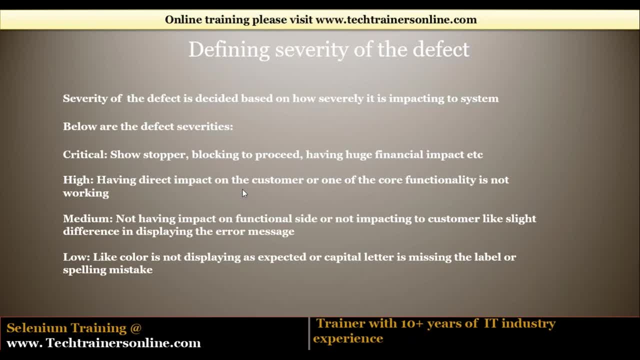 but the error message is: instead of three, they are displaying it as a fine file. right, I can consider that as a. I can consider that as a medium defect. it is working fine. functionality is working fine. what is the functionality? account should be locked after three wrong password. it is locking, but the message. 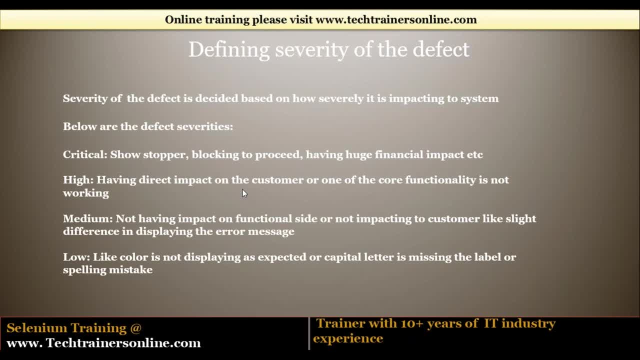 what it is displaying is, instead of three, they are displaying it as a fight, which is misleading. I can consider that defect as a medium. and the last severity is low, like color is not displaying as expected. our capital letter is missing. capital letter is missing. the label are spelling. 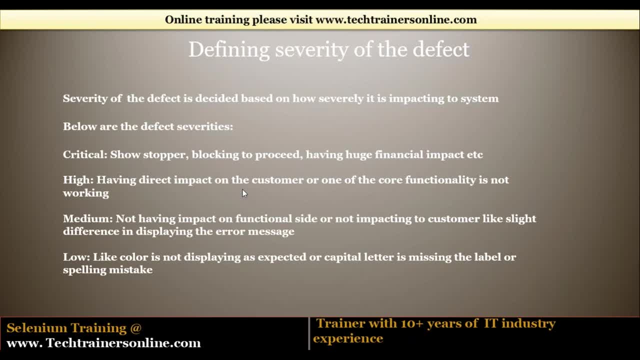 mistake. so anything relevant to alignment, spelling mistakes, color issues, all these minor things would come under the low severity. so I repeat again: all the defect management tools will have severity and priority. you have to select that particular value from the drop-down when you guys are raising the defect and 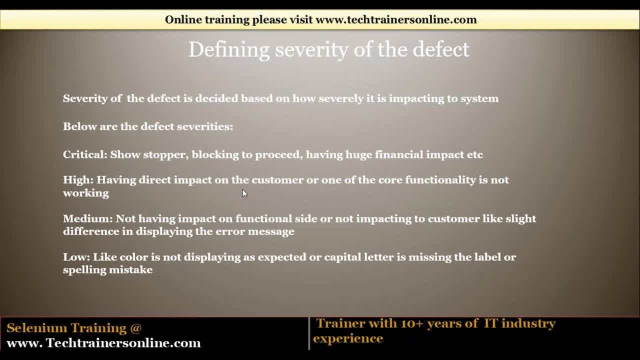 some tools will have other than this, what I have selected, and you can see that this value is higher than this, what I am talking about. some tools will have only these four severe it is. some will have more than this. so that's what exactly? the difference between one tool to another tool. any questions on severity? 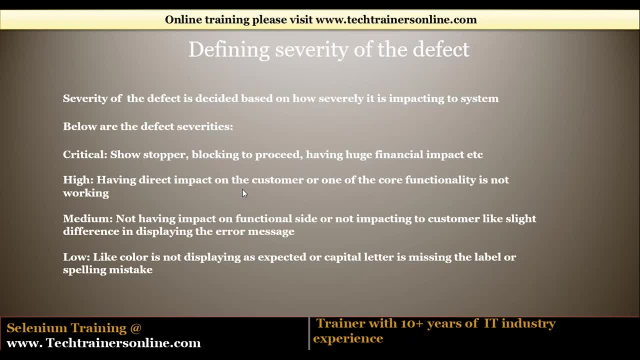 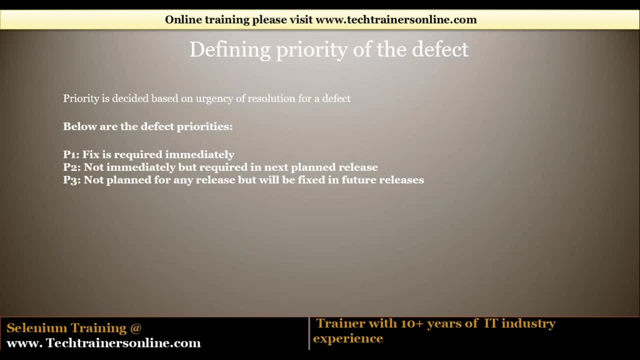 of the defect. okay, let's move on for understanding the priority of the defect. so priority means based on urgency of resolution for a defect. Now let's say the testing team has 20 defects. Do you think all 20 defects should be fixed immediately? 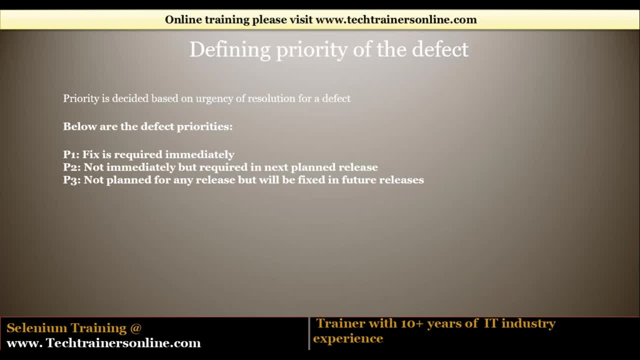 Priority is going to define me which defect to be fixed first right. So priority means the defect that needs to be fixed in urgency basis. So like we have P1, P2,, P3, and P4.. P1 is nothing but priority one. 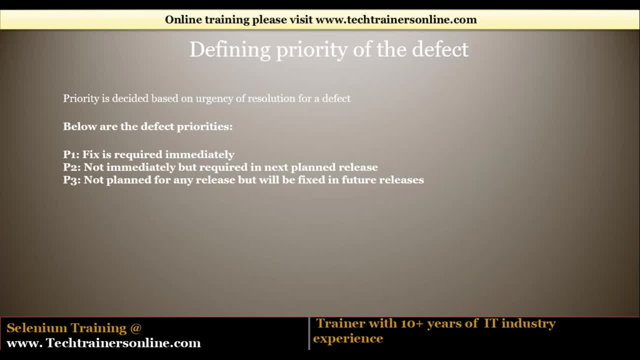 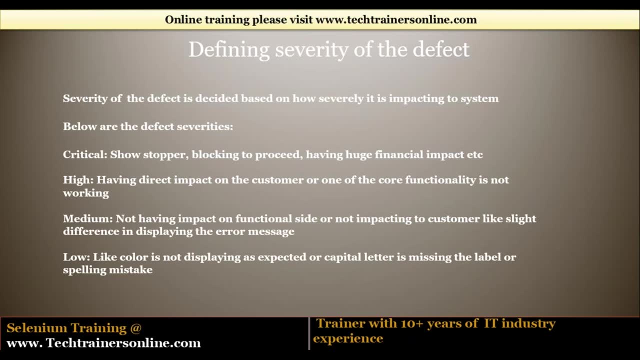 Priority two, priority three and priority four. Some tools will have the same priority and severity and priority will be the same. Now we are talking critical, high, medium and low. Priority also can be have same: critical or medium, high and low right. 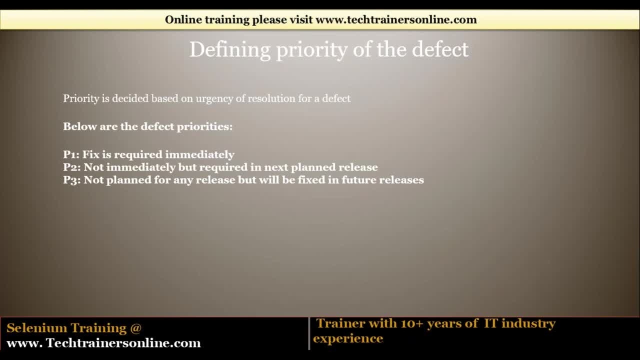 It differs tool to tool, but most of the tools will have P1,, P2,, P3, and P4.. So when I say I have to raise a defect as a, when I say I have to raise a defect as priority one, 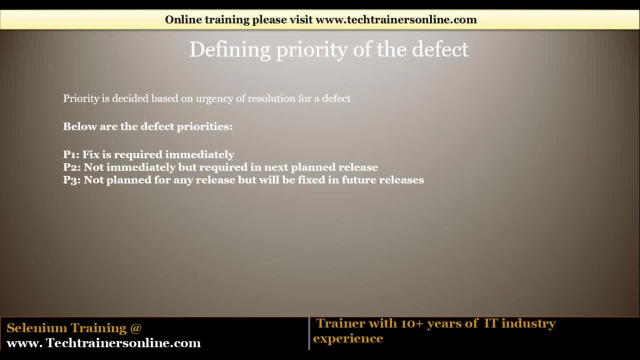 which means it has to be fixed immediately. I'm also giving the definitions of P1, P2, P3.. What do you mean by P1?? Fix is required immediately. If I'm selecting, this is again drop down. You have, it will be loaded with the values. 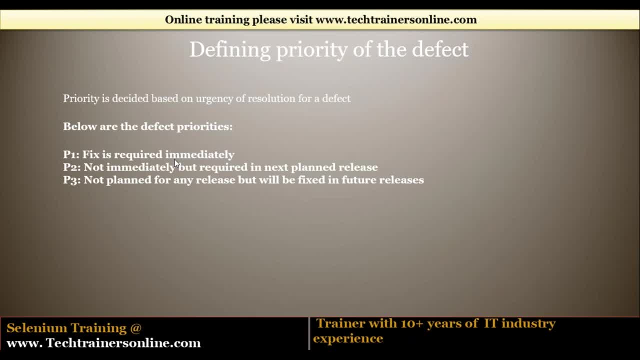 It's again drop down. It has to be loaded with the values, So you have to select the specific priority based on your defect. So if I'm choosing the P1, it has to be fixed immediately. What do you mean by fixed? 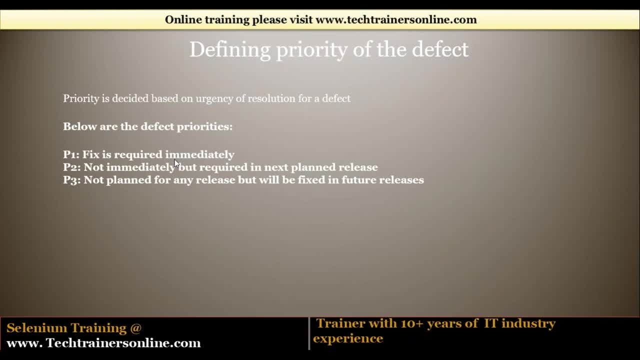 Required immediately. Do you think that I have to fix in two minutes of time? No, So if you guys remember, if you guys are aware about SLS, do you guys know what do you mean by SLA? I think maybe Anquish you might aware. 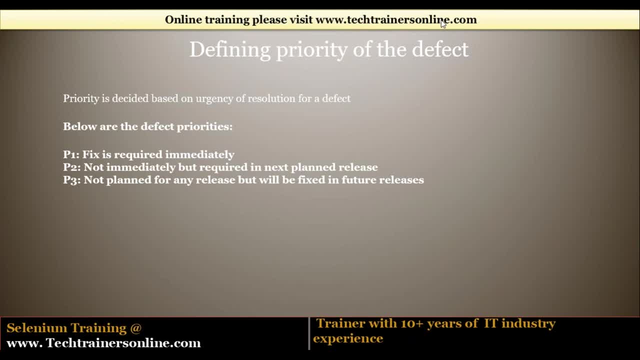 Do you know what is SLA? Yes, sir, The time you want to complete the task. Yeah, service level agreement, what we talk about. So we are going to have an agreement with the client which we call it as SLS- service level agreement. 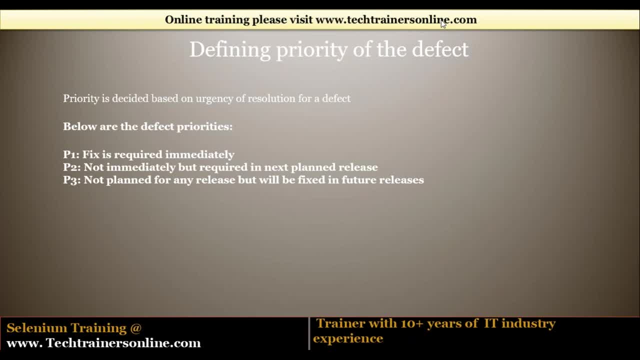 If someone is raising a P1 defect, what is the timeline by which we have to fix it, If a critical and a P1 defect is coming from the production, So what is the SLA to be fixed in? SLA means what is the timeline that you have to fix it. 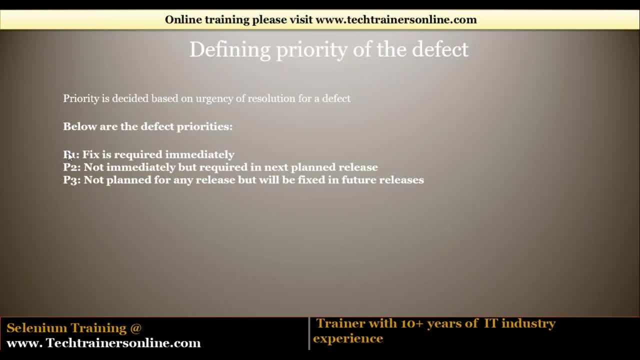 So if I say P1, most of the time SLA for the P1 would be is, like you know, SLA for P1 would be 24 to 48 hours. Yeah words, any defect that is coming as priority one should be fixed within 24 to 48 hours. 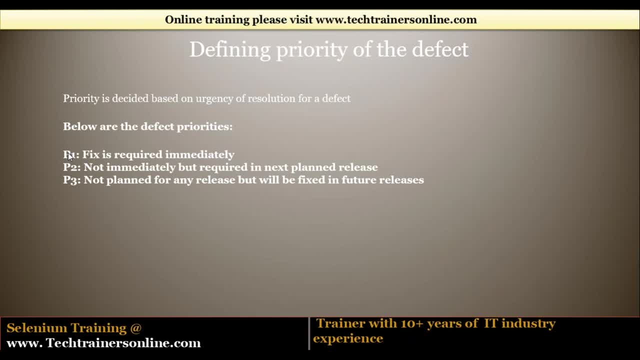 it generally differs to client to client. again, i don't say 24 hours or 48 hours, so that's how you guys are going to agree with your, your client. so you have to define your slas with the client and then you need to proceed according to that. so when i say p1 is red, it. 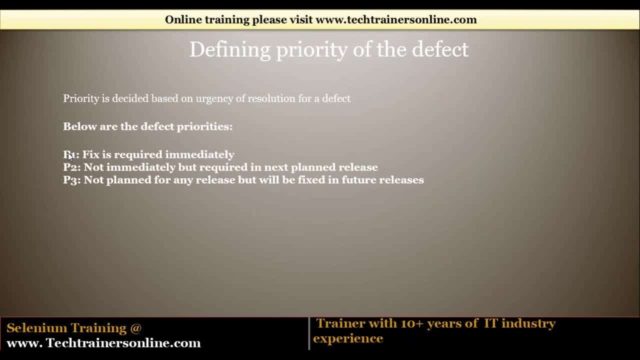 doesn't mean you have to fix it right away. even developer needs some time to undo the analysis: why it is happening, debug it, understand it and fix it. even tester also needs to retest the defect. it's time, it takes time right, so you can't ask: fix it immediately. 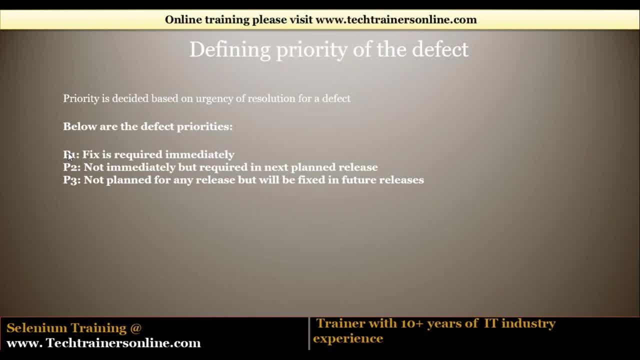 so p1 fix- required immediately. it doesn't mean immediately. it takes generally 24 to 48 hours of time. what we have agreed sls with the client p2- not immediately but required in the next planned release. now i am raising a different call: p2. it doesn't mean i have to fix it immediately, not even in the current release. 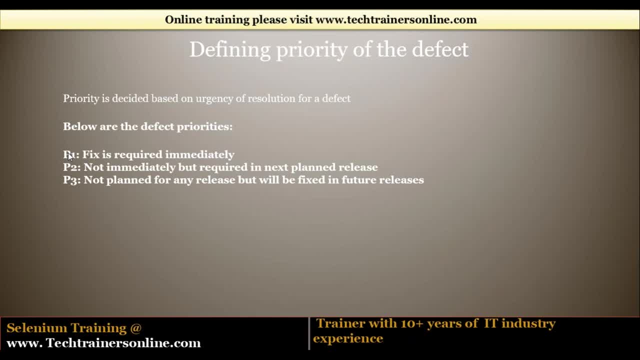 i can consider it in the next release that is coming in after 15 days or after a month. i can keep that defect open, concentrate on working or fixing of the priority one defects which is the first priority for me. once i am done, fixing of all p1 defects. 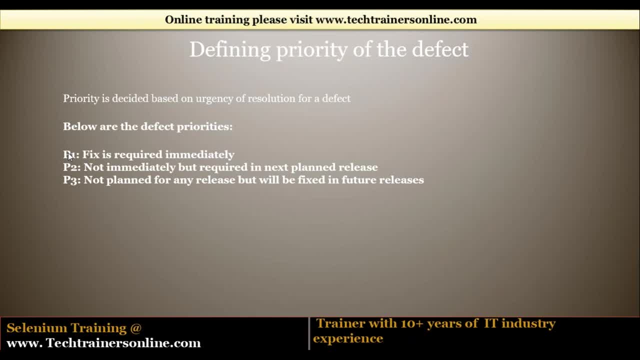 i would go for the p2 defects right, and then p3 and p4. normally uh, not planned for any release but will be fixed in future releases. any defects p3p4 priorities may not require to fix in the current release but it will be considered to be fixed after p1. p2 defects are being fixed. these are: 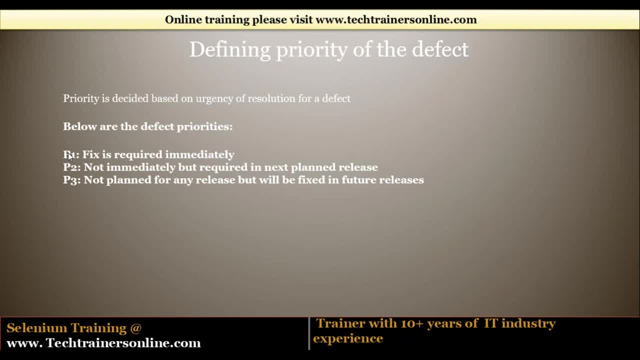 the priorities. any questions? yes, sir, uh, can you see that the defel due to which the tester is blocked, that comes under p1. madeleines d students: fin� sim um, um, um you d sim, um, sorry, and so the defect due to which the tester is blow, that should come under p1. 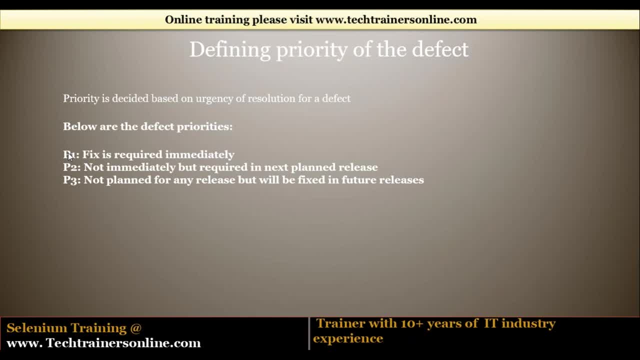 right, yeah, yeah, that is why I'm doing the test. okay, but any defect that is coming in the production? let's say that you are using your ATM card. even after entering the valid user ID and password, ATM has taken your card inside. that's a p1 also coming, because the customer is not allowed to do any transaction and 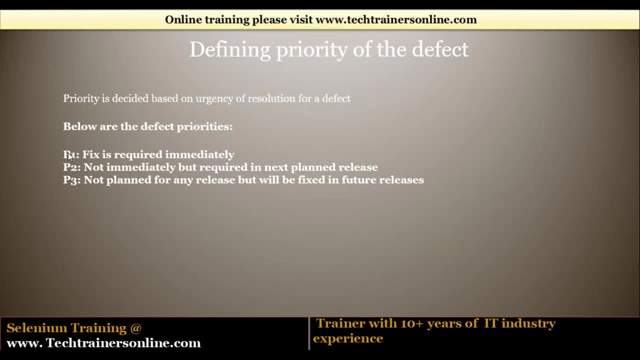 also customers card is taken inside the ATM machine, it's obviously p1 should be fixed immediately. that is coming from the production. it doesn't matter from where defect is coming in, but you need to understand the urgency of the fix. if it has to be fixed urgently, then choose the p1. 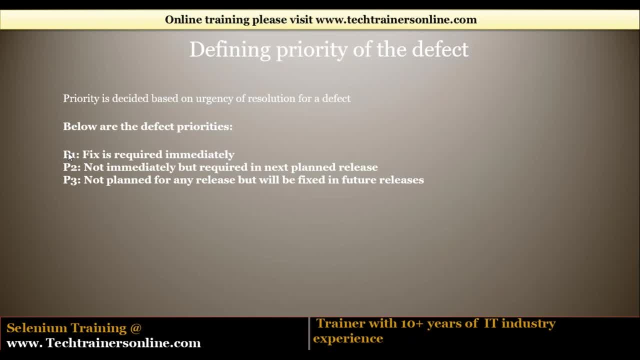 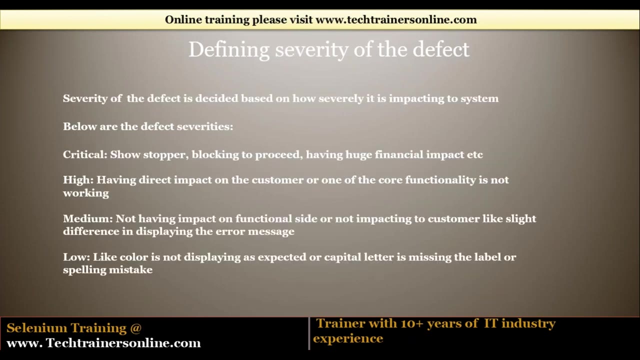 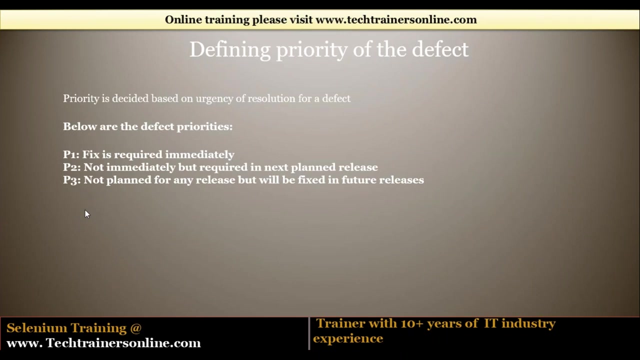 okay, now I want you guys to you know, do the analysis that you know can I have? I'm just giving it. as for you guys to think about it, can I have critical severity equal to critical and priority equal to p3? I'm saying it's a critical defect for 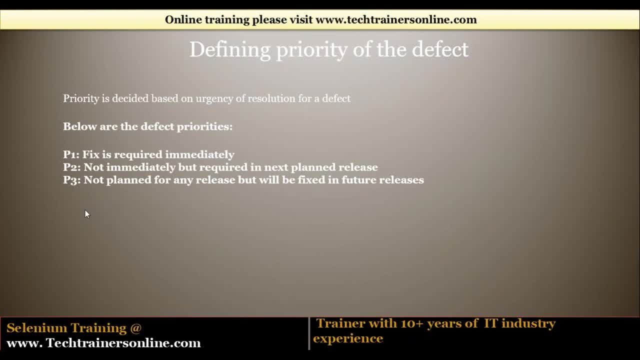 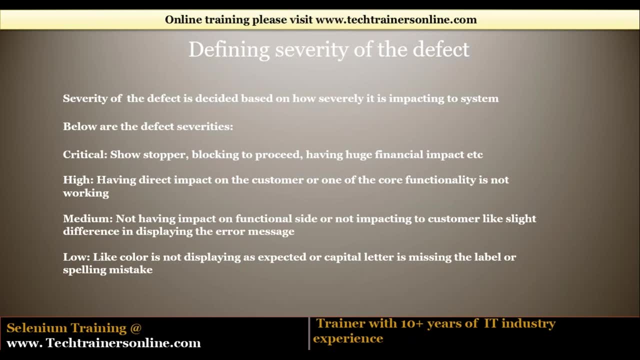 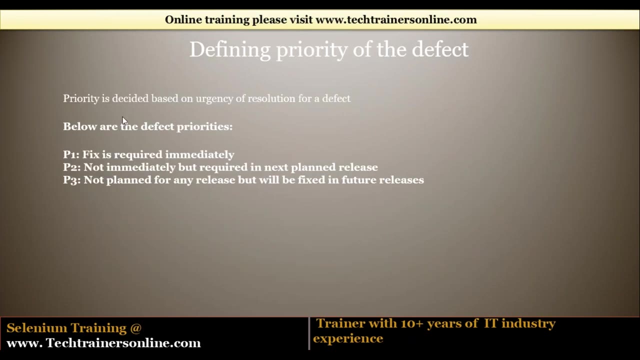 me. but I am saying p3, don't fix now, we will see it in future. can we have some scenarios like that? that's one thing. and second thing: I am saying severity equal to low. okay, I'm saying severity equal to low and I'm saying it's a p1 defect for me, fix it. 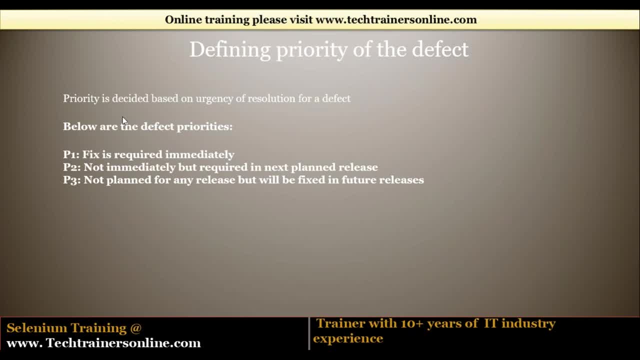 immediately. managing is not going opposite direction. I'm saying severity is low but critical of p1. I am saying reality. I'm saying Buwan, fix it immediately. do you think it could happen? you think about it and let me know in the comments section. don't be confused on my specific questions. 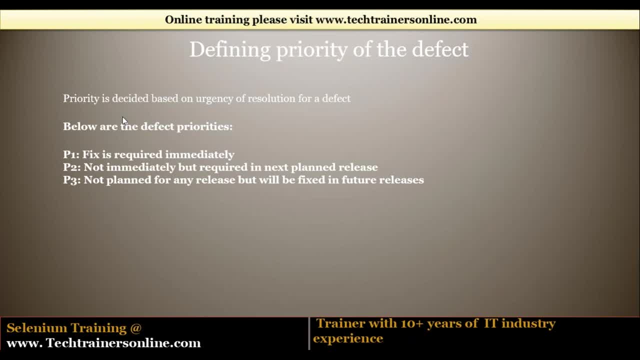 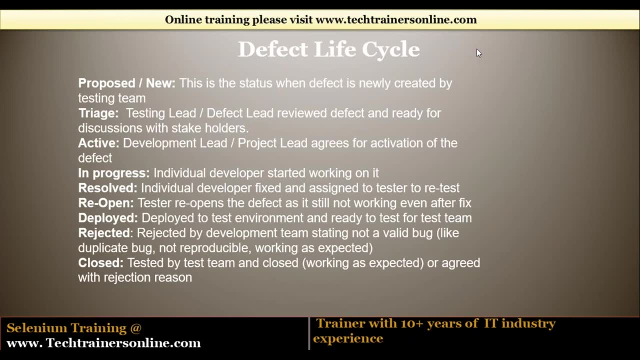 just let me know it really long as always, and thanks for watching. ref liegen jetzt dabei belli in tomorrow's session. okay, so let's try to understand the defect life cycle. so what do you mean by the defect life cycle? so every defect management tool has the different statuses. 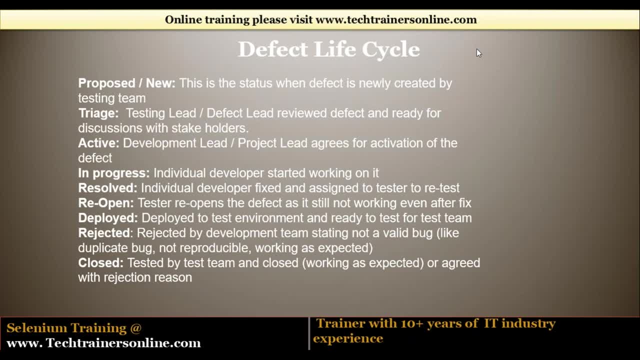 different statuses is nothing. but you know, once you raise a defect, what is the status of the defect then, how it moves on. now, whenever you guys raise a defect, typically it will be in the proposed. it will be in the proposed slash new. so whenever you guys raise a defect, it would be in the proposed status some. 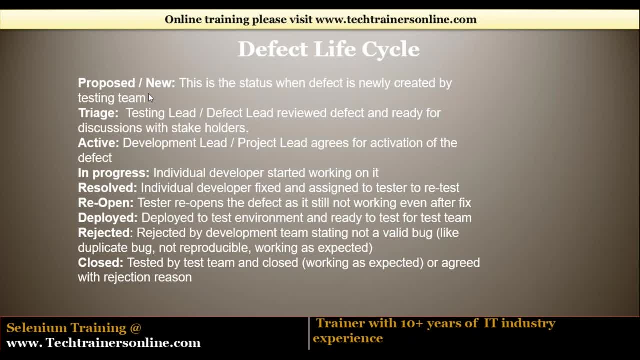 tools will have status as proposed and some tools will have the status as new, right. so what do you mean by a new or proposed? because this is the status when defect is newly created by the testing team. like, say, you found a defect, you raise a defect, the status of the defect would be new. 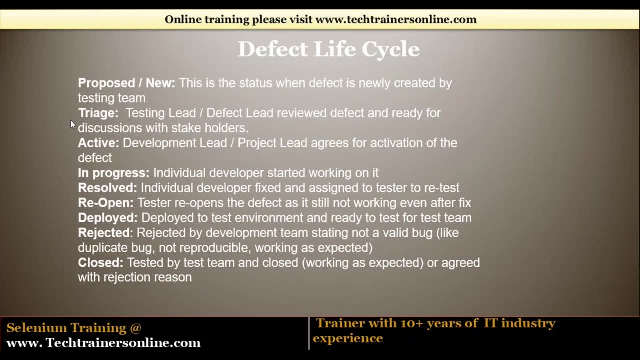 then the defect status will be changed to triage. now, once you guys raise a defect, to whom you have to assign? you need to assign it to a developer or assign it to your test lead. again, it differs to the project to project if it is very small team. 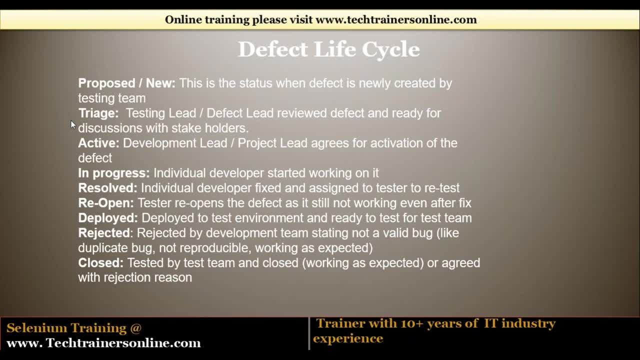 okay, if it is very small team, you guys can go ahead and assign it directly to the developer. if it is a big team, there is a separate role called defect lead or defect manager role, and you know that would be that would be given to defect lead. once you guys found a defect, raise it. 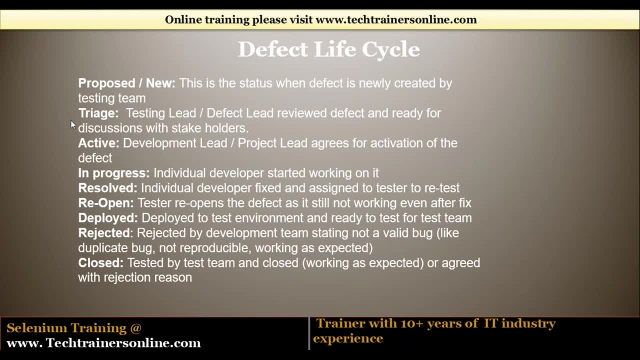 and then assign that defect. your supervisor r to your test lead and your test lead looks at the defect and your test lead finds all correct and this is valid defect. then your test lead is going to change the status of the defect as triage, which means that team leader defect lead. 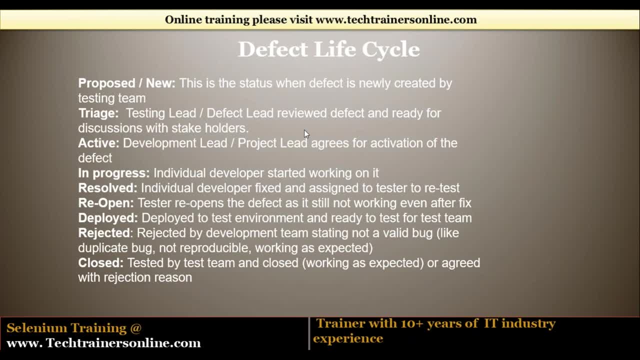 reviewed your defect and ready for discussions with the stakeholders. so if i have a 20 members testing team once defect is raised i would not directly take it to the developer to discuss. i will schedule a call, which we generally call it as a trash meeting, so where i generally call. 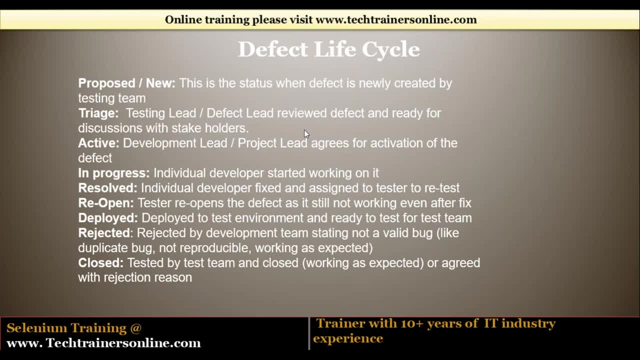 it as a trash meeting where we have, um, you know, once in a week or twice in a week. so i will connect with you guys on that. so once you get my details, you can see what i got and what i got from that. so now i will. 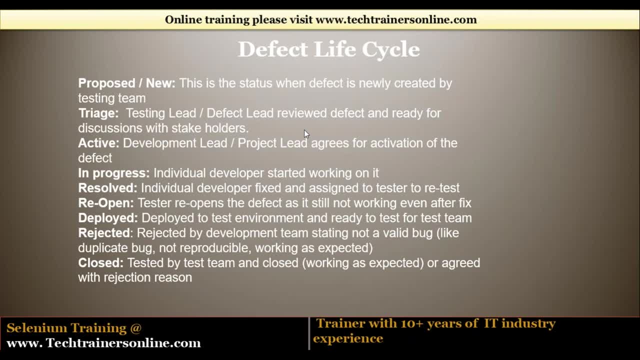 you know, once in a week or twice in a week. so i will connect with you guys on that. so i will connect, Consolidate all the defects that are raised by the testing team and make a meeting called triage. In that meeting, discuss all the defects which are in the status called triage, which means the defects are really ready and it can be discussed with the stakeholders. nothing but the development team. 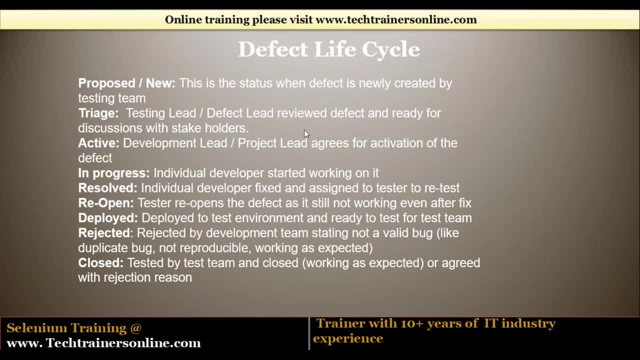 In this defect triage meeting, client is also going to be involved And if the developer and tester is arguing- developer is saying it's not a defect and tester is saying it's a defect- then client involves and clients to put their opinion whether it's a defect or not. 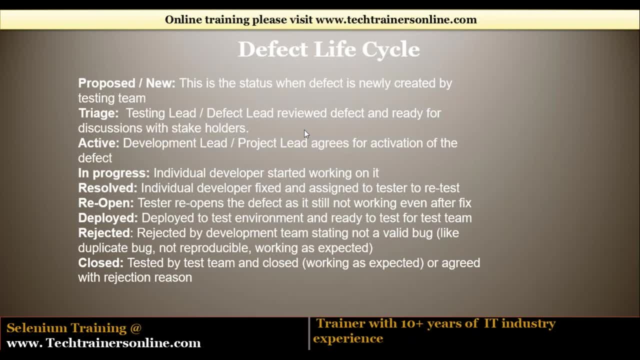 If a client says it's a defect, we have to fix it, Then active. So first it starts with new, then it goes to triage and then it goes to active If the development team is agreed it has a valid defect. So once the defect is agreed, the status of the defect would be changed to active. 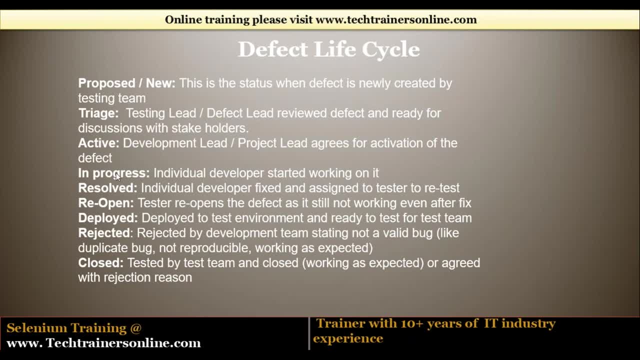 Then it will change. Then the defect status would be changed to in progress when the developer is working. Maybe I have 100 defects raised, but development team will not be working all 100 defects at a time, right, So they keep changing the defect to in progress, whichever the defects they are working in. 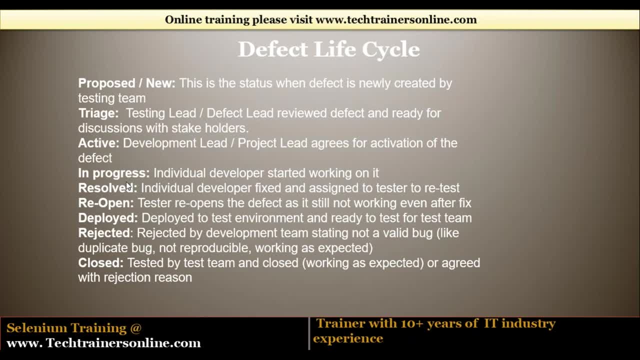 If you see any defect status is in progress, it means that the team is working on fixing it. The next one is resolved. Once the development team fixes the defect, they can resolve it, change the status to resolved And give it to the testing team to test it. 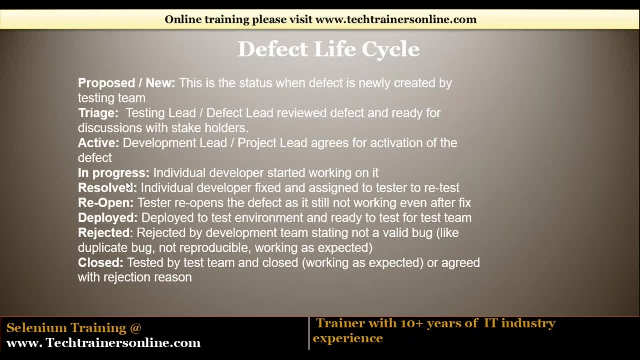 Give it to the testing team to test it, And tester is going to test it. So forget about re-open or deploy. Forget about deploy we will talk about You can ignore it completely. So when I say resolved, it is fixed by the developer and ready to test. 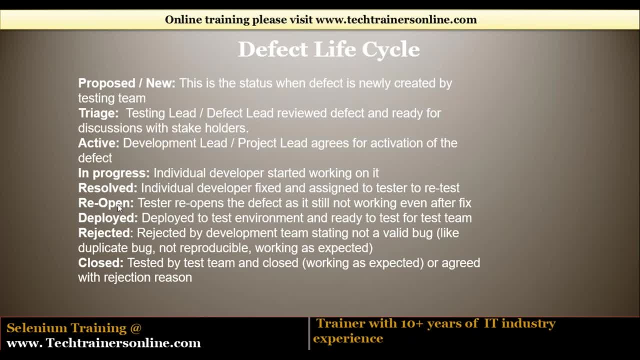 Now re-open. What do you mean by re-open? Now, I am a developer, I fix the defect and I assign it to the tester. I assign it to the tester And once the tester is testing the defect right, Once the tester is testing the defect, they still find the same problem. 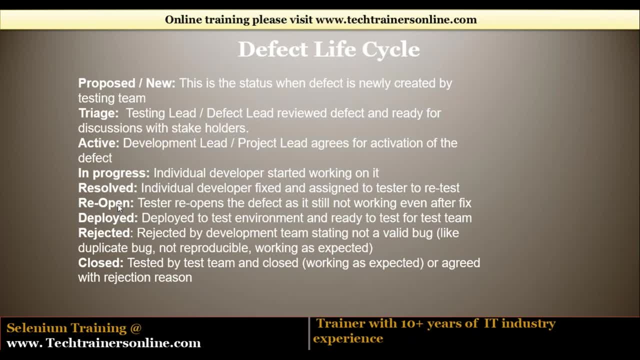 You can go ahead and re-open the defect. What is the status of the defect? Resolved? From resolved, it can be changed to re-open or it can be changed to closed. As a tester, once it is being fixed, I re-test the defect. 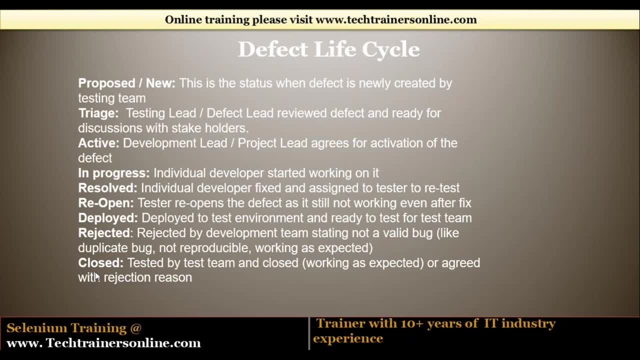 Once I re-test the defect, if I see it is working fine, then I change the status to closed. If it is closed, I will mark the defect as closed. If it is still having the same problem even after the fix, I go ahead and re-open the defect. 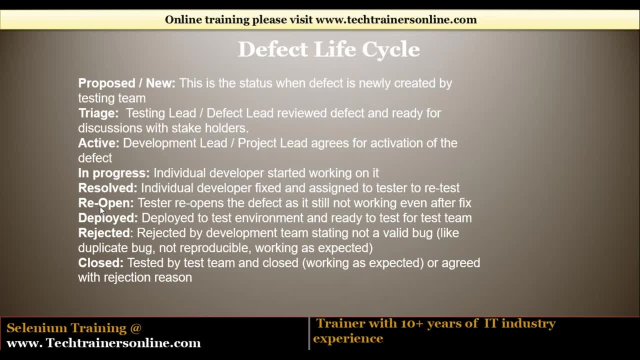 If multiple defects are getting re-opened by the testing team, it is not a good indication to the development team. They are not properly fixing the defect Or they are not even testing the defect once they have fixed the defect. That is called a problem with the development team. 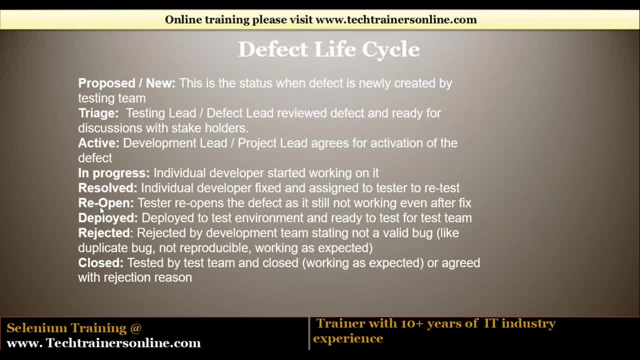 Why they are not fixing it properly, Why so many defects are getting re-opened by the testing team. Now you also have one more status called rejected. So what do you mean by rejected? Now tester raises the defect I just gave an example of. let's say I was saying that Dhan Sri is raised a defect where she is not able to log in with user ID and password. 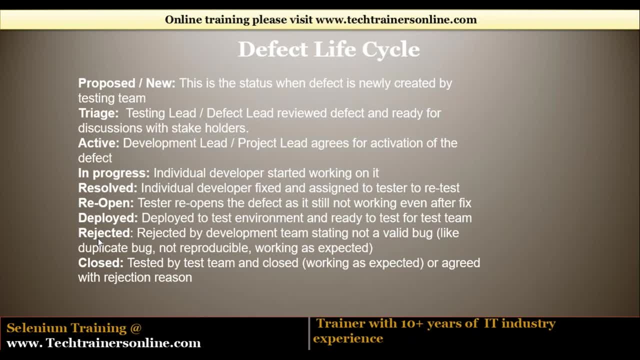 We discussed that there is a problem with the test data. Do you think it is a defect? Because others are able to log in, but only for her credentials. it is not allowing to log in Because account is locked. straight away developer will investigate it and straight away can reject the defect with the valid rejection reason. 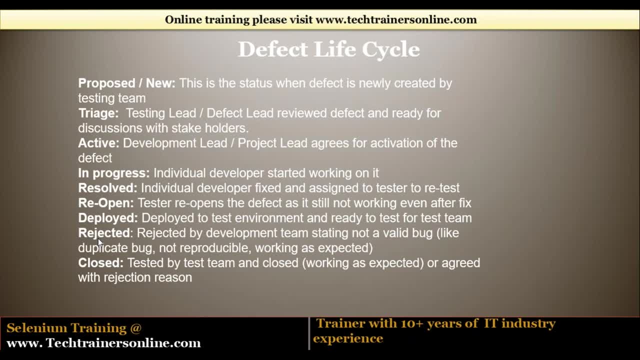 Saying that it is a problem with the user credentials that are used. It is locked. I unlock the user now in the backend. try to log in and re-test and close it. It can be rejected. Developer can even also reject the defect. 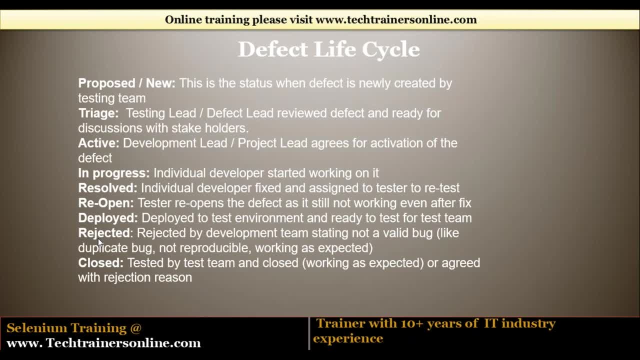 It does not mean that he or she should accept every defect that you are raising it. So that is where the defect is going to be rejected, Rejected by the development team stating not a valid bug, due to it can be a duplicate also. 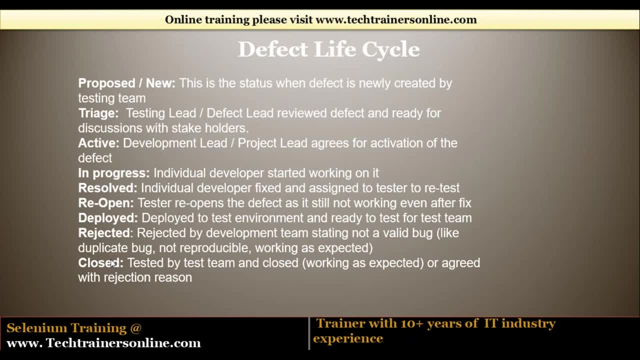 Like Ankit and Dhan Sri, both raised the same defect with the different IDs right, So I can keep one defect active and another defect. I can mark it as a duplicate and reject the defect right And it may not be reproducible. 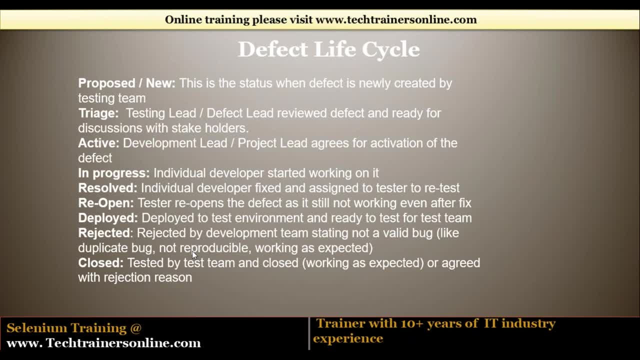 Now I set an example user ID and password where she raised a defect. It is not allowing to log in. It is not reproducible for other users, So I can. It has been rejected or working as expected. So when the developer is rejecting your defect, either it can go to close status. 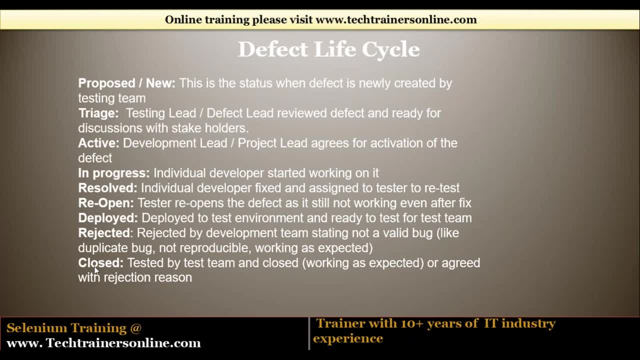 Now I am a tester. I raised the defect. There is a duplicate defect which is already raised by Ankit- Sorry- someone else in the testing team, And then they can go ahead and reject the defect, saying that it is a duplication of defect, and assign the defect back to me. 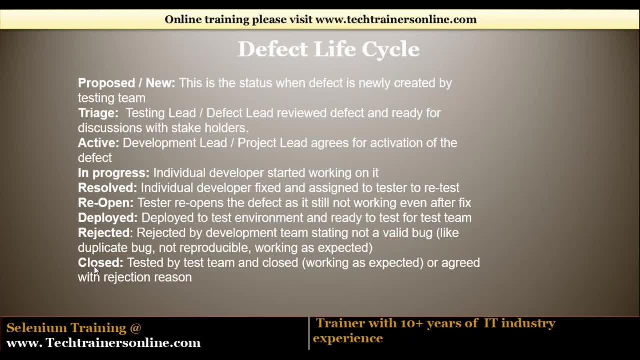 What I can do. I can see the rejection, I can see the rejection reason and I can straight away go ahead and close the defect with a rejection reason. It doesn't mean that the developer is giving a rejection reason. tester has to listen. 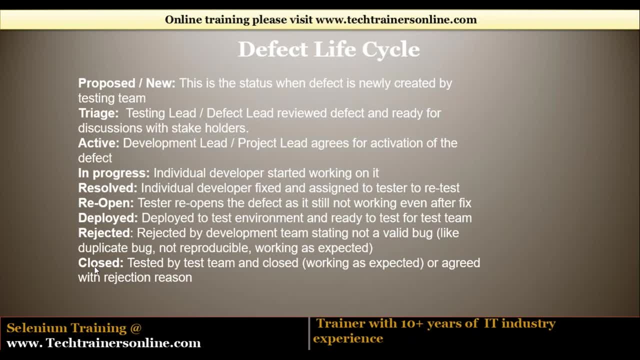 No, If you are not conveyed with the rejection reason, again, change the defect to triage so that you can go ahead and discuss with the developer. So these are the different defect lifecycle, generally what we call it as Any questions so far. 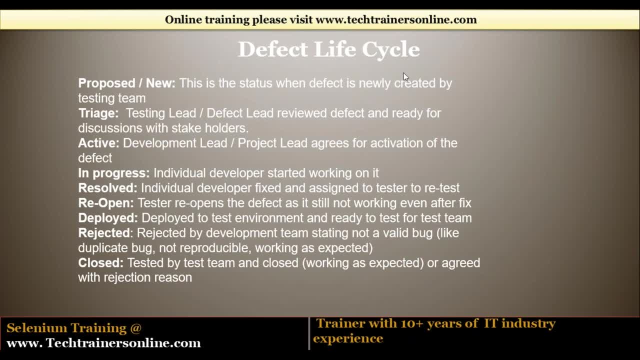 For this lifecycle. there is a tool, because if we do manually it's very time-consuming process. You cannot change the status of the defect. it will not change on its own. you have to change it. So let's say you raised a defect by default, if the status would be new, you don't have to select any status first time when you are raising it.